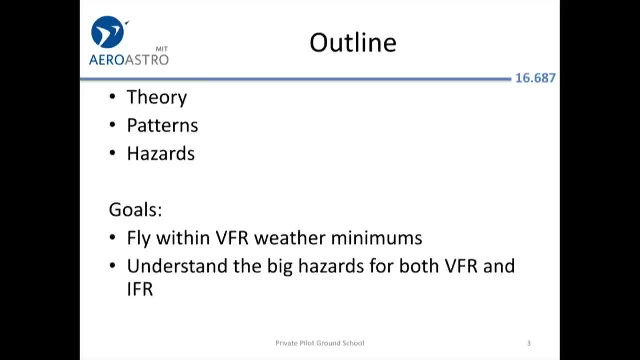 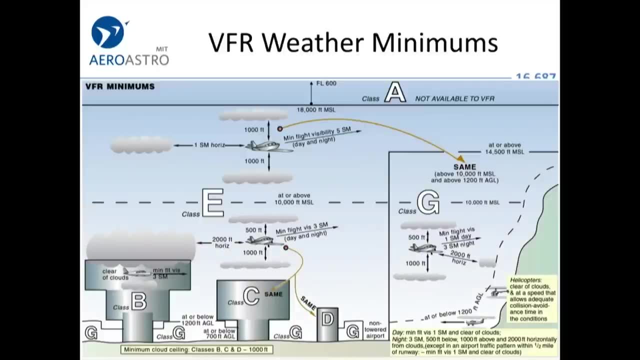 weather minimums and predict when those minimums aren't likely to be met or when there's going to be really serious hazards such as thunderstorms. All right, this will be on the test. You have to memorize all of this. Well, you kind of do. Anyway, they want you, you will you. 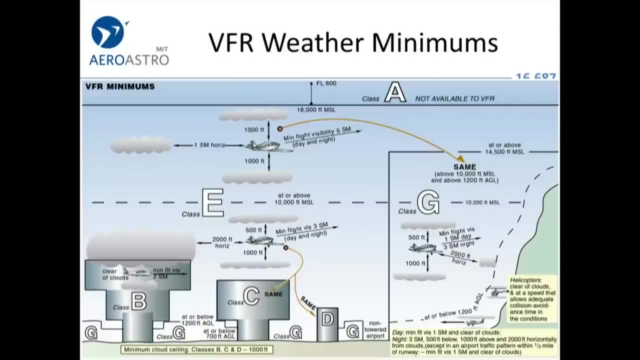 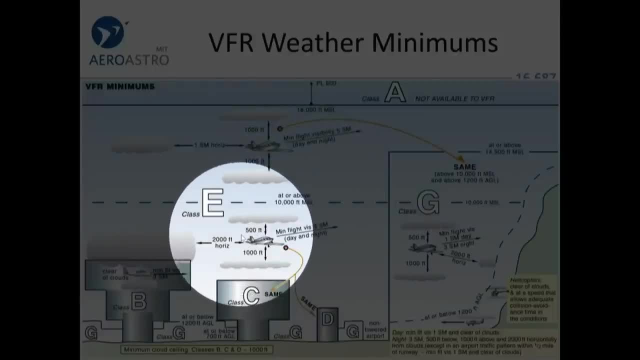 have to learn some of the stuff for the exam. In reality around here almost all airspace is at least class echo, That's controlled airspace. It means controllers could give you a clearance to fly on instruments and separate you from other aircraft, So they want you to be well separated. 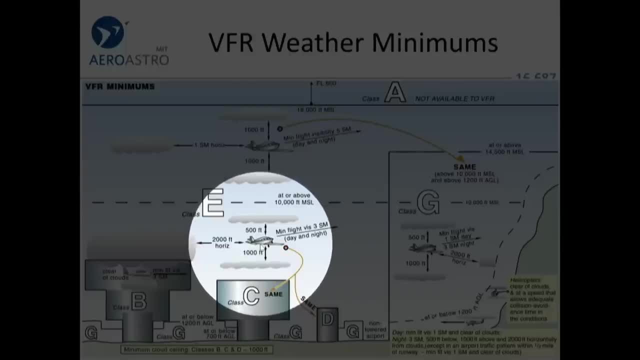 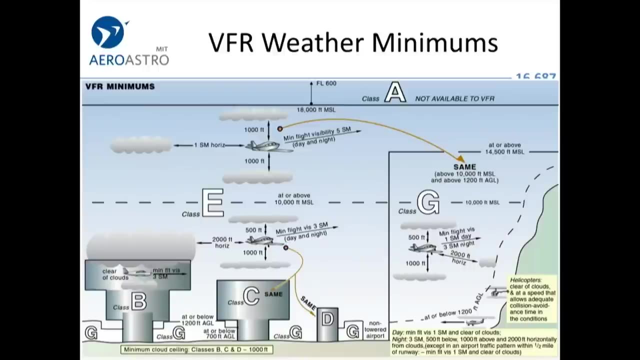 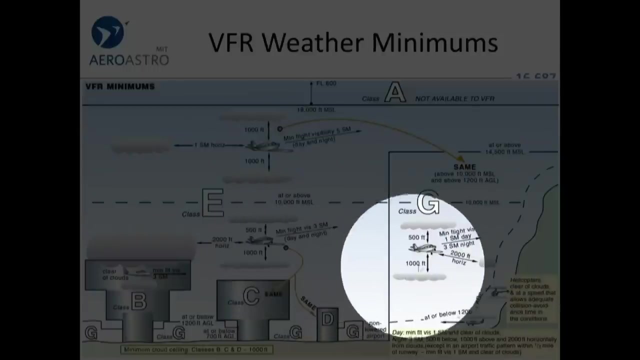 from clouds 1,000 feet above, 500 feet underneath, 2,000 horizontally. That way, if an aircraft IFR- comes out of the clouds, there'll be some time for the two of you to see and avoid each other. You can see the weather minimums are different in class golf airspace And actually. 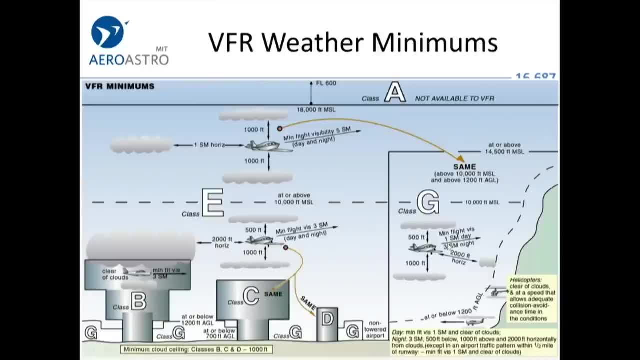 in uncontrolled airspace, like up in Alaska, if you're flying on instruments, you don't have a clearance. So you say, well, how is that possible? You can be instrument rated, have an instrument capable airplane and fly from airport to airport in the clouds, But the air traffic controllers 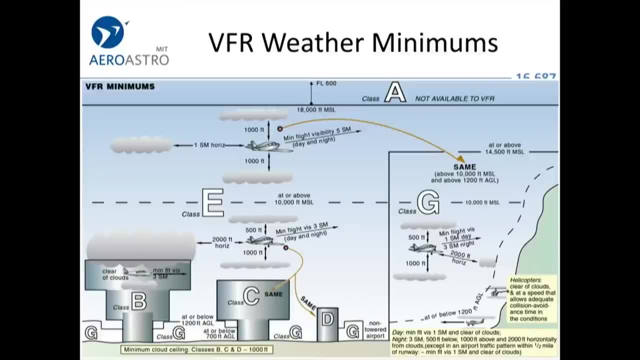 they can't give you a clearance and guarantee you separation from other aircraft because they don't have radar. They don't even have the authority. It's not controlled airspace. I've done some flying up there in little airplanes and you have to be very patient. Another interesting 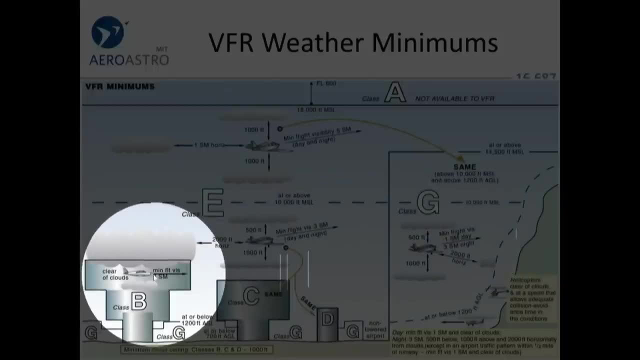 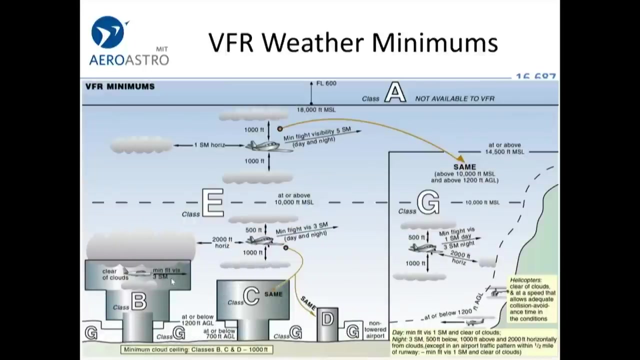 thing to notice about this- we'll talk about it more again later- is notice how class Bravo airspace has lower minimums than ordinary class echo airspace. So we have to be 1,000 feet from the clouds here. Here we just have to be clear of the clouds. Why are the minimums reduced, right? 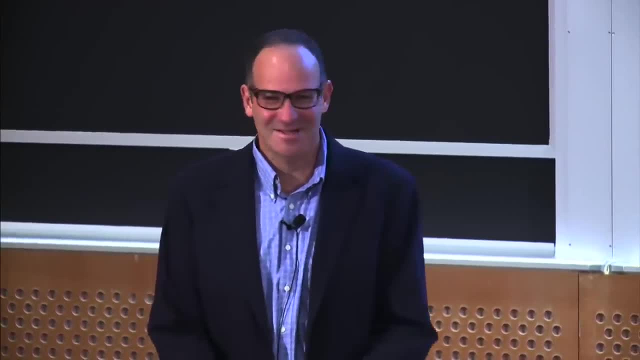 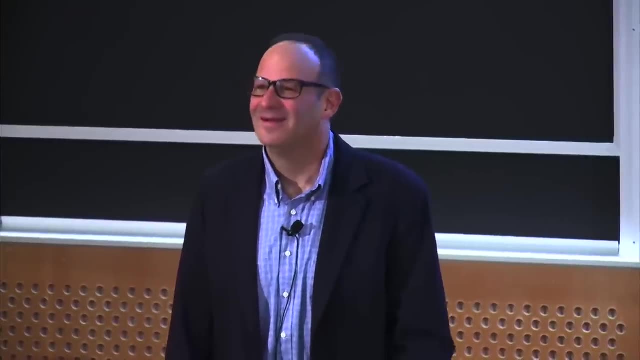 around Logan Airport and JFK and LAX, And they are Because everyone's in contact with the tower, so the tower's telling knows where everyone is. Yeah, great answer. So her answer is that air traffic control is in contact with everybody. 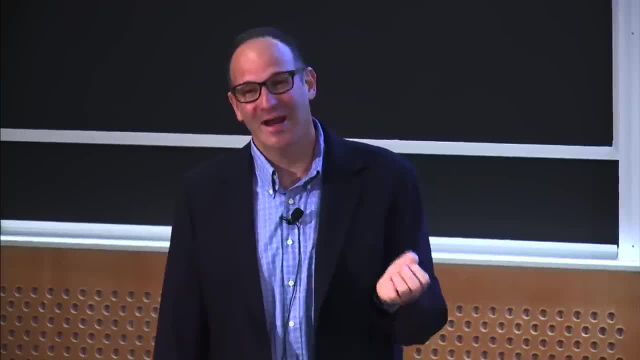 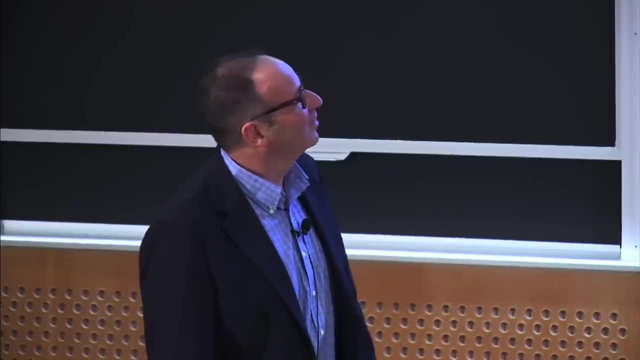 in class Bravo airspace and knows where they are, And in fact their own clearance is in class Bravo airspace. So they're being told what to do: fly this heading, fly that heading, maintain this altitude. Great answer, All right. So how do we know if the weather minimums are going to be? 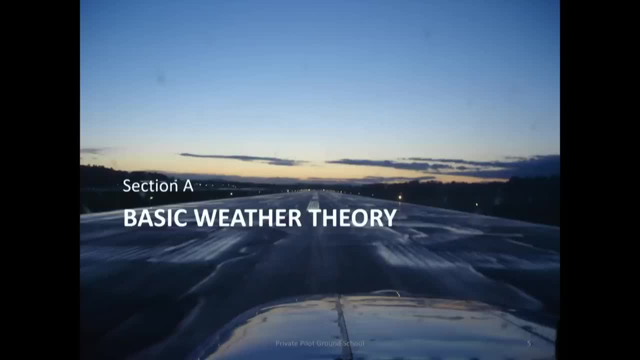 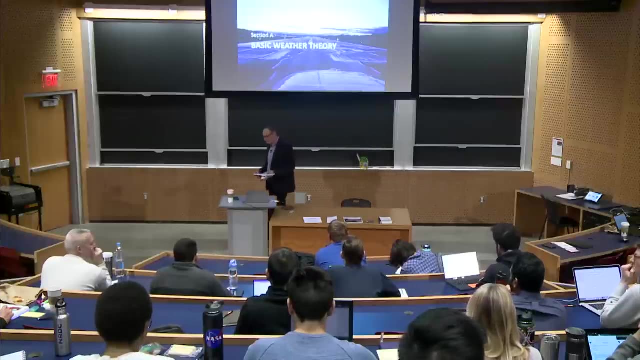 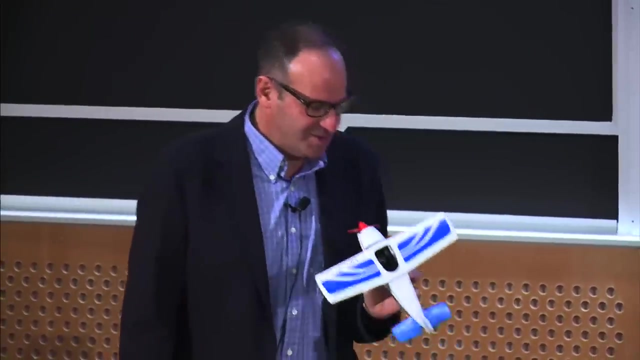 maintained. Let's talk about weather theory. So raise your hand if you're a science major here, as opposed to engineering, Where are the smart scientists? All right, Francis, Francis. So the science approach to this task would be to say: 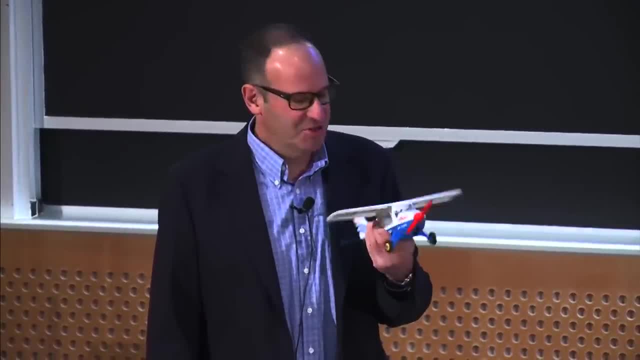 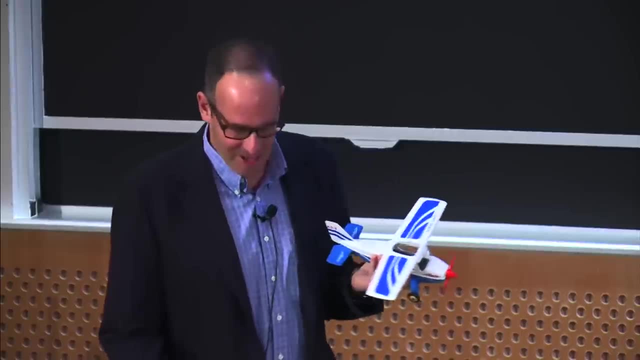 you know, if we're going to be able to maintain the altitude, we're going to have to maintain the altitude, And if we could just assume that humans are only four inches tall, then we could build some really great aircraft, And we'll get into that in a moment. Just think about that. If you're 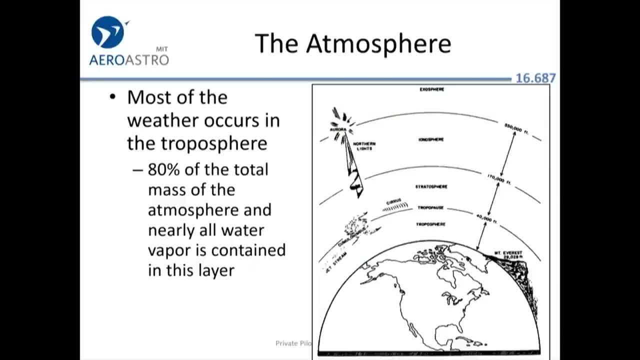 a scientist, how much flexibility can you have compared to being an engineer? All right, So let's look at the atmosphere that we do have. Mostly, the troposphere tops out around 40,000 feet, according to this chart, And that's where most of the water vapor is, and therefore, 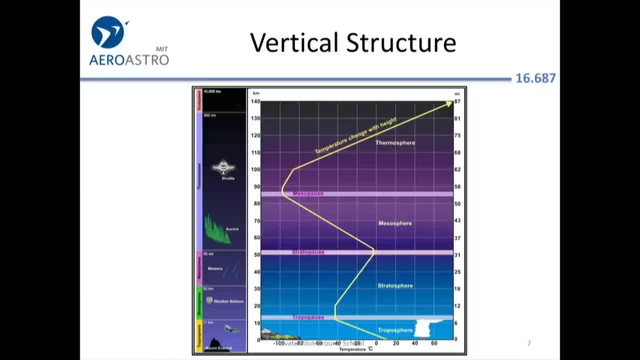 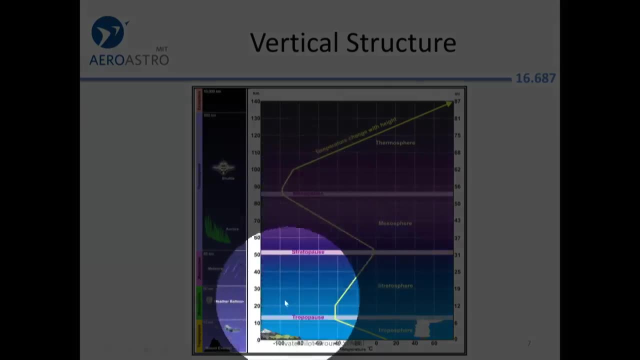 most of the weather, Also the higher temperatures You can see. it actually does get warm again way up high in the thermosphere. This is in kilometers on the left, So you can see the part of the Earth that we're flying through is really just, I don't know, probably around. 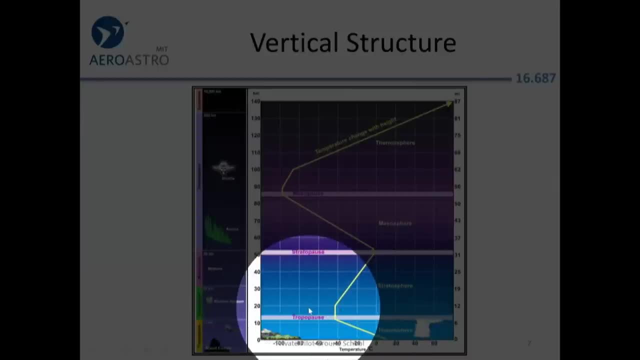 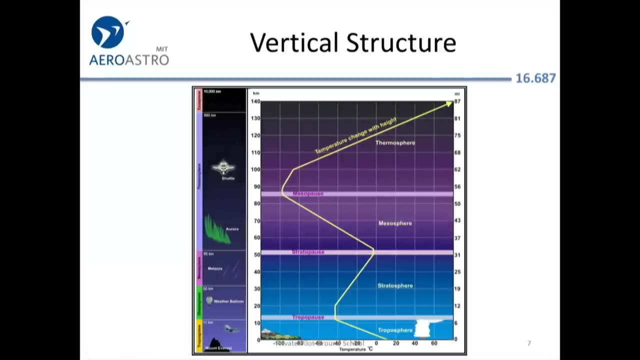 say 20 kilometers and down. What did Laz say? He said he could go up to 65,000 feet in this F-22. So that's what about? that's a little over 10 miles, So like 20, yeah, it's about 20 kilometers. 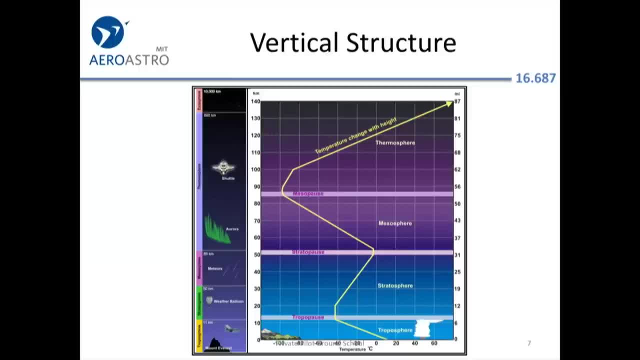 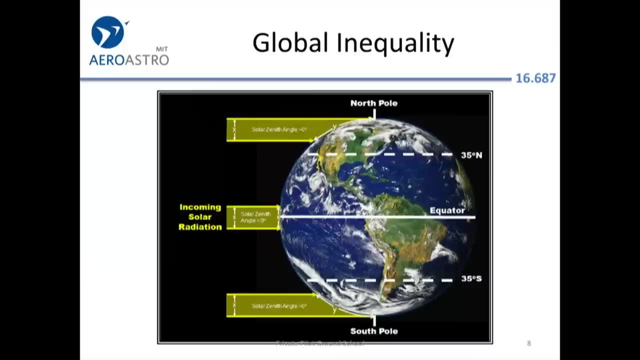 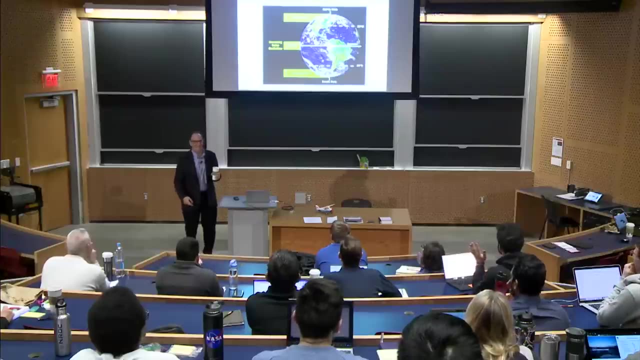 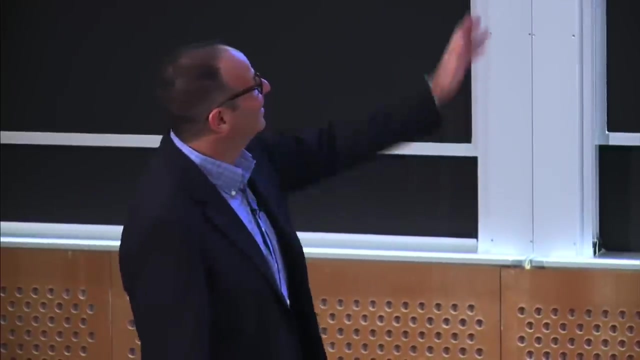 somewhere in that neighborhood, Anyway. so not too many people are going higher than just the bottom zero through 20 on this chart. All right, Who's concerned about global inequality? Raise your hand. Awesome, Well, you'll be pleased to know that. so is the FAA And this figure here. 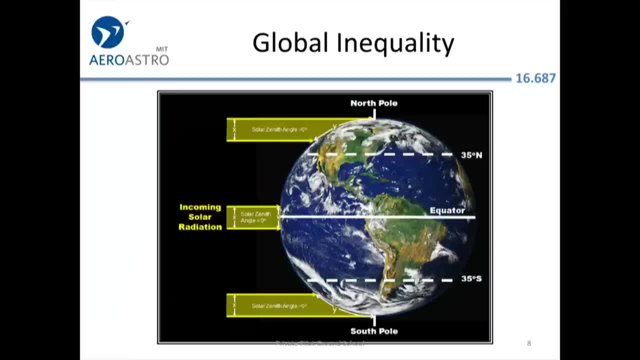 shows you why it's warmer at the equator than up at the North Pole. There's the same amount. we're missing a little bit of tilt here, but that's OK. There's the same amount of incoming solar radiation, but it gets spread out over the师. 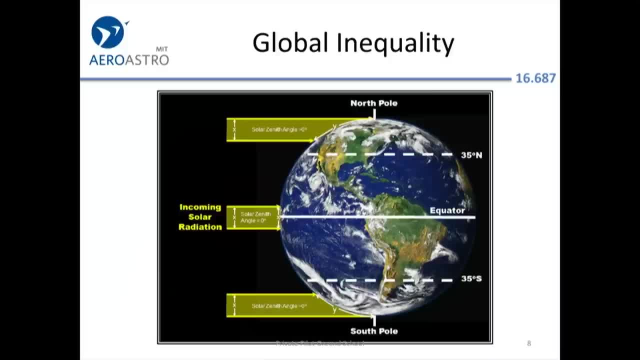 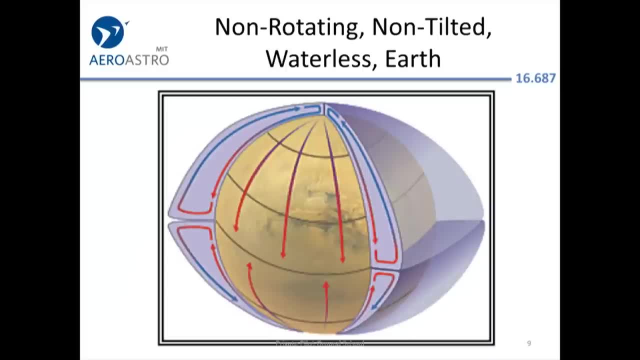 There's the same amount of incoming solar radiation, but it gets spread out over the 스, over a larger portion of the Earth up near the poles, All right, so this is where guys like Francis have it easy. If you want to understand something, you just say: well. 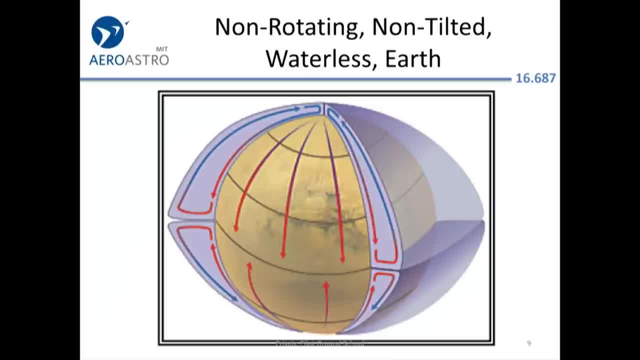 I've got an Earth and it's pretty much the same as the existing Earth. It just doesn't have any water on it and it doesn't rotate and it's not tilted with respect to the sun. So now I'll do my analysis and I'll publish my paper. 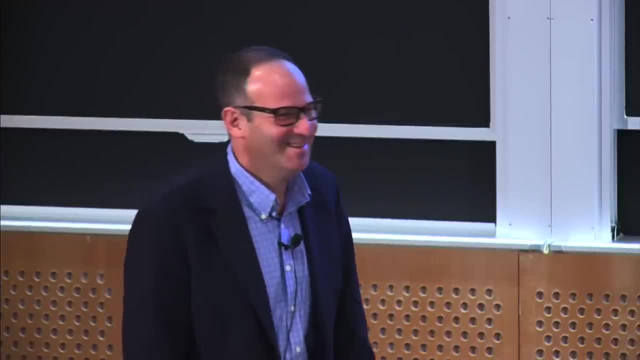 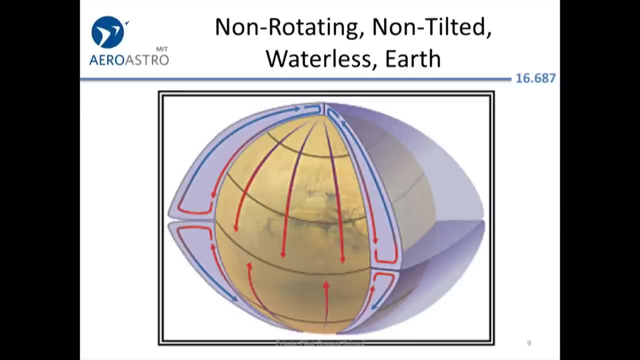 and I'll get tenure and your problem is solved. So let's say: let's see what would happen here In a non-rotating, non-tilted, waterless Earth. it would get hotter at the equator and the air would rise up from the heat. 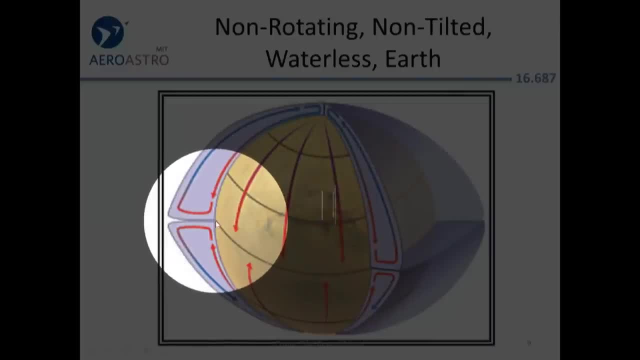 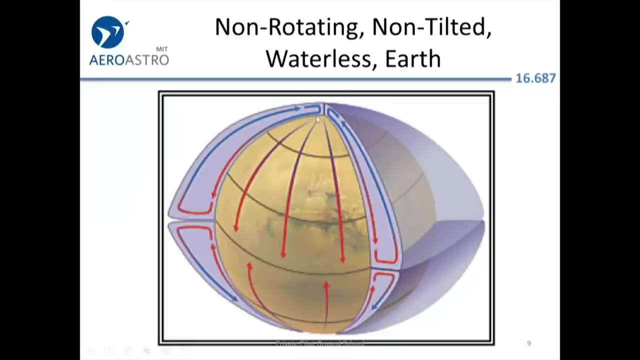 So we can see that here. So we would have low pressure right there at the equator and then the air would circulate up and we would have high pressure up the equator, So we would have low pressure up the poles. Does that make sense to everybody? 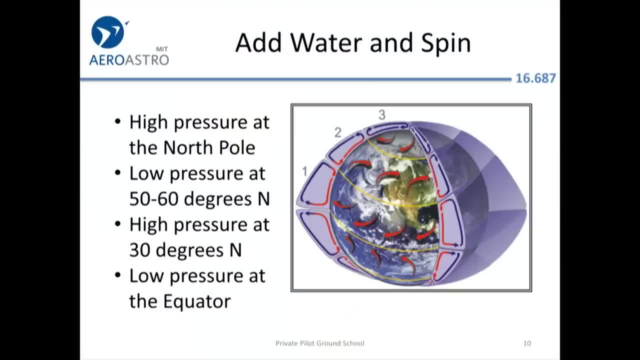 All right, great Problem solved, We can go home. Unfortunately, as engineers, we have to deal with the real world a little bit more. So if we're spinning around the Earth, we're going to end up with these three cells in each hemisphere. And in this case you end up still with low pressure at the equator, but then you get a high pressure with all the air sinking down here and you get still low pressure. You still get high pressure up at the poles and low pressure down here. 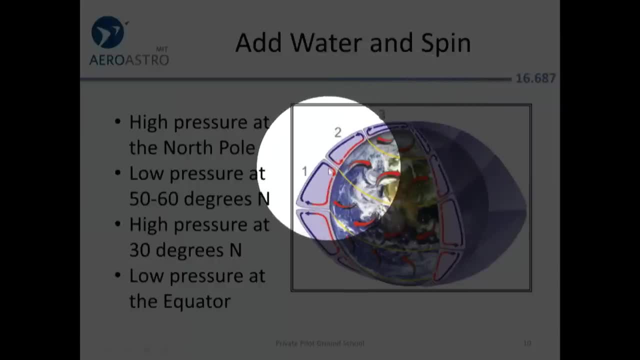 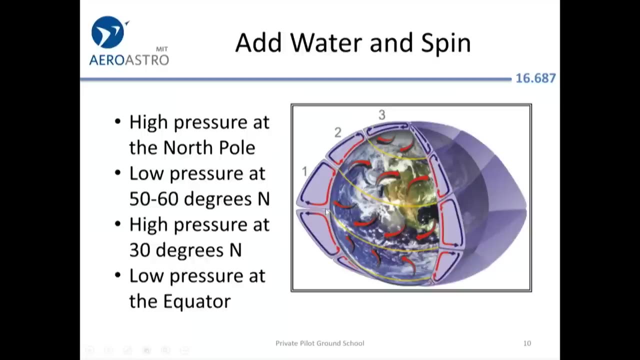 Let's see if I got that right. High, that should be high. It says high pressure at 30 degrees north. Oh yeah, high, high, that's good. And the s and low and low. All right, we got that right. 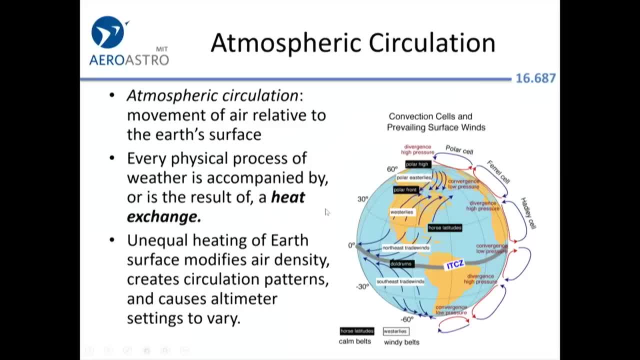 It gets more confusing, as you see. OK, so the circulation. one thing that the FAA wants you to know is that it's heat exchange that drives the weather. So the weather is basically a function of the sun heating up the Earth, and then it's not uniform. 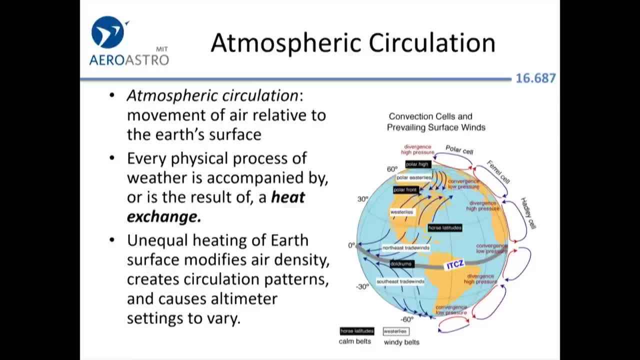 so the heat gets pushed from one part of the Earth to another, And all of this unequal heating is responsible for the altimeter varying, for wind blowing around. Pretty much every phenomenon that is of interest to pilots is caused by heat trying to move from the hotter parts. 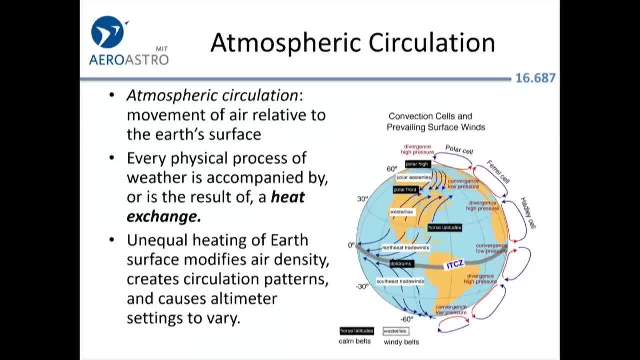 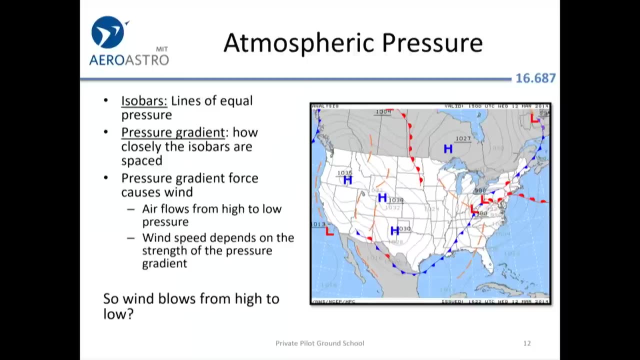 of the Earth to the colder parts of the Earth. We'll talk a little bit more about these, but notice, there's parts of the Earth that are windier than others. Unfortunately, we're in one of the windier parts. OK, so you also have to know, as a pilot, just what an isobar is. 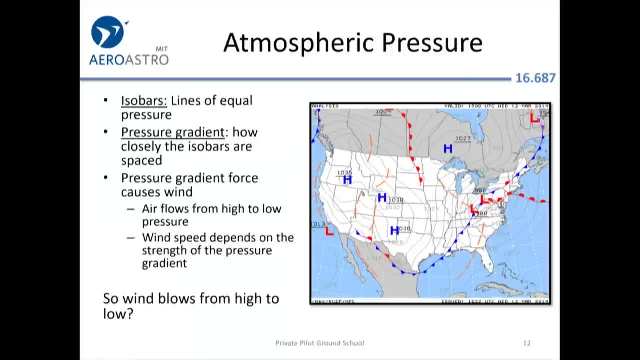 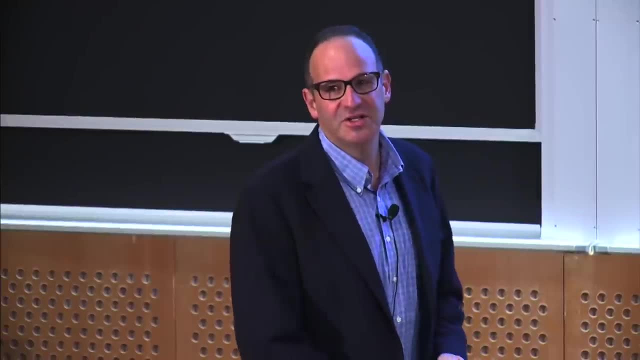 That's the line of equal pressure And that tells you, that gives you an idea of how the wind is going to move. We'll see that in a minute. The tighter the isobars, the more dramatic the pressure change in a region. 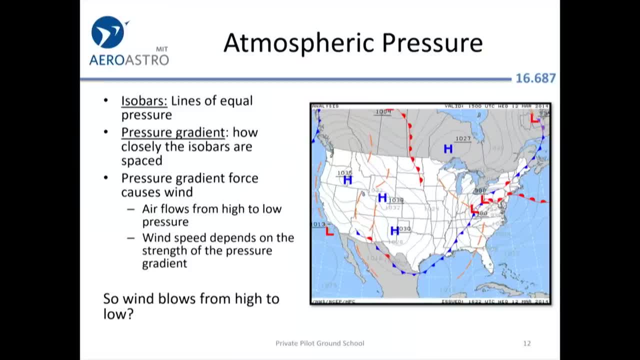 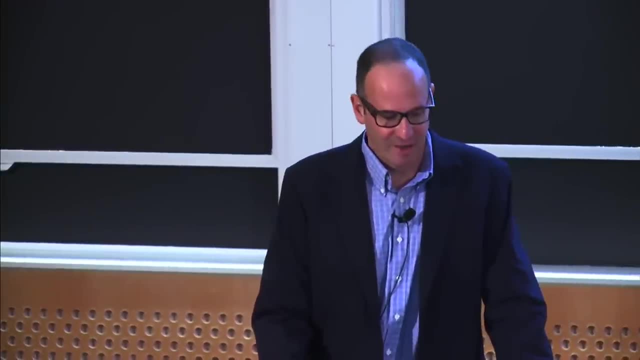 And it's the pressure gradient force that's causing the wind to flow from the high to the low pressure. So you might think, on this chart, for example, that wind wherever you see an L and an H- that you would just draw a vector of wind from one place. 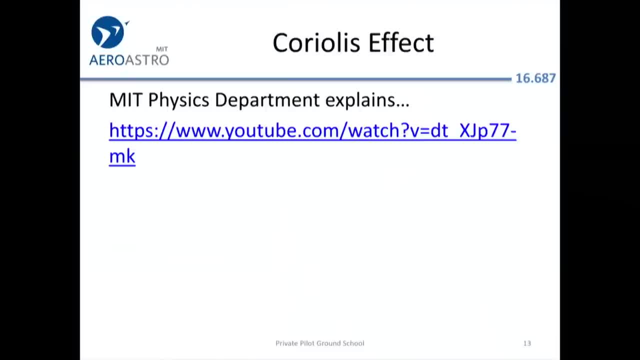 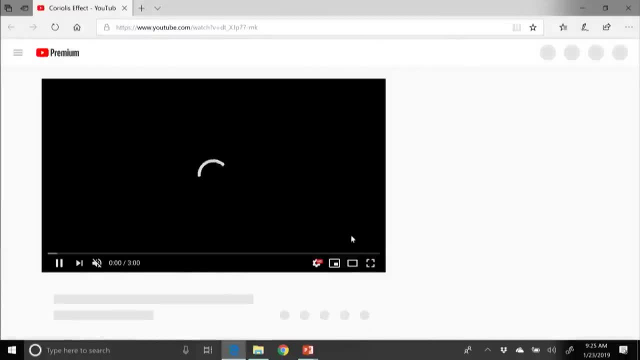 to the other right. That kind of makes sense. However, there is Coriolis force. This is for Francis the science major. Francis, what course are you? I'm course 9, so nothing good business or anything. 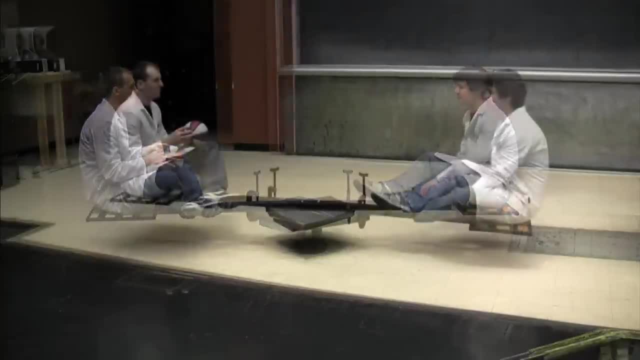 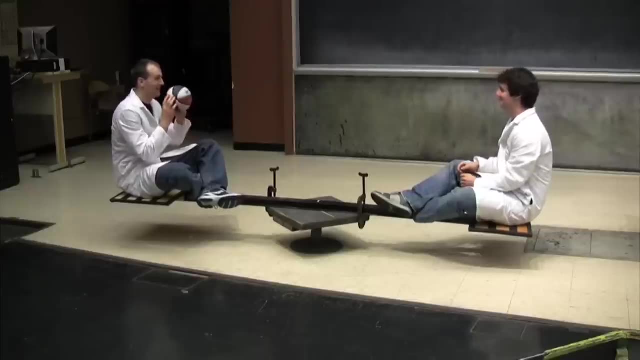 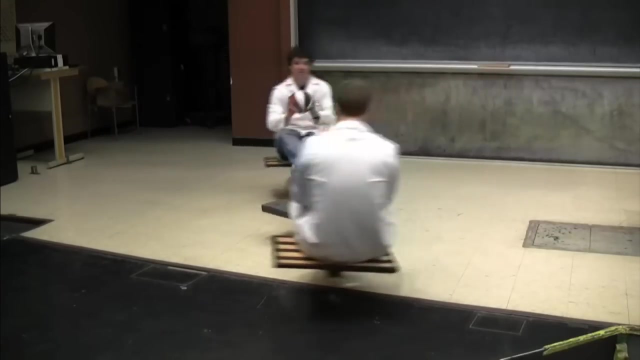 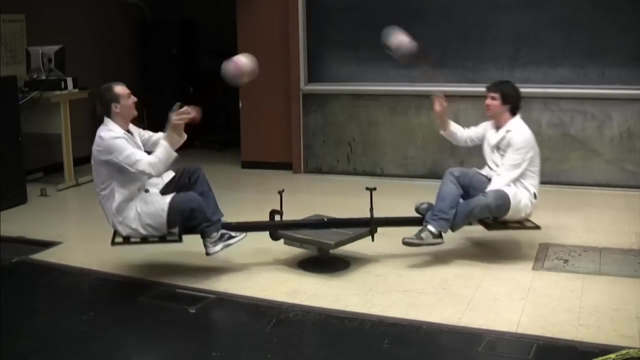 No, All right, so scientists wear lab coats. Coriolis force is a fake news force formerly known as fictitious. So you can see they're throwing the ball straight, but because they're on a rotating platform, it's apparently curving. 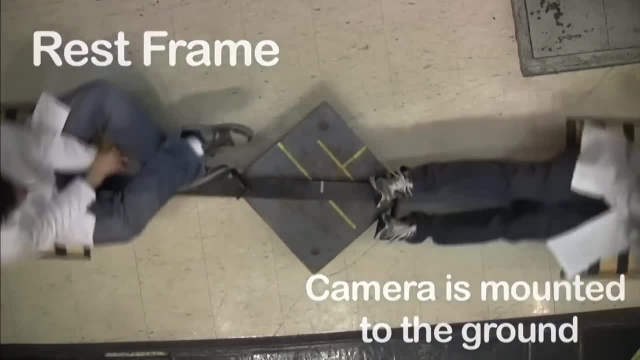 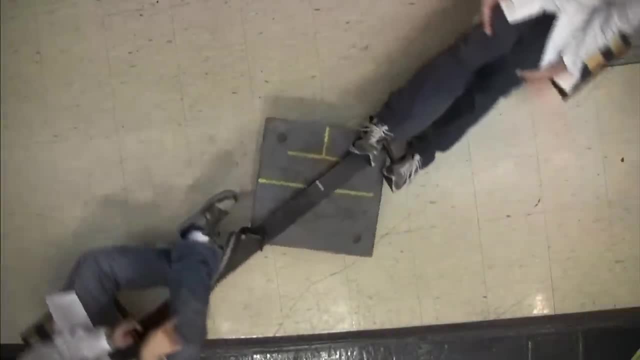 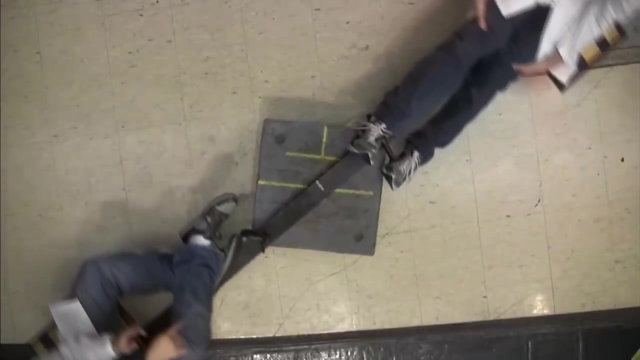 So camera is mounted to the ground and we'll see the ball going straight. They're going to draw you a little dash line at one point So you can see the path is actually straight. So the ball has inertia, Basically, once it's launched it. 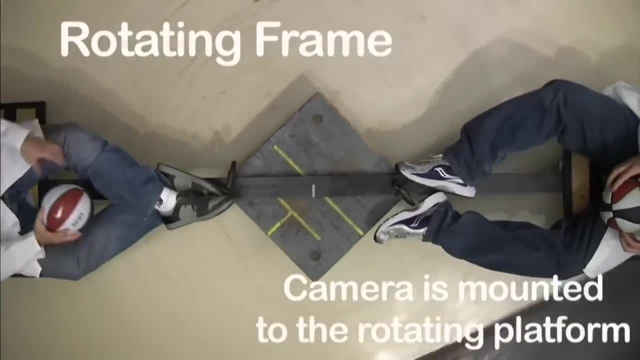 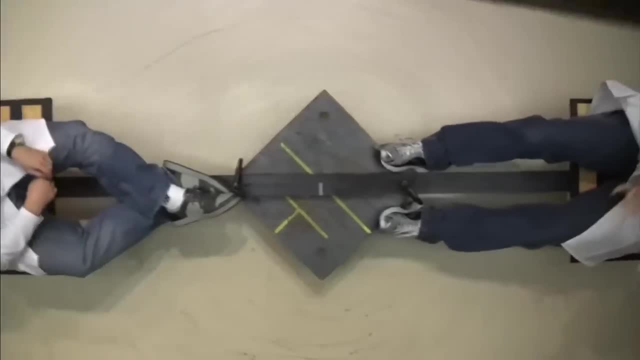 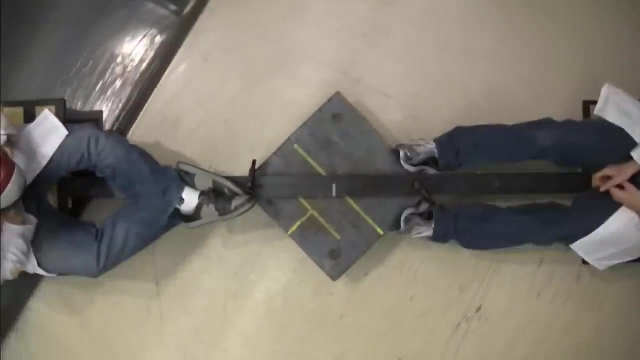 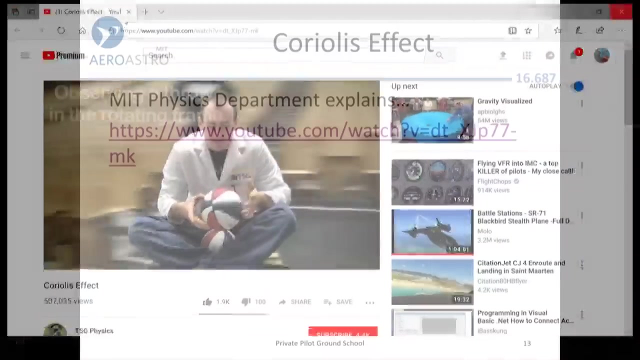 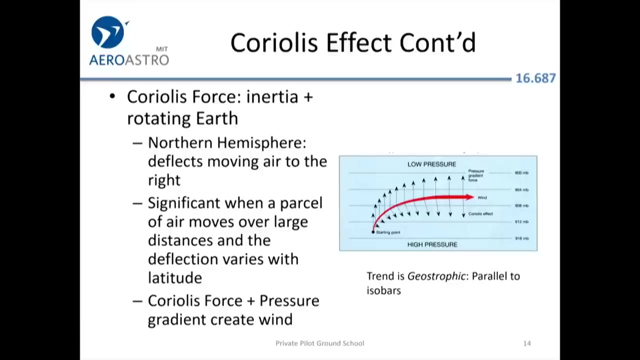 wants to keep doing whatever it was doing And this guy's white lab-coated colleague colleague just moves away from where the ball was going. All right, everybody's got that. That's Coriolis force for you, All right. what happens when we do this on the Earth? So think about it. You have a parcel of air that's moving with the Earth at the equator. If you displace it up to a higher latitude, it still has that velocity, But now the Earth isn't spinning as fast, so it ends up essentially moving a little bit to the right. 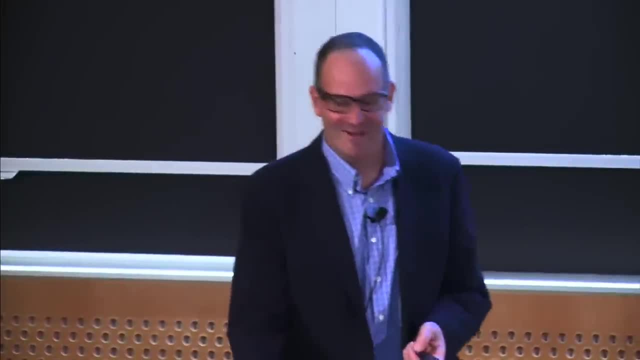 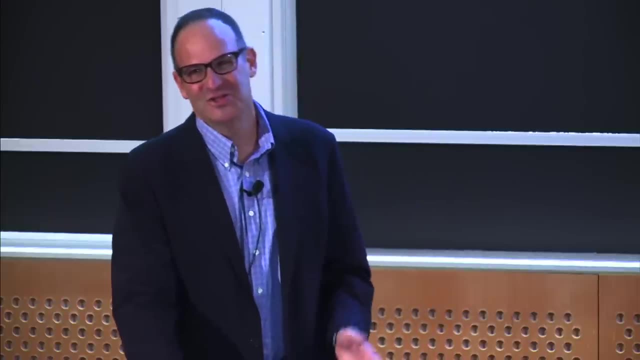 That is the fundamental insight, just as you said. As you saw in that video, You'll have to go home and think about that a little bit, But basically I think the most effective way to think about it is just that: the parcel of air. that was at the equator wants to keep moving as if it were still at the equator, but it's not there anymore. So it moves relative to the underlying Earth. If you combine the Coriolis force and the pressure gradient then you get the actual wind direction. 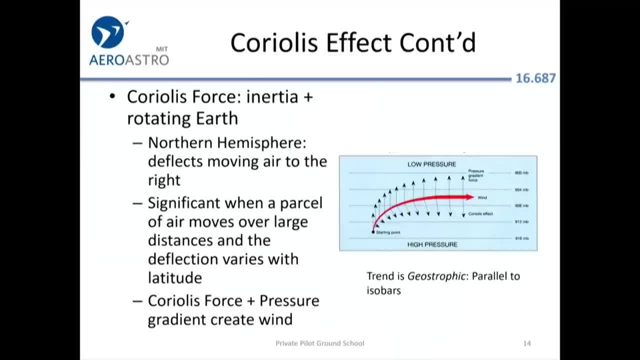 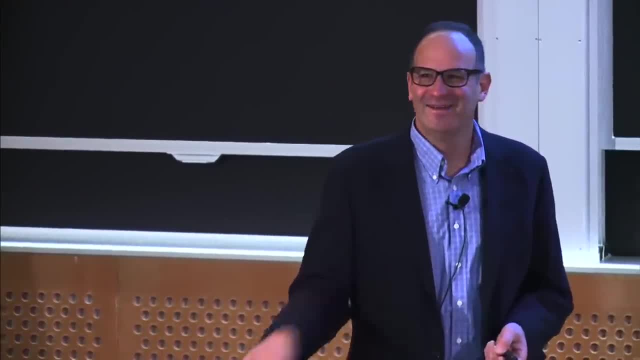 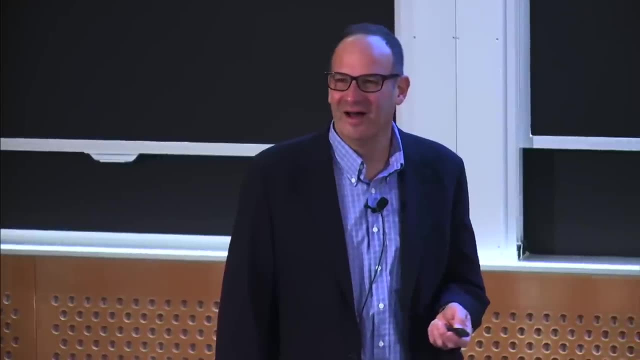 And the trend. And, as seen here, eventually there's so much Coriolis force over so much time that the wind actually moves exactly 90 degrees to where you think it should move. It flows along the isobars instead of perpendicular across them. 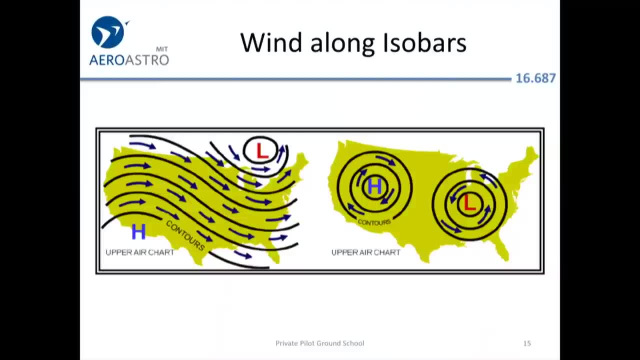 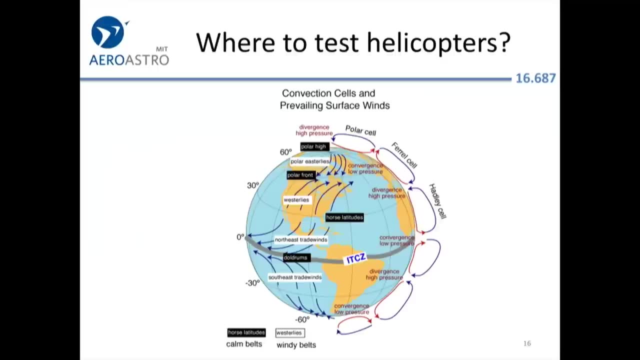 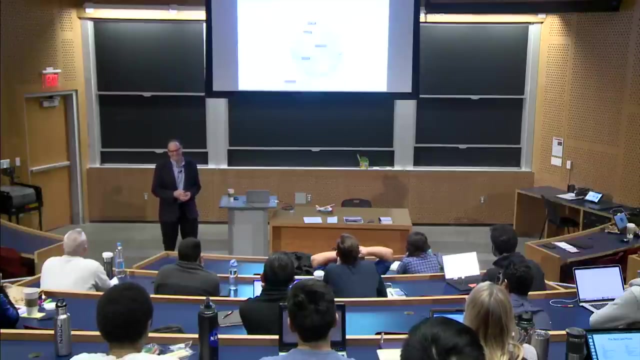 So there you have a couple pressure systems And you see that the wind is circulating around these lows and highs rather than, you know, flowing directly from one to the other, as you'd expect. All right, Who would like to become a helicopter test pilot? 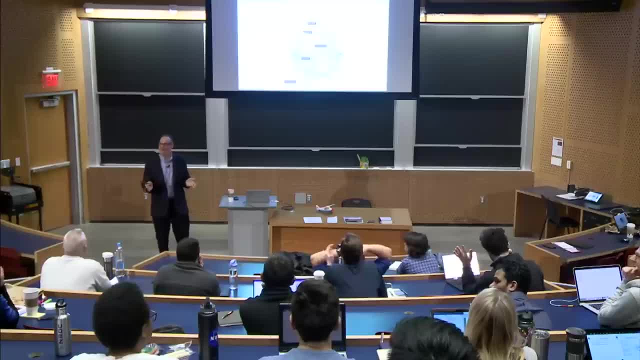 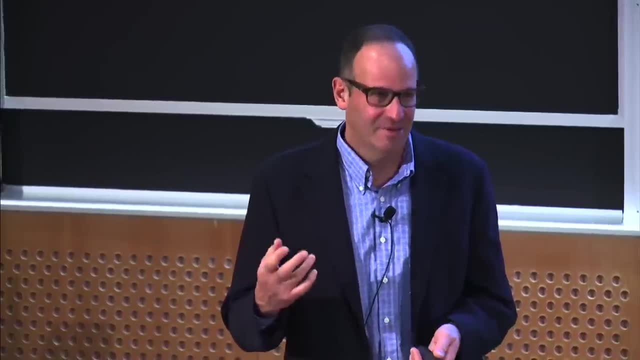 Raise your hand if that sounds like a fun job, OK. So when you're developing the manual for your Sikorsky helicopter, you've got to go somewhere where the wind is calm. Where would you all suggest going now that you've seen this chart? 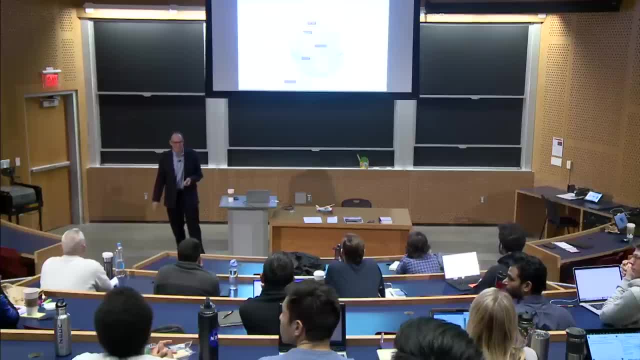 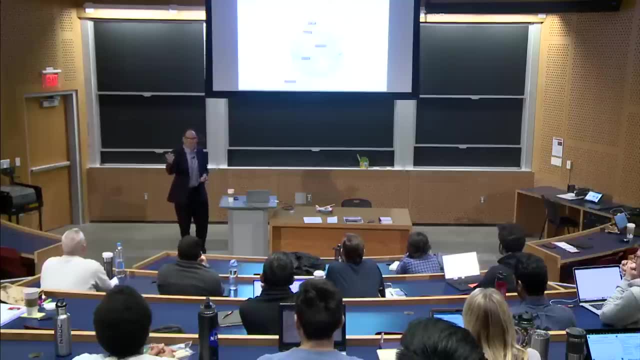 Who wants? What's your name, sir, Sorry, Oh, Jeremy. Jeremy, where do you want to go? You're going to take your Sikorsky helicopter and you're going to write the POH Florida, Florida, Sikorsky, which is headquartered in Connecticut. 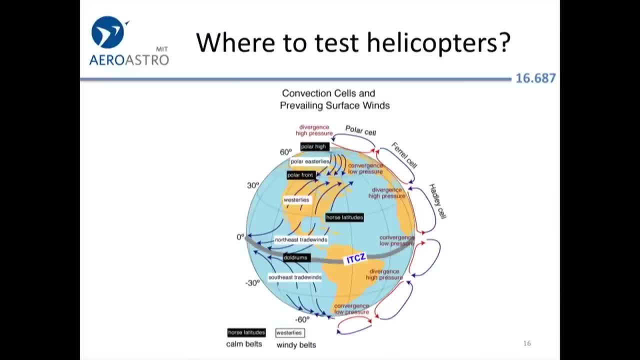 they have a big flight test facility. I believe it's in Palm Beach. So there you have it. They thought just along the same lines as you And they'll be in the horse latitudes. There's a whole bunch of there. Nobody really knows why it's called the horse latitudes. 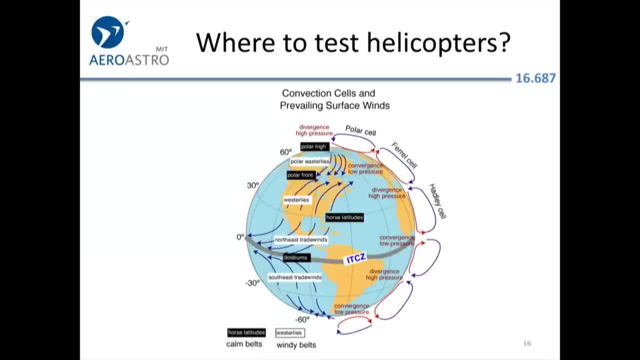 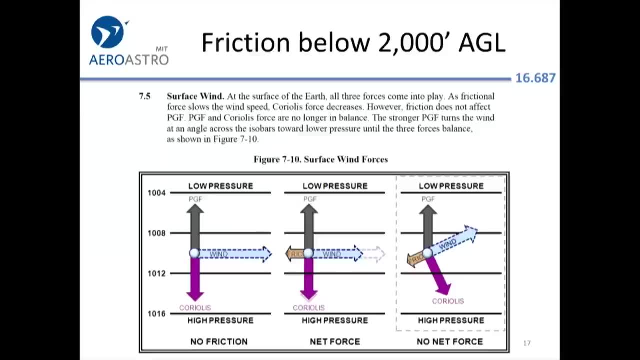 One idea is that the ships, since there's no wind in those latitudes, they have to find a current And then they get pulled along by the current as if they were on a horse. All right, Surface friction is a little bit complicated. 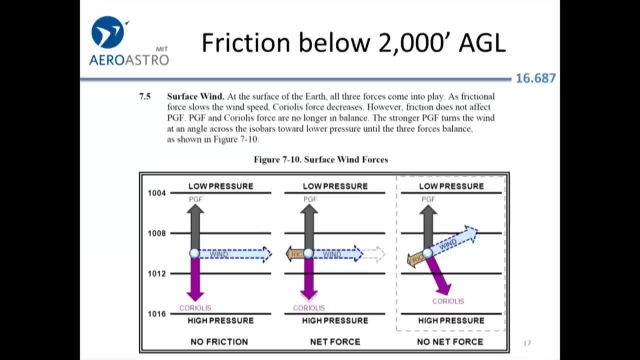 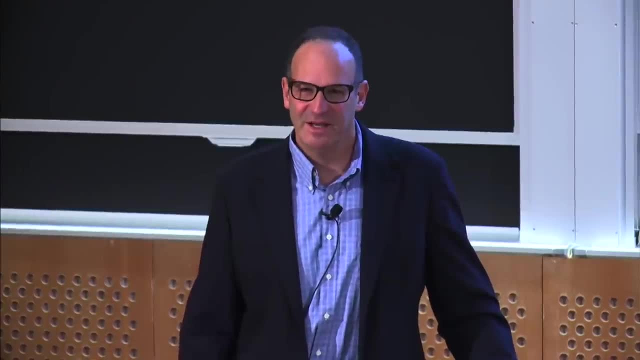 It tends to drag down the wind. You'll have to study this vector diagram on your own, But really, from the FAA's point of view, they just want you to know mostly that, OK, OK, OK. So wind 2,000, 3,000 feet up is going. 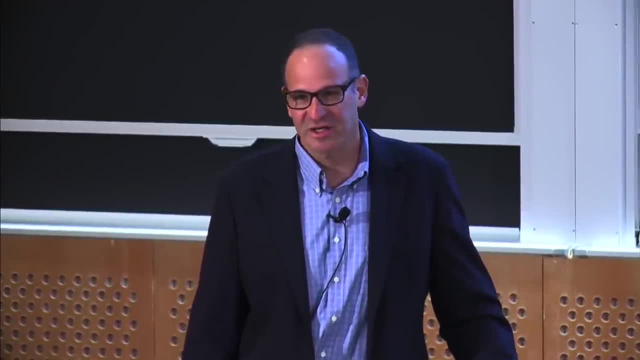 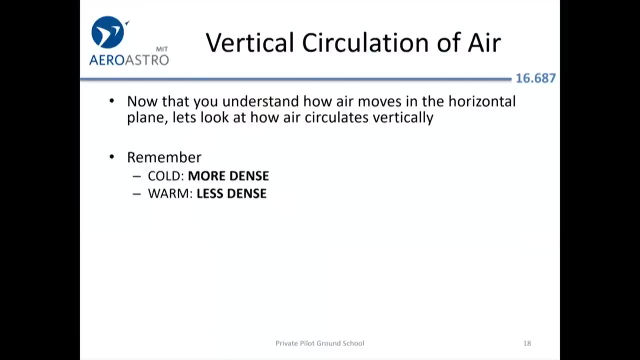 to be different from the wind on the surface because of surface friction. It'll be less intense and in a slightly different direction. OK, Vertical circulation of the air. I think you're going to be OK, if you just remember that warmer air is lighter than colder air. 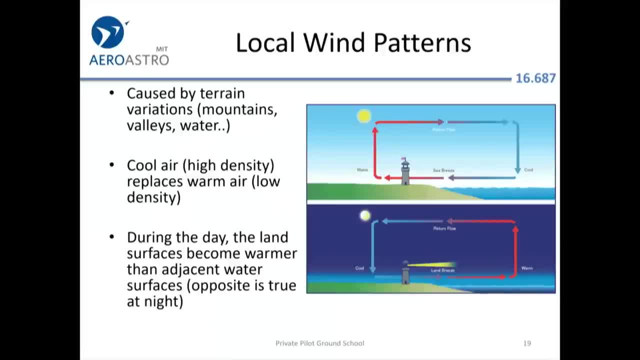 That's all that you pretty much need to know. OK, local wind patterns. So if you heat up the shoreline, the air will rise off the shore and pull in air from the ocean during the daytime, So you get that sea breeze, And then at nighttime the opposite happens. 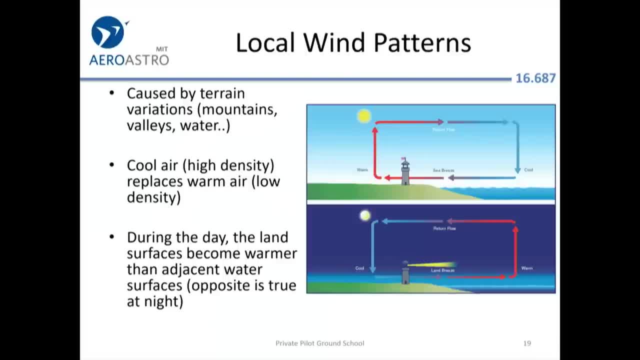 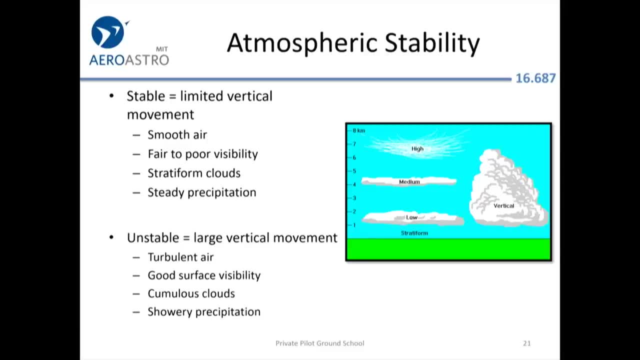 So you get a land breeze. So there are some of these predictable local weather patterns. The bigger ones have to do with atmospheric stability. If you have a Stable atmosphere, meaning that a displaced parcel of air tends to get pushed back down to wherever it was, 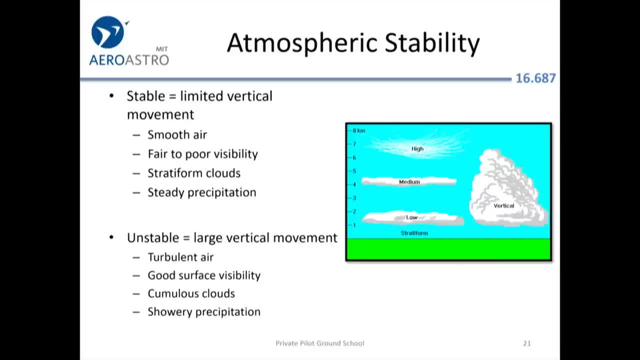 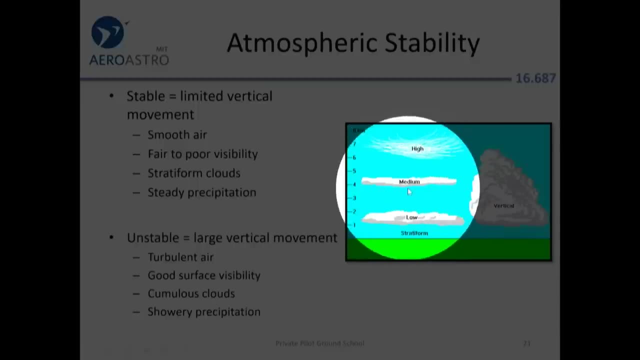 Then you get these weather characteristics, where you're not going to be bumped around in your aircraft, You're going to have trouble seeing And you're going to see clouds that are basically flat, these stratiform clouds here that you see on the right. 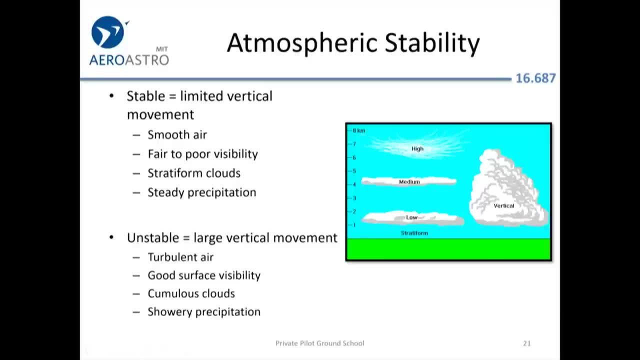 If it rains, it's just going to rain all day. It's going to be a typical miserable New England day where it rains all the time, or Seattle, I guess, is like that as well. Well, what about if the air once displaced? 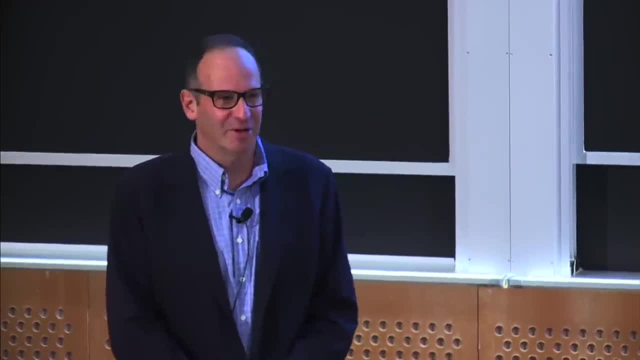 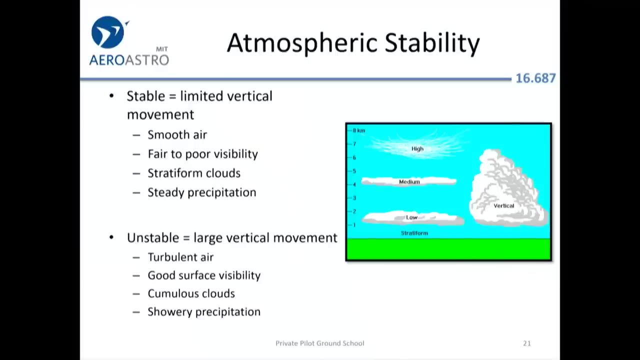 tends to want to keep being displaced. If it rises up a little bit, it keeps rising. Then you have these clouds with vertical development And the good news is you can see really well. You're not going to have an obstruction to visibility unless you're in heavy rain. 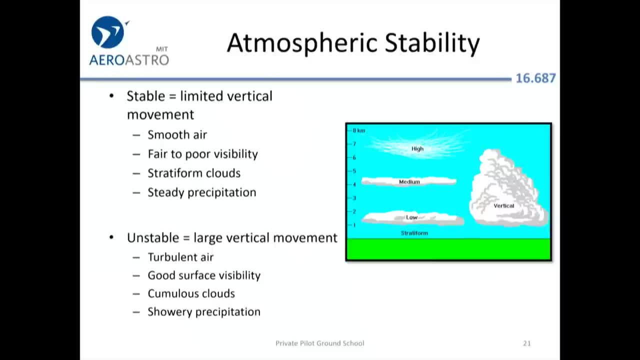 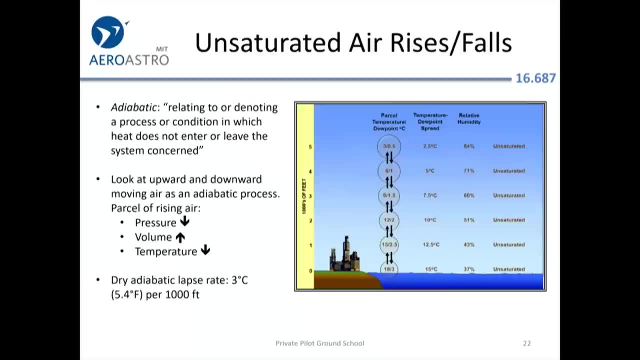 And the rain won't be all day every day. OK, It'll be showery, But it'll be very turbulent if you get into that cloud or maybe right underneath that cloud. OK, What about the profile of the atmosphere? Let's have a look at this. 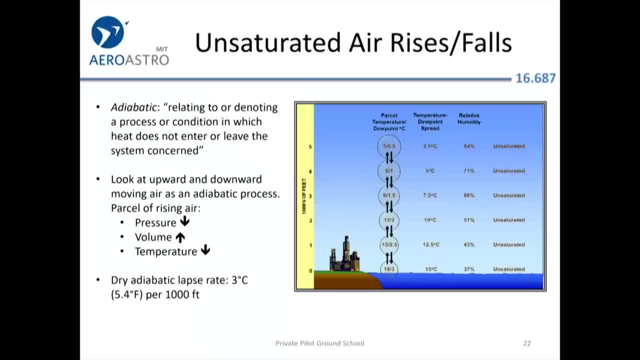 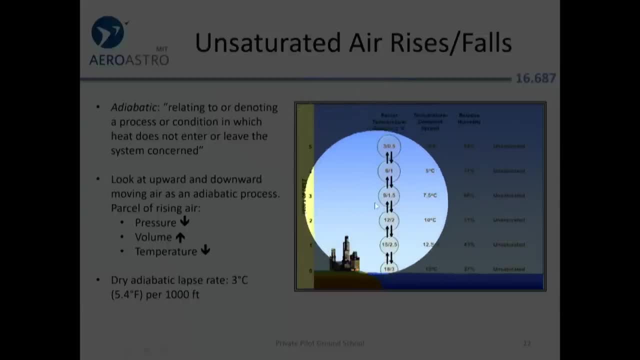 So on the right, I wonder if this is actually my newest version of the presentation. We'll say I corrected an error. But on the right, you can see that for every 1,000 feet you go up. So we go from 0 to 1,000 feet up. 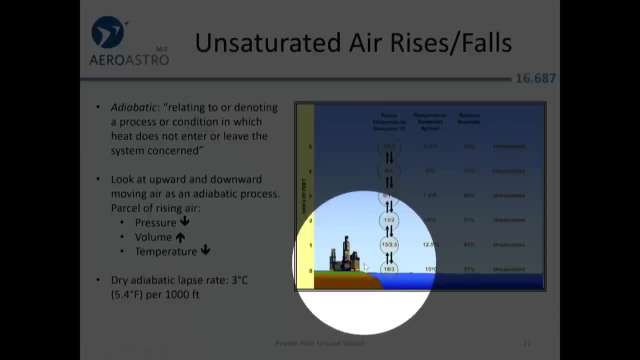 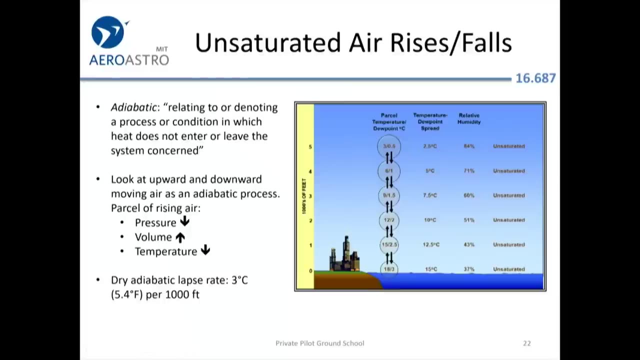 The temperature has gone from 18 Celsius to 15. So it's lapsed by 3 degrees And the dew point has gone down by half a degree. Does that make sense? The air goes up, It's lower pressure. This is called an adiabatic process. 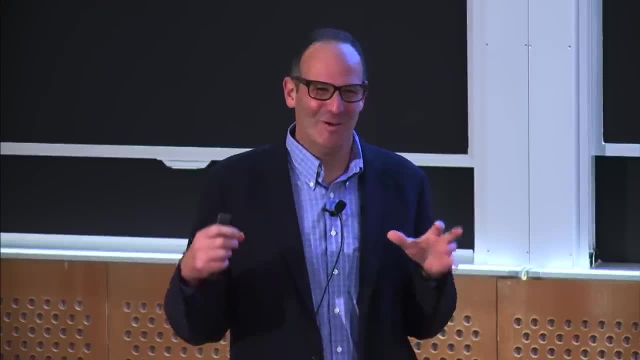 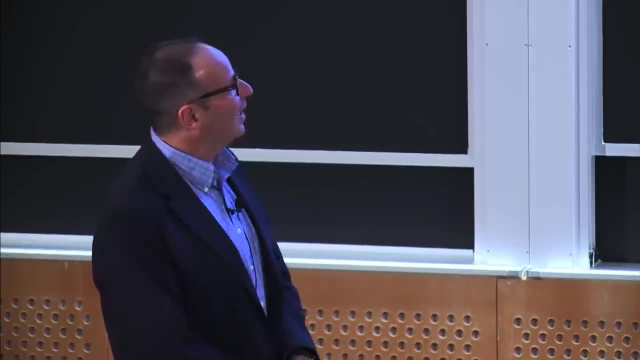 I was not a chemistry major, But I think that means that we're not adding or taking away. OK, We're just moving the heat from the air, We're just moving it, So the temperature and dew point spread actually does get narrower. 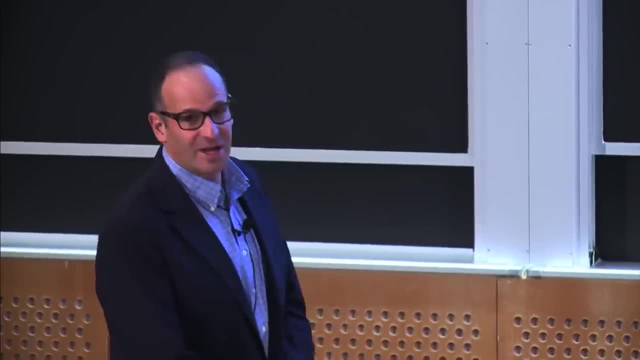 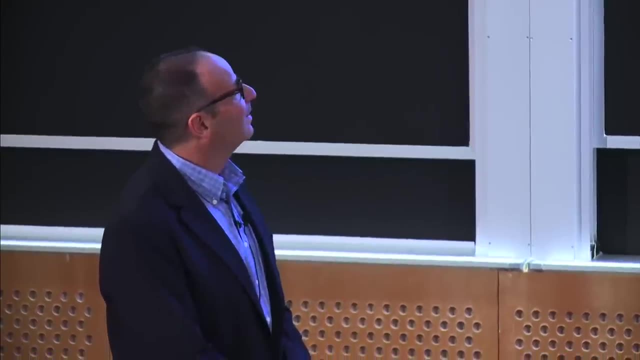 You can see, as we rise up to 5,000 feet, the spread has gone down to 2 and 1 half degrees because the dew point is not falling nearly as fast as the overall temperature. Does that make sense? So I think this conceivably could be an FAA test question. 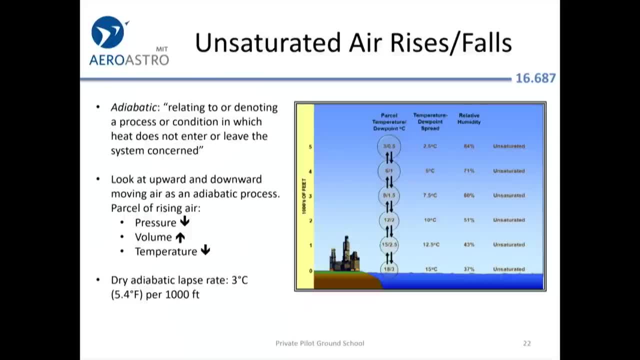 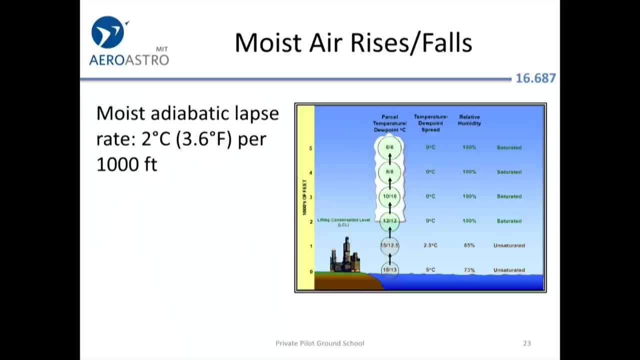 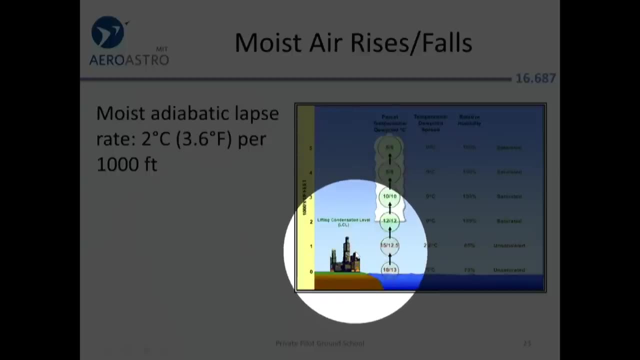 that the dry adiabatic lapse rate is 3 degrees. OK, Then the moist air is lapsing only at 2 degrees. So this figure shows you going from 0 to 1,000 feet, and from 1 to 2,000 feet we're dropping. 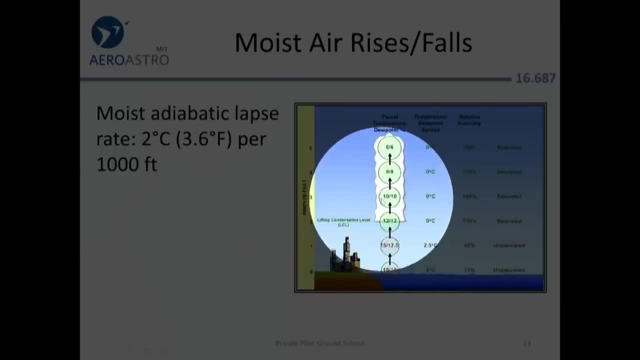 3 degrees per 1,000 feet. After that we're dropping only 2 degrees per 1,000 feet, And once the temperature dew point spread goes to 0, that's when a cloud happens, So the air can't hold any more water vapor. 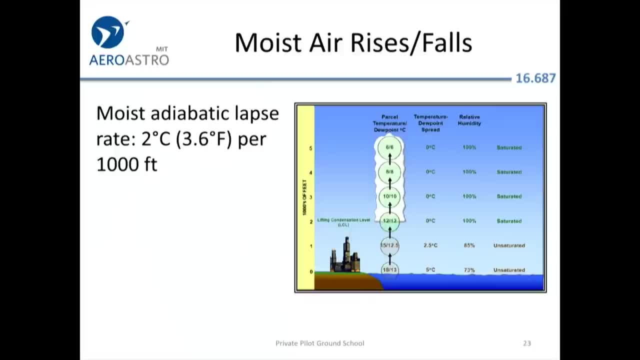 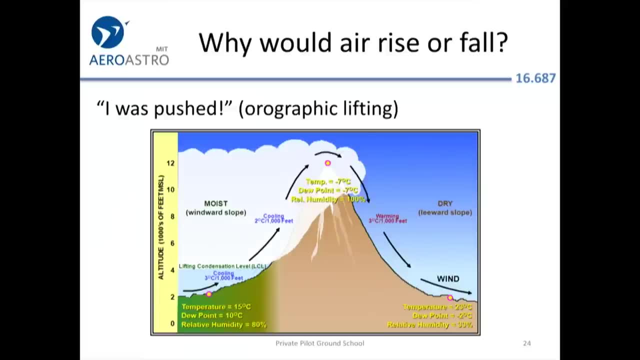 And when the temperature and dew point meet, the water vapor turns into water and I've got a cloud, All right. So you might ask yourself: well, why is this air moving at all? Why does it start moving? One thing that can start it moving is the mountain range. 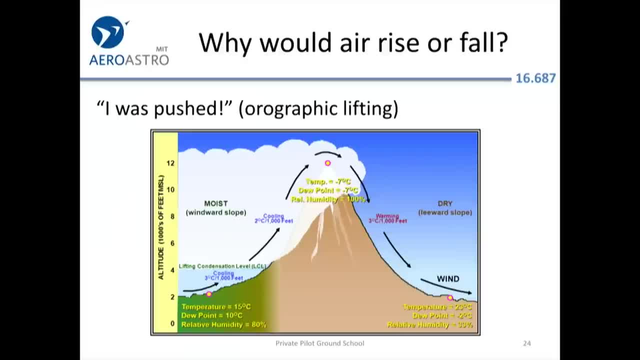 So the air gets pushed by a wind coming from the left, So the air gets pushed by a wind coming from the left side of the slide up to the top of the mountain, And at that point it will condense into a cloud. Just let you absorb that cloud here for a minute. 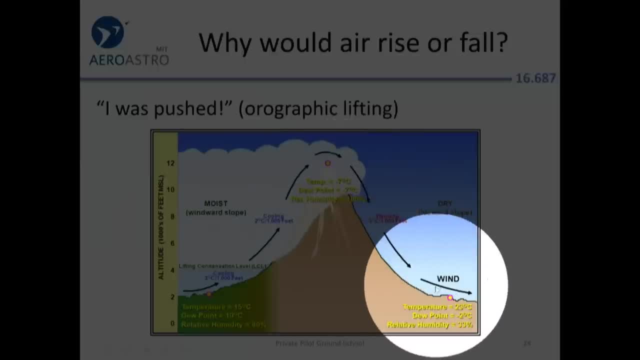 Notice also that relative humidity is just another way of stating the temperature dew point spread. So here temperature and dew point are pretty close: 10 and 15, or 15 and 10.. So we got relative humidity of 80% Over. here they're quite far apart. 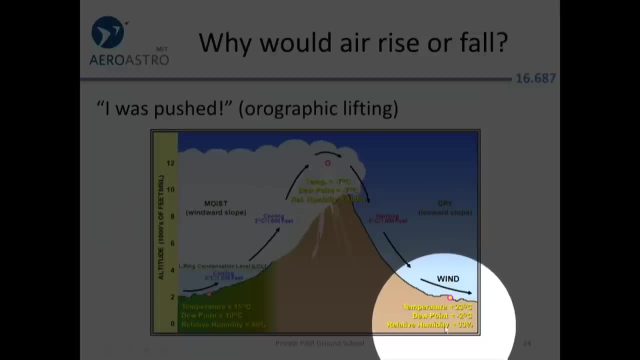 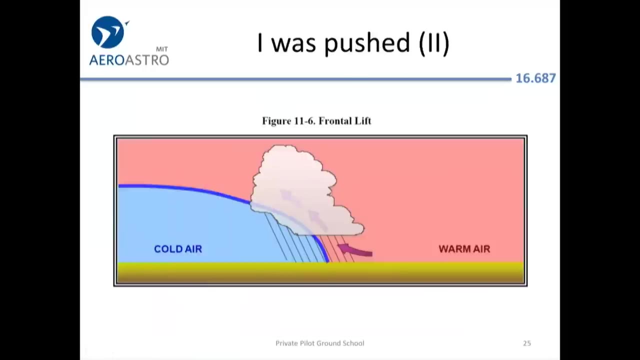 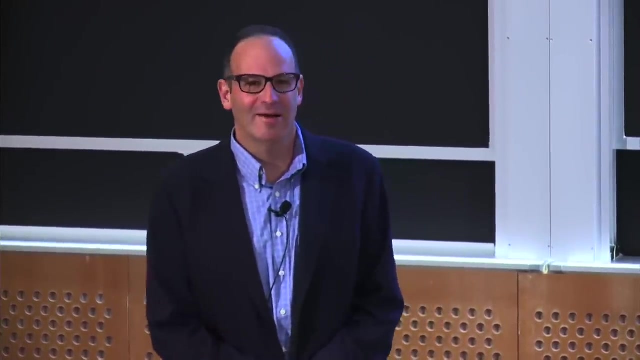 The temperature is 23, and the dew point is minus 2.. So the relative humidity is low. OK, You've heard that there's a cold front coming in and we have all these thunderstorms. Well, this is why The cold air is denser than the warm air. 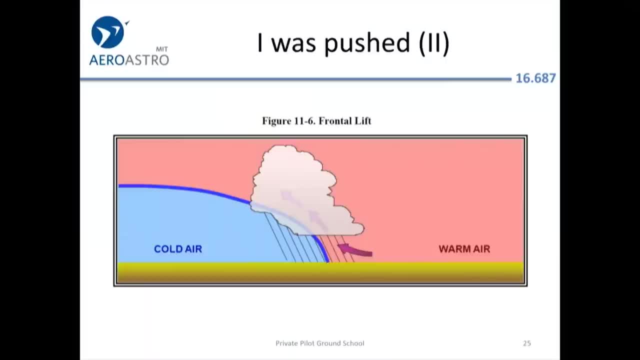 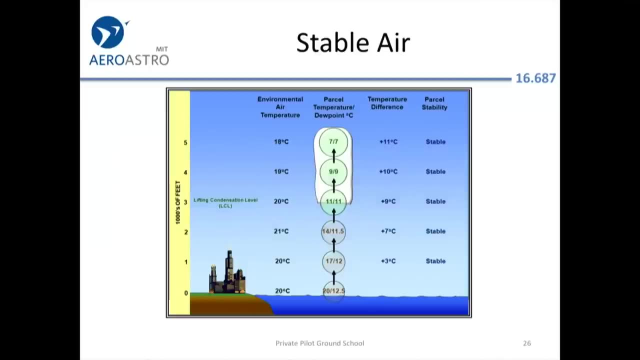 So it pushes the warm air up And at that point you get clouds forming and you get thunderstorms, all along the line of the cold front. OK, so what if you have stable air? Well, let's have a look at this. 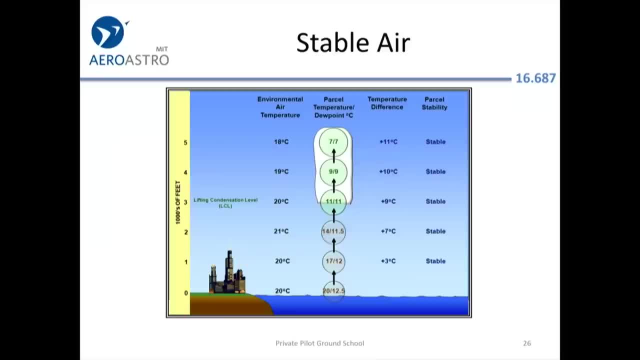 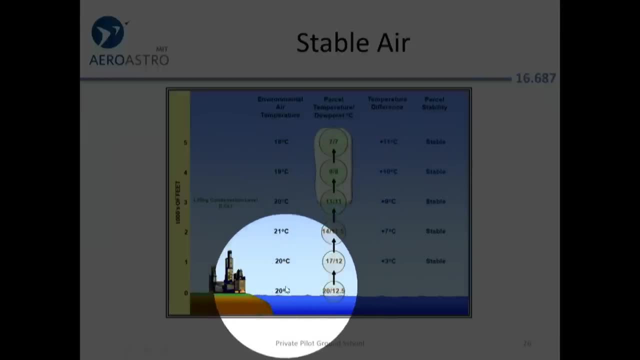 You end up. let's see, we've gone from 0 to 1 to 2, and we've only dropped. we're only dropping- actually we're not dropping at all- and then we're back up. This is the cold front. 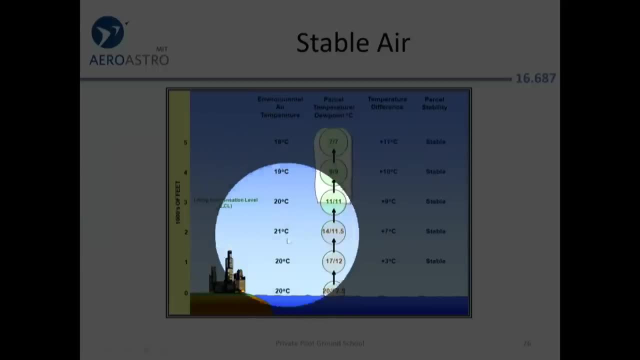 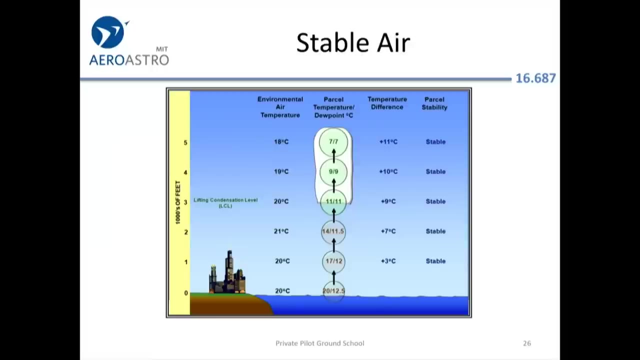 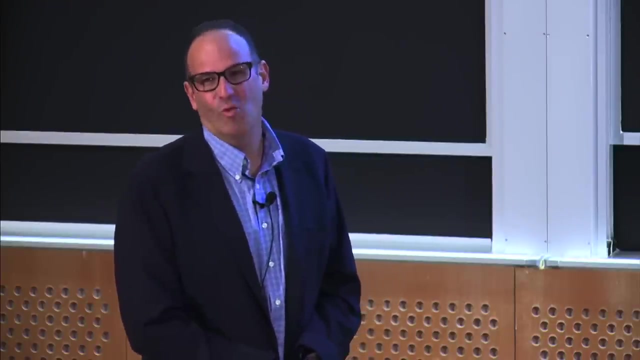 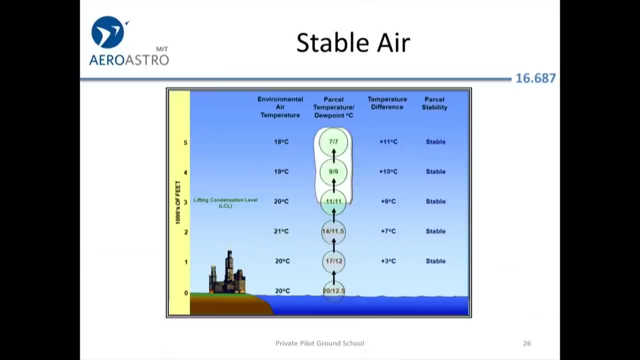 This is an inversion, OK. so basically, the air temperature is pretty constant as we go up. So if a parcel of air rises up into the atmosphere, it's not warmer than the surrounding. it's not going to be warmer than the surrounding air. 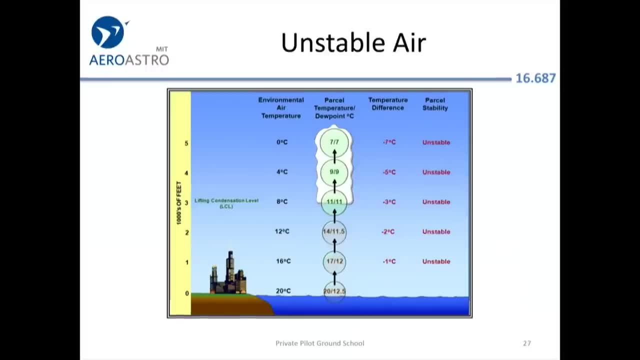 So it doesn't want to keep rising? OK, what if it's unstable? So look at this. by contrast, The environmental air temperature is lapsing at a higher than standard rate. So it's going up, it's going down 4 degrees Celsius. 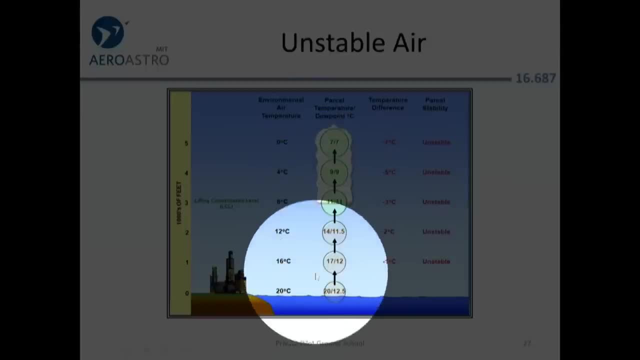 per 1,000 feet And this parcel of air that was in equilibrium down at sea level is still warmer than the surrounding air. So it's going up, It's going down 4 degrees Celsius per 1,000 feet And this parcel of air that was in equilibrium down at sea level is still warmer than the surrounding air. 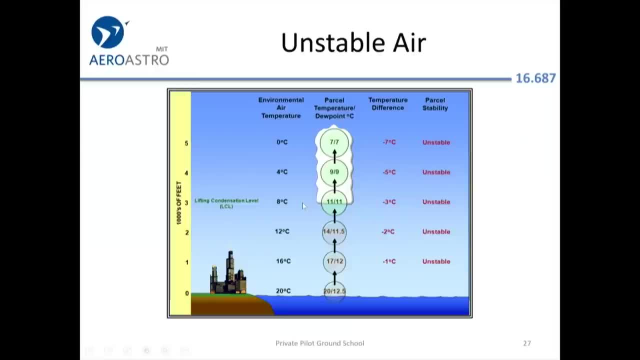 OK, what if it's unstable? It's going down 4 degrees Celsius per 1,000 feet And therefore it wants to keep rising. Does that make sense? So, basically, if it goes up and it wants to keep going up, 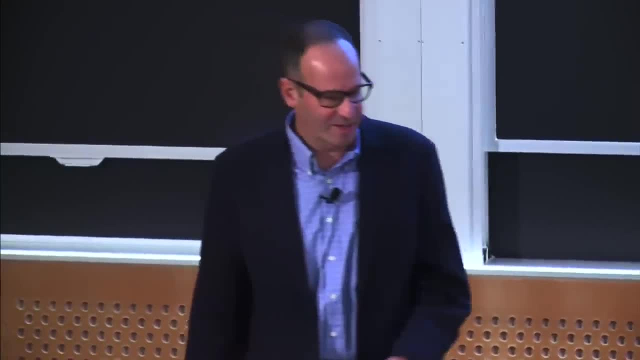 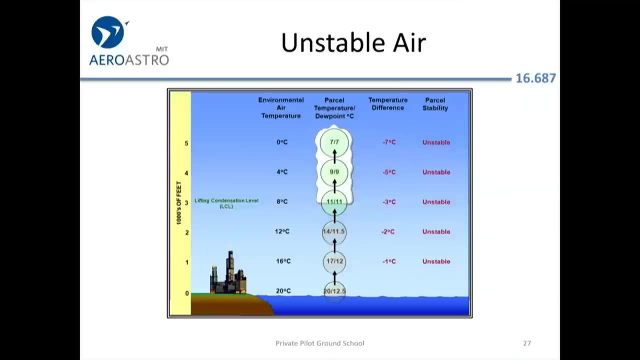 that's unstable and a perfect situation for forming thunderstorms, which we'll talk about shortly. Temperature inversion, like we saw on that earlier slide where it was actually a little bit warmer here. that tends to keep air OK Where it is. 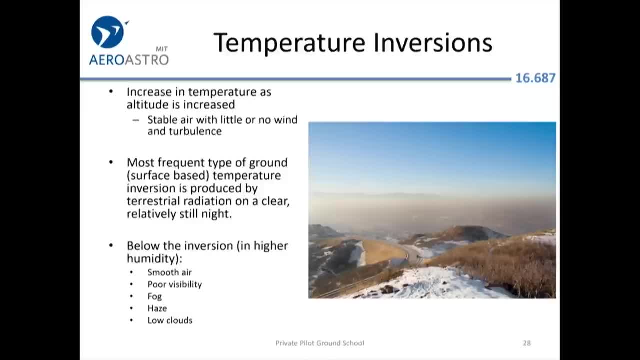 And therefore you end up with poor visibility and haze, because all the stuff that's obscuring your visibility is just staying underneath the inversion. It's kind of a common phenomenon, I think, in some of these basins like Los Angeles. 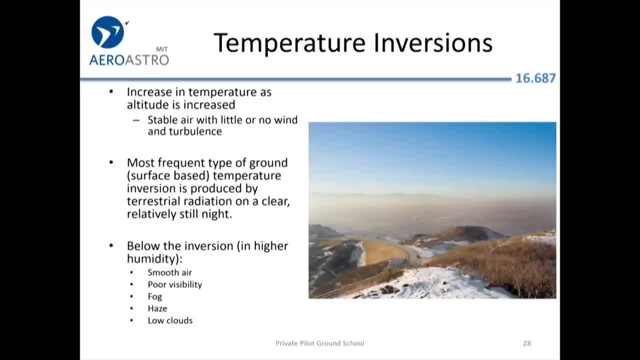 Talk about an inversion and ordinary people think about that and hear that term and worry about it Most frequently. you're going to, I think, see this on the test. maybe is radiation Thought, You know, radiation Phenomenons, phenomena having to do with the ground, radiating. back heat into the atmosphere or into space at night tends to make the ground cold and the air right next to the ground cold, whereas the air just slightly higher than that, a couple thousand feet up, hasn't changed its temperature too much. So the terrestrial radiation on a clear, still night. 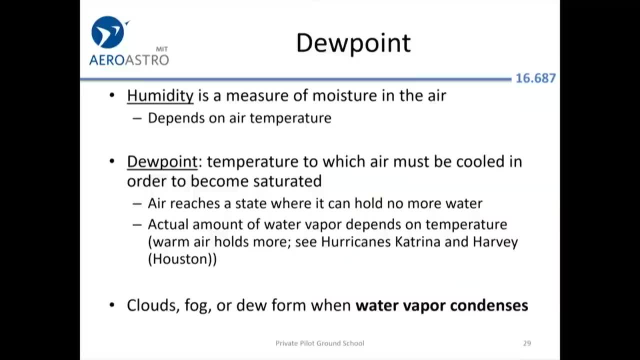 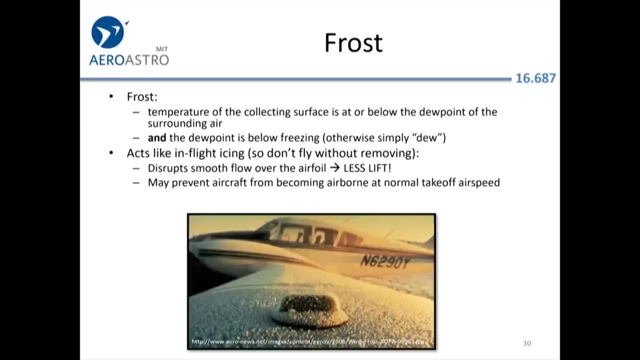 can cause a temperature inversion. We talked about this Earlier. when the temperature and dew point meet, then that's when the water vapor will condense Frost. When the dew point is below freezing and you have a surface that's cold, then you will get maybe. 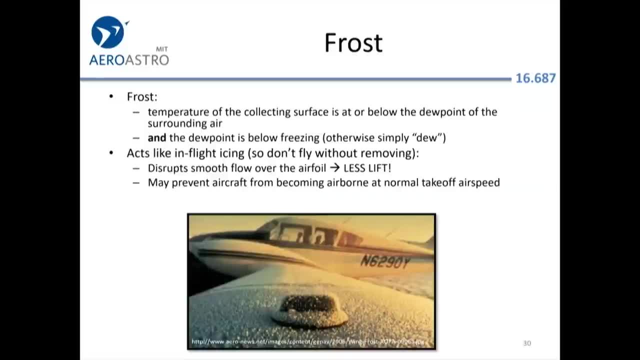 it's cold because it radiated its heat back out into space at night, for example. That's when you get frost forming and you want to definitely clear that off your aircraft before you go anywhere because it messes with the smooth flow of the air. 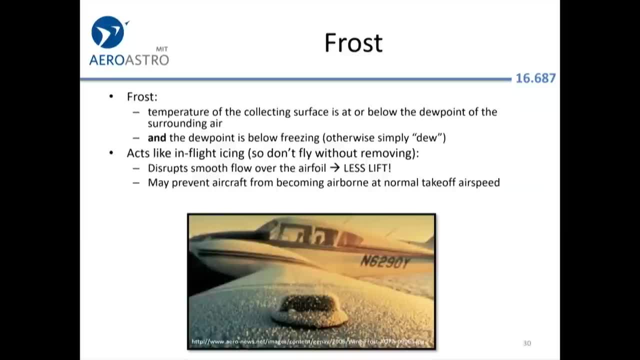 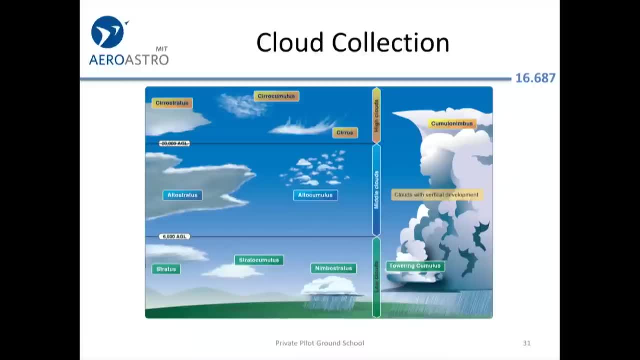 So the wing becomes much less efficient, even if the shape hasn't changed that much. All right, Let's look at the kinds of clouds You've got. basically, the prefix to the cloud tells you what, What height it is, And then the second part of the word. 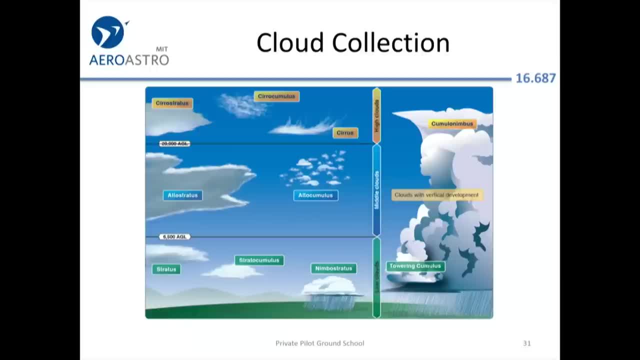 tells you kind of the shape of the cloud. So I'll just let you absorb this a little bit. If it says nimbo or cumulonimbus or nimbostratus, that means it's raining Towering. cumulus is bad if they talk about that. 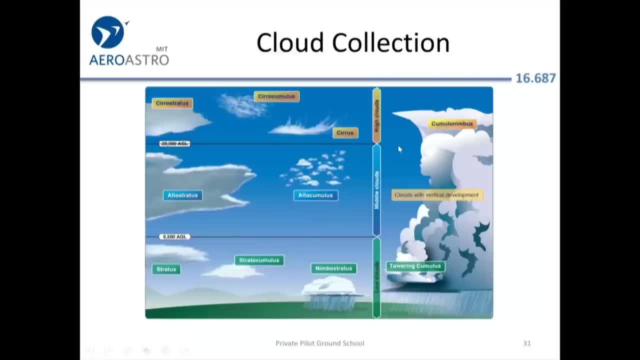 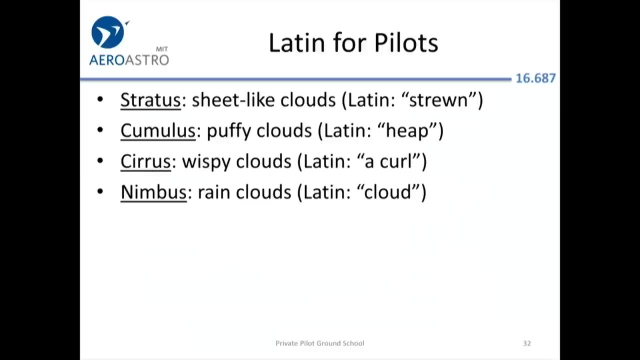 And cumulonimbus is the worst. That's just another fancier way of saying it. That's just another way of saying thunderstorm. OK, So here's your Latin lesson for today. Unfortunately, I didn't study Latin. It would have been nice when I went to Peru. 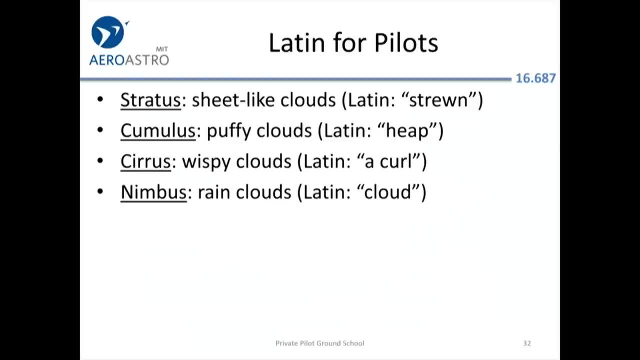 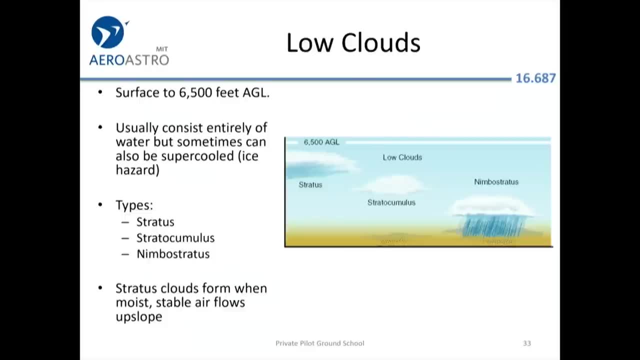 to be able to communicate with the locals in Latin America. OK, That wasn't funny. I guess If you have a local language, So low clouds, the main hazard to worry about is icing. If the water is super cooled, that's the worst. 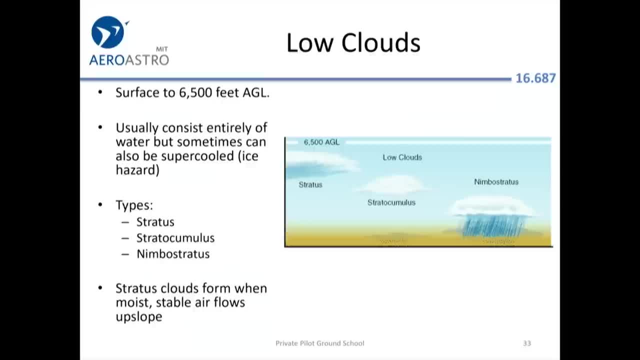 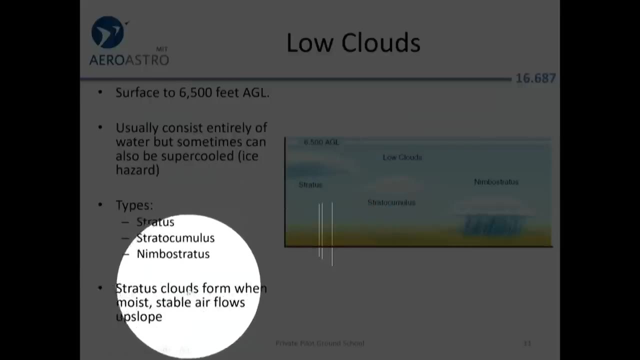 You can usually get a forecast of that. You'll get air mats for icing And they might talk about super cooled water as a hazard. I guess this might be an exam question. Stratus clouds form when moist, stable air flows upslope. 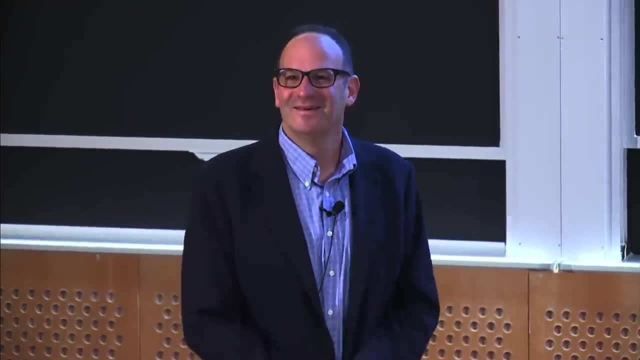 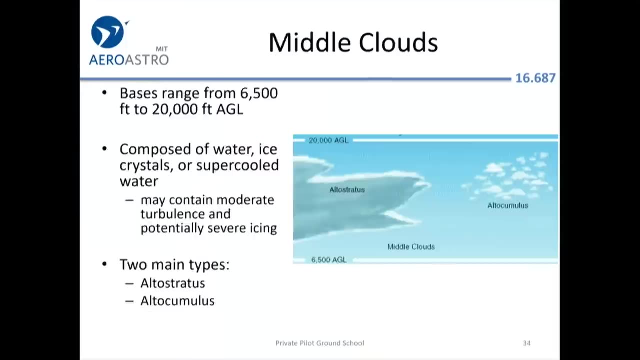 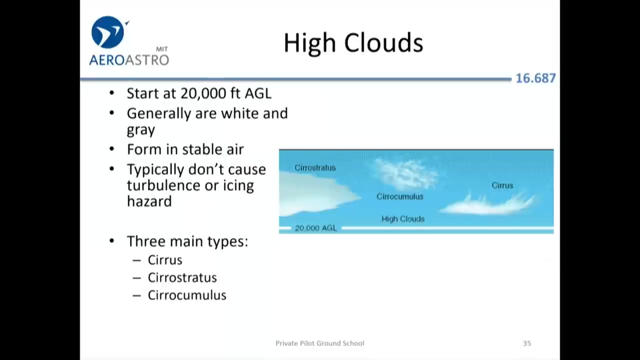 But just remember, stable usually means flat clouds, stratiform clouds And unstable is where you get the cumuliform clouds. So same deal. Those alto cumulus are going to be much more turbulent and probably more severe icing potential. The high clouds. 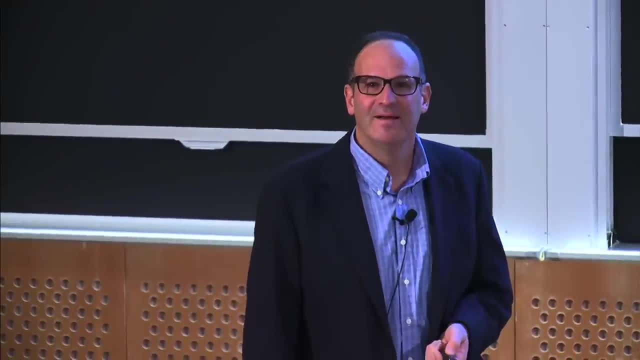 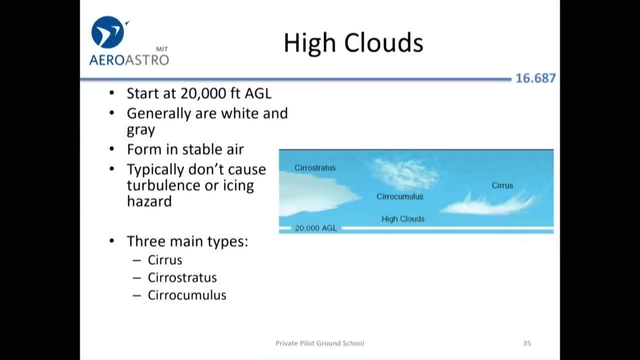 It's so cold in the high atmosphere that the maximum amount of water that can be stored is pretty low, And therefore you don't tend to get ice. when it's below, say, minus 15 degrees Celsius, There just isn't a whole lot of moisture to begin with. 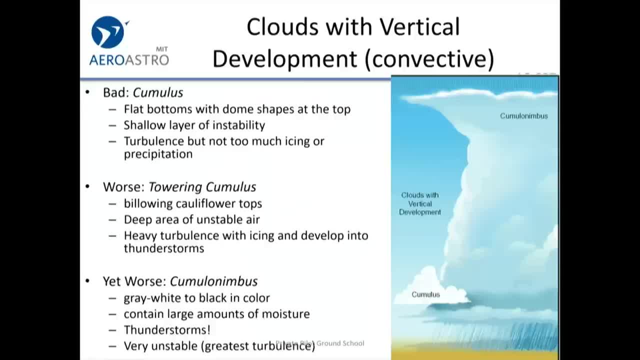 OK, So this is what, as a GA pilot, you're more likely to have to worry about. You're probably not going to be able to do it, You're probably not going to be up at 25,000 feet and you're a Piper warrior. 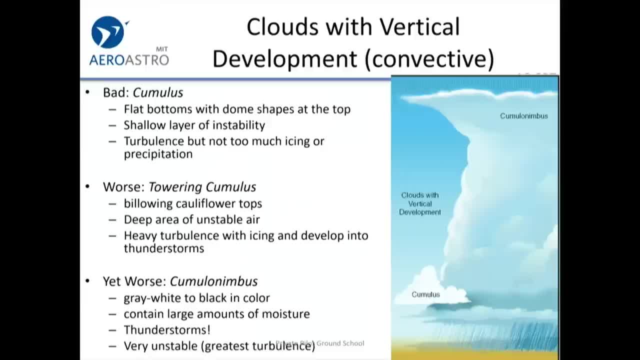 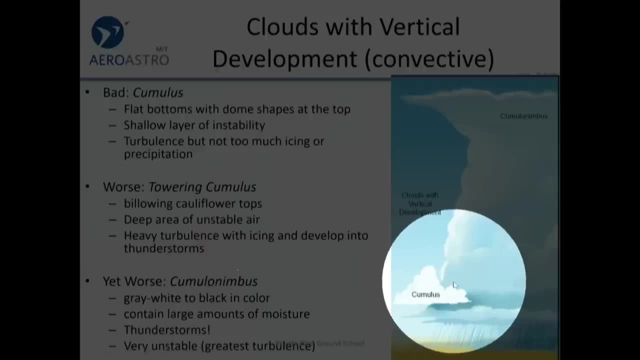 But you could be underneath a cumulus cloud. I will tell you that if you have passengers and there is low cumulus clouds, you desperately want to get above those. So let's say there's a bunch of cumulus clouds at 4,000 or 5,000 feet. 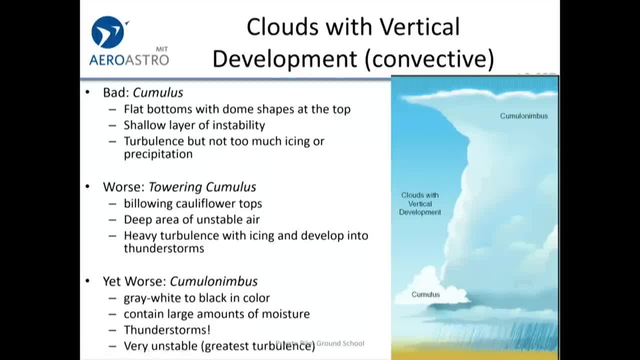 You can climb probably to 8,000 or 10,000 feet in a light airplane And it'll be much, much smoother. So as soon as you get above The cumulus clouds, that's where the air tends to smooth out. 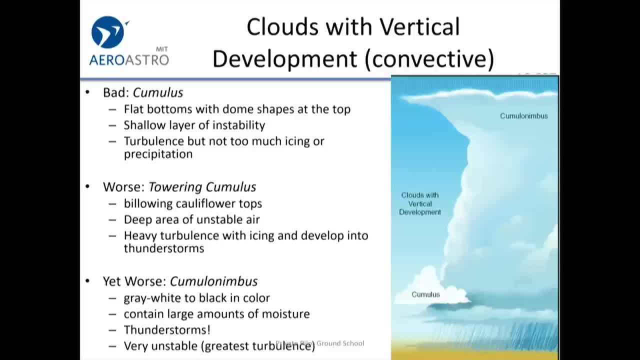 And it will be much more comfortable. But if it's a towering cumulus cloud they may go up to as high as 60,000 feet down in Texas And you really can't get over them in anything short of an SR-71 or maybe LASA's F-22.. 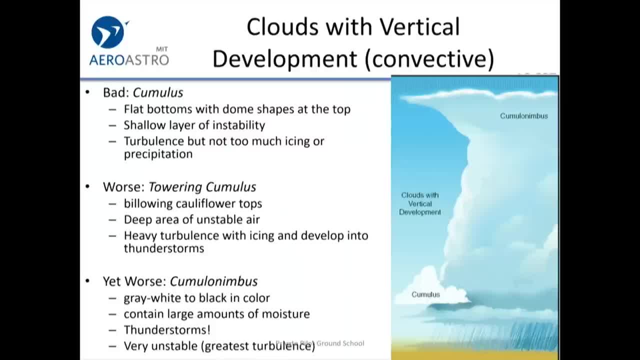 Even the latest Gulf Streams only go to 51,000,, I believe. OK, So thunderstorms are the worst hazard. You know, even airliners get in trouble in thunderstorms, with hail smashing into the windshield and turbulence that can bend stuff. 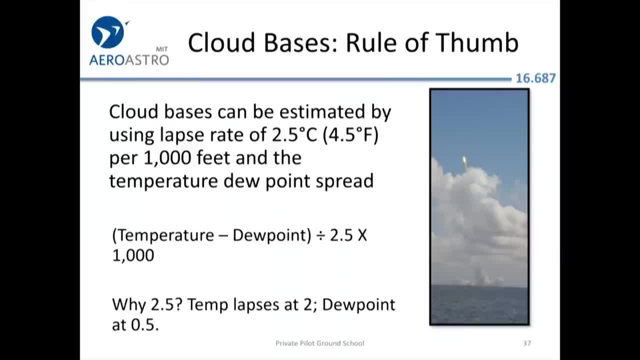 So how do you predict if you're flying along, and well, if you're preparing to go on a flight, how do you predict where the clouds are likely to be? One thing you do is look at the temperature due point spread. The SAA tells you to use a lapse rate of 2.5 degrees Celsius. 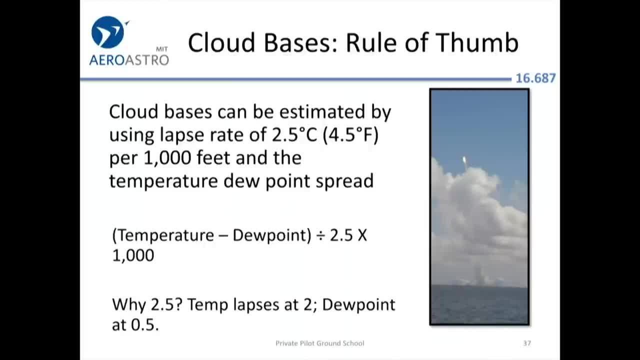 to figure out where the clouds will be. So if there's a 10 degree temperature due point spread, then you should expect the clouds to have a base at about 4,000 feet. There's a typo on the slide. Sorry about that. 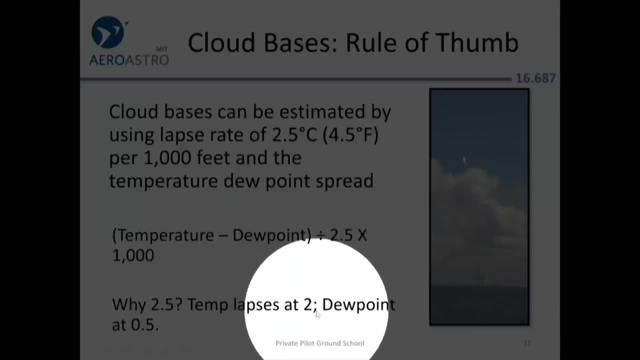 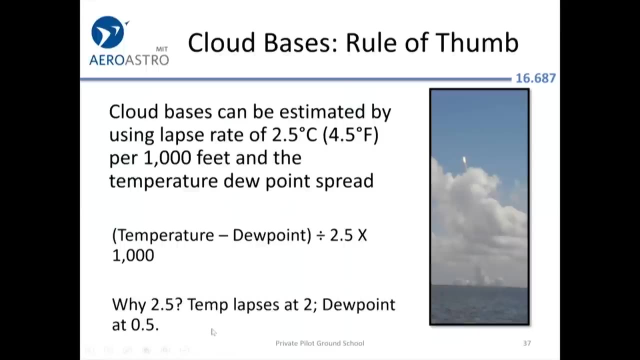 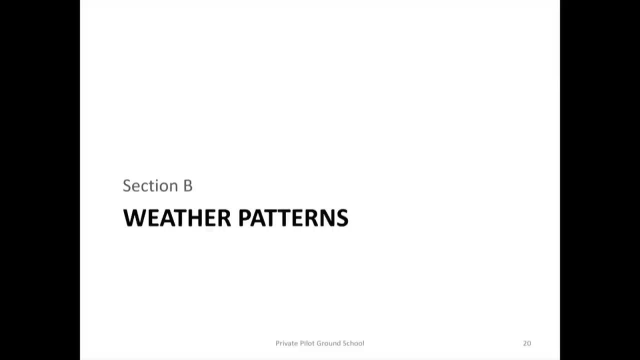 I thought we had the new version in the Dropbox. The temperature lapses at 3 for the dry adiabatic air, You remember that, And the dew point's at 0.5. So if we go back to that figure, I think it was our yeah. 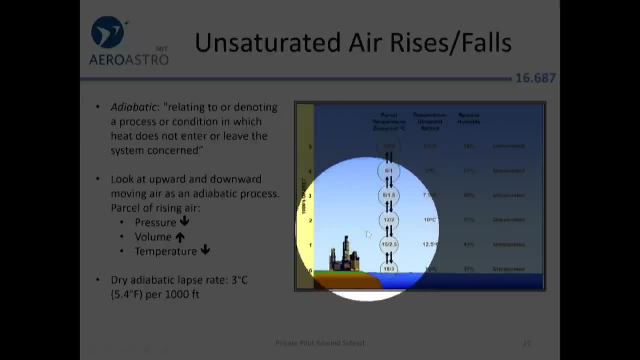 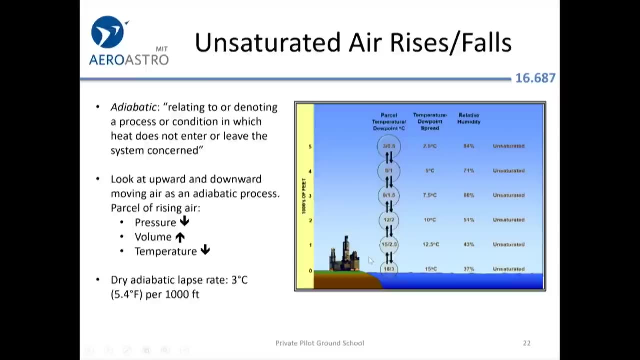 Yeah, if we go back here- you remember this- We went from 18 to 15 to 12. And the dew point, meanwhile, is falling from 3 to 2.5 to 2.. So that's why it's 2.5 as a rule of thumb. 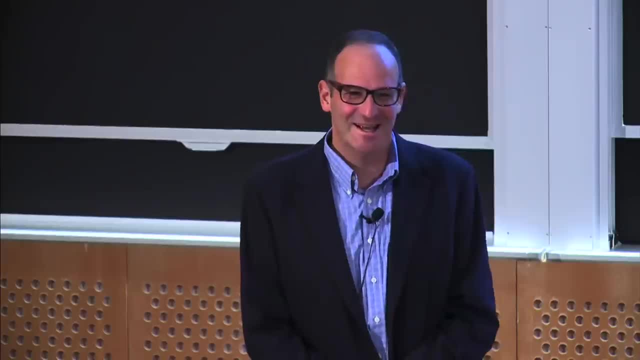 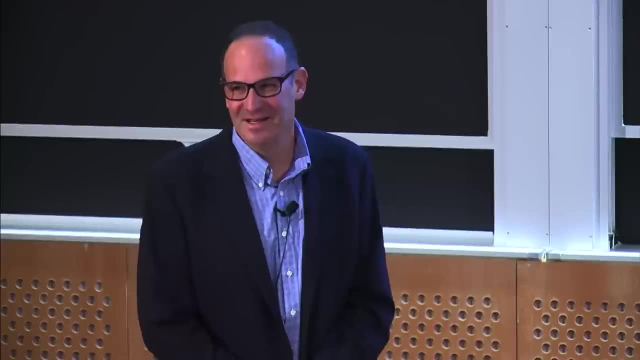 That's not great, But you can actually, if you study, just look at METARs around the country And I think you will see, because they give you the bases of the clouds and the ceilings. I think you usually will see that it's. 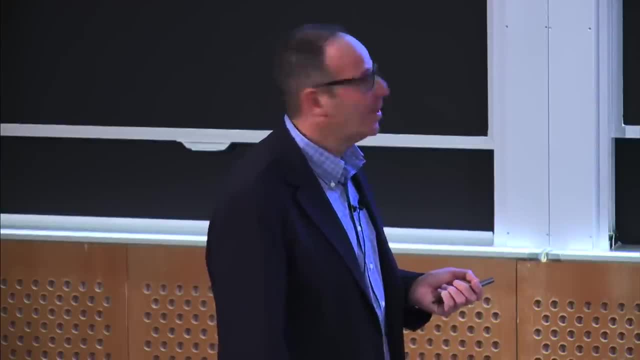 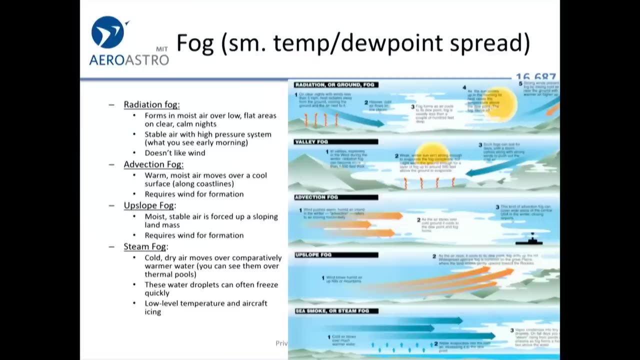 reasonably close to this formula, but almost never spot on. OK, this is worth studying. I'm not going to cover it completely here, But some of these are Exam questions. Advection fog, I think I remember they like to ask about that. 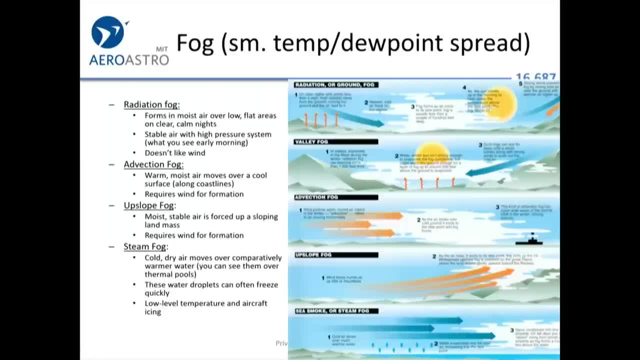 When the warm, moist air moves over a cool surface along coastlines. So I think that makes sense. Maybe that's what they're having in California a lot of the time. You know they have the fog over the coastal areas, I think. 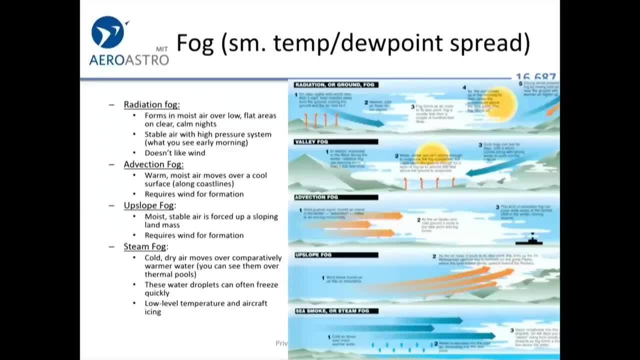 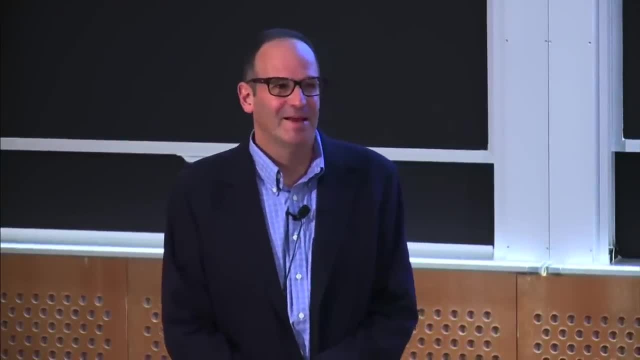 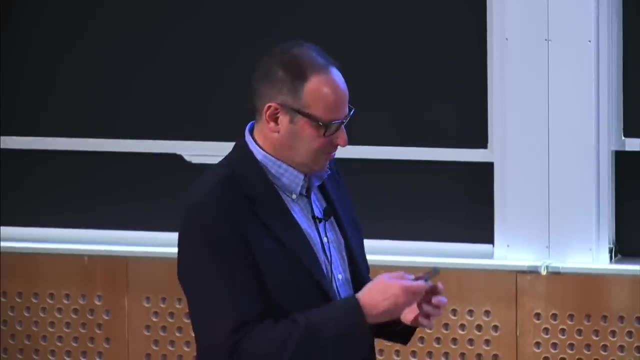 And radiation fog also, like in the Western deserts, oftentimes there's fog in the morning, So I think the air advection fog would be a coastal phenomenon And the radiation fog is something they could have in a place like Arizona or Palm Springs. 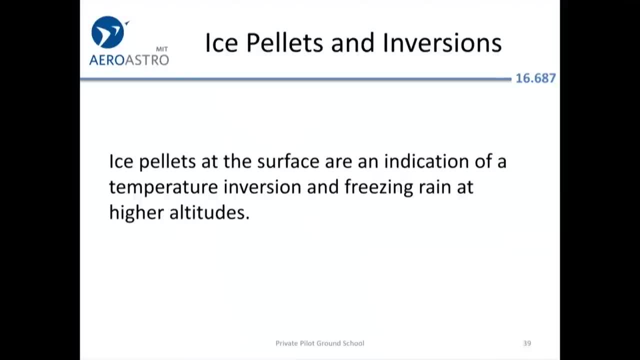 OK, the FAA loves this. If you see ice pellets, you probably shouldn't be flying, But they want you to know that if you do see ice pellets, you're going to be flying. If you see ice pellets, how did they arrive? 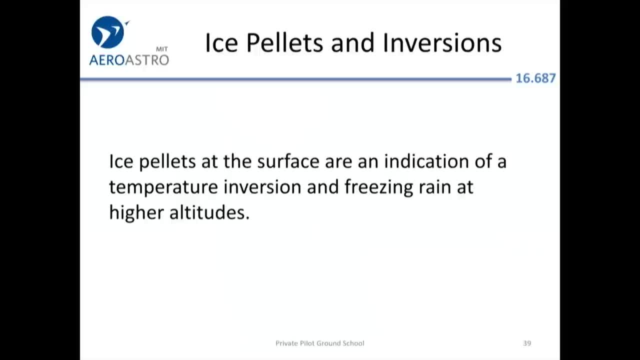 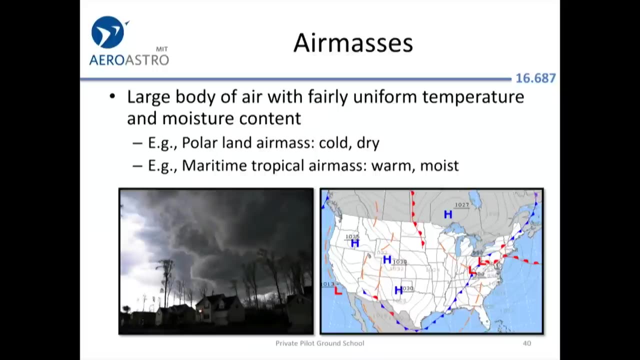 Well, they had to be freezing rain up higher. So don't climb in hopes of getting out of the ice pellets, because then you'll have freezing rain on your airplane, which is probably the worst kind of icing-related hazard. OK, air masses, you can just have a look here. 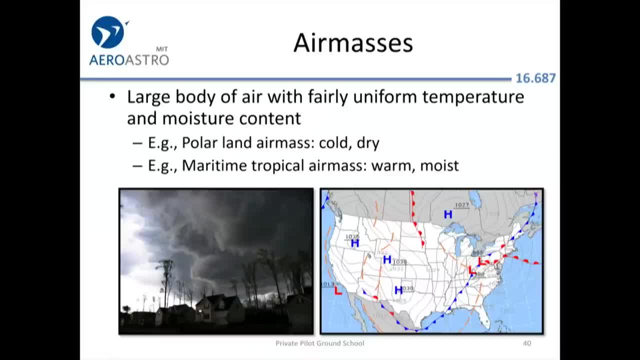 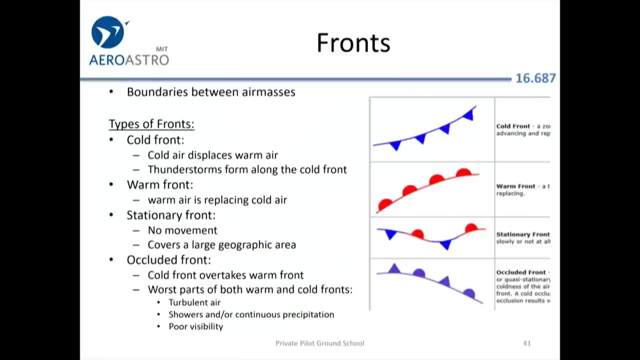 Basically, if you hear that there's a polar air mass coming in, it's going to be cold, Not too exciting. Might be a question, Fronts, they do want you to be able to read one of these maps. They may occasionally ask you a question. 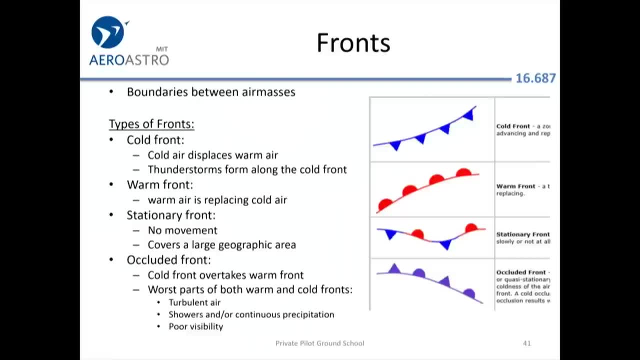 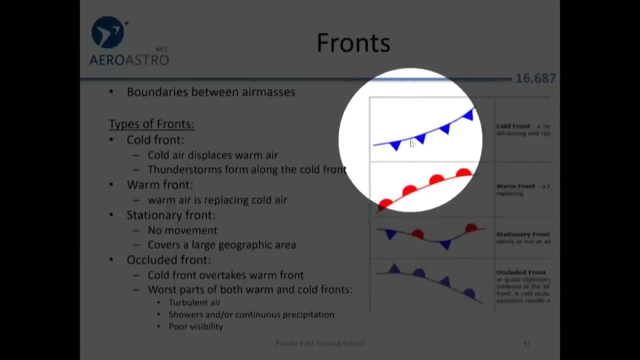 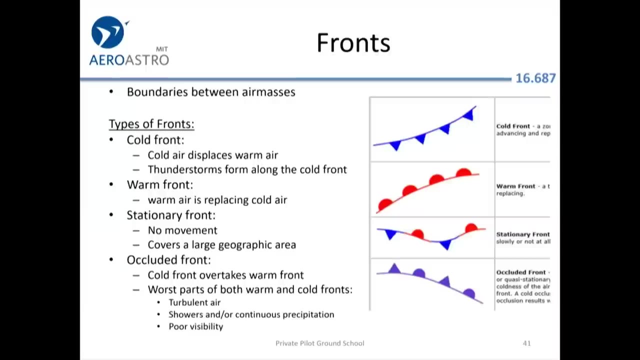 So one thing to remember is the cold front has the pointy spikes like icicles. So if you can remember that, you'll be pretty good. There's a cold front Again, you can OK. OK, I'll just kind of read this and study it at your leisure. 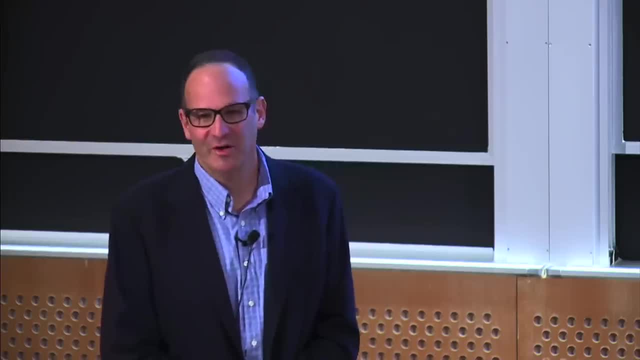 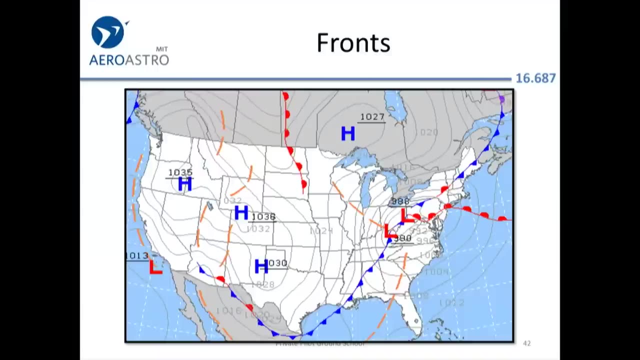 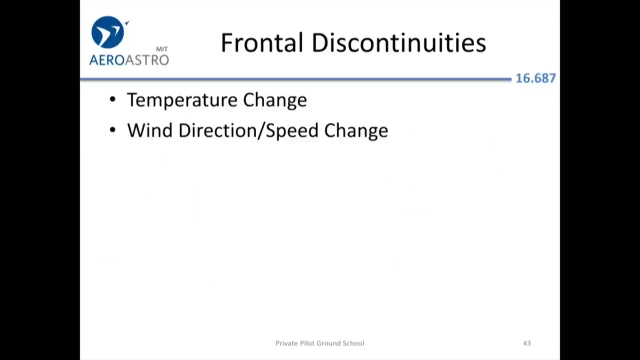 I guess they might want you to remember that the front is the boundary between two air masses. OK, here's a typical drawing where they'll show you the cold fronts and the warm fronts. When there is a front, how do you know when the front has gone through? 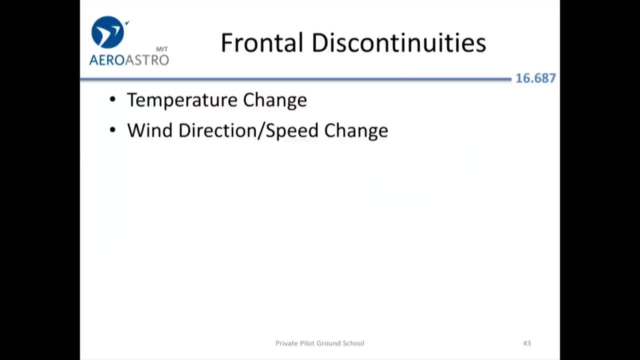 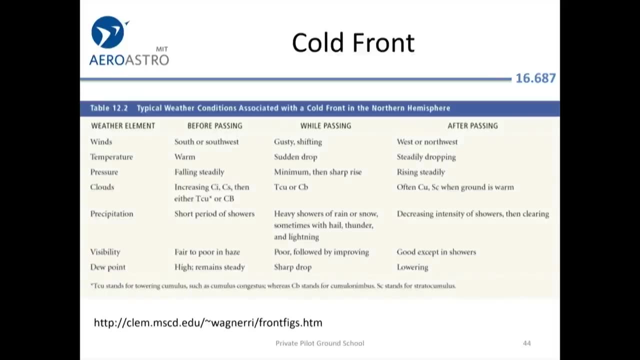 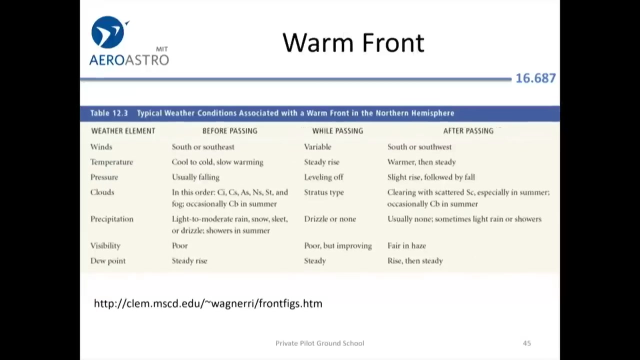 Well, the temperature has changed and the wind has changed. Simple as that. So here's a little explanation of what you can expect. when a cold front goes through, Everybody's happy with that, OK. When a warm front goes through, it gets warmer afterwards. 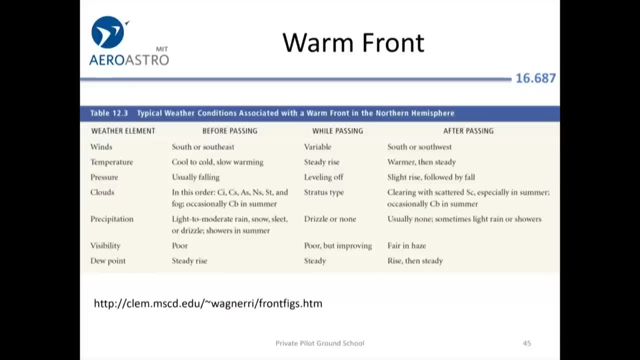 Ha, Ha Ha. Yeah, So the warm front produces, as you can see, light to moderate rain drizzle. the visibility is bad. That's actually the important thing here. Look at the visibility: It's poor, and then it becomes fair and haze. 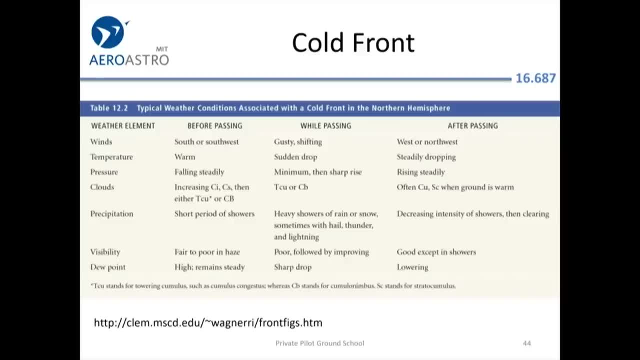 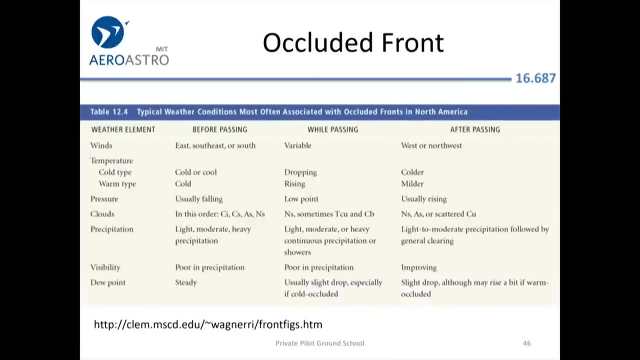 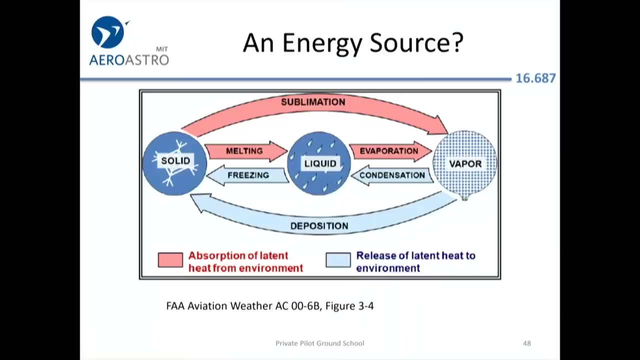 whereas the visibility becomes really good after a cold front comes through. So that's the way this looks. So, with no heat, we have very bright, cloudy, cloudy fronts and occluded fronts. same deal: Bad visibility. All right, let's talk about hazards. 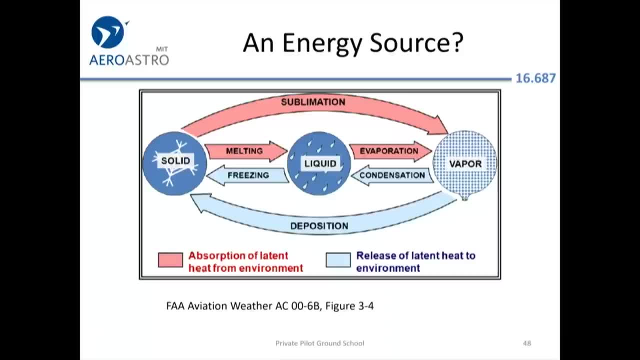 This is more important. So this is a summary of where heat is released into the atmosphere versus absorbed by water. Water goes, for example, from vapor to liquid. It releases heat, So that's exactly what's happening when it's raining in a thunderstorm. 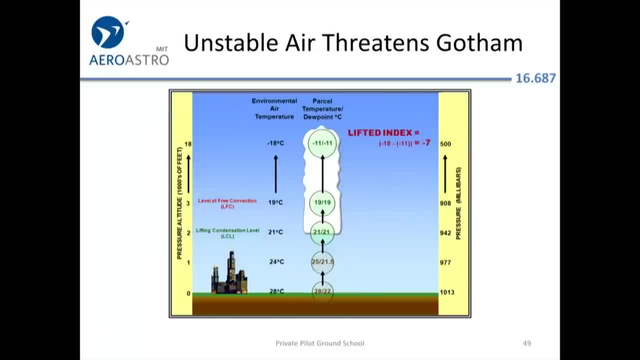 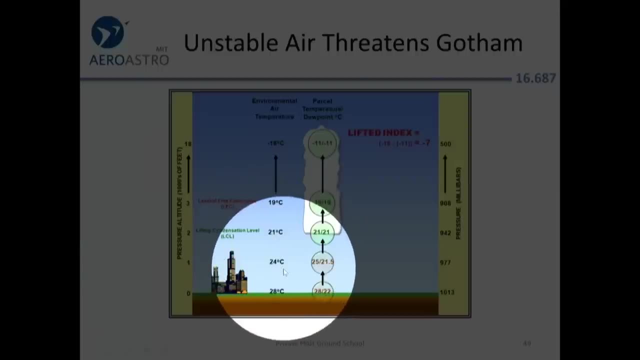 And that's not a good thing. All right, so here's the FAA's chart of a cumulus cloud forming, So you can see the lapse rate over here in the ambient atmosphere. It's going from 28 to 24 and down to 21.. 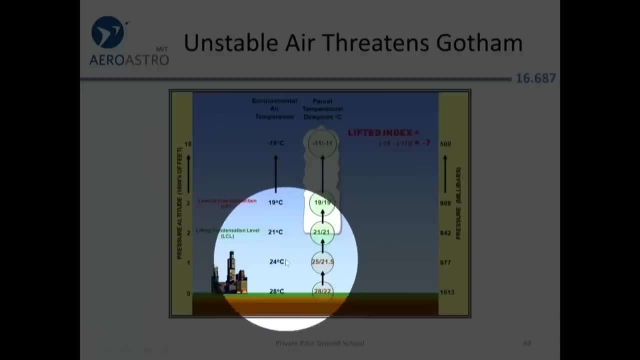 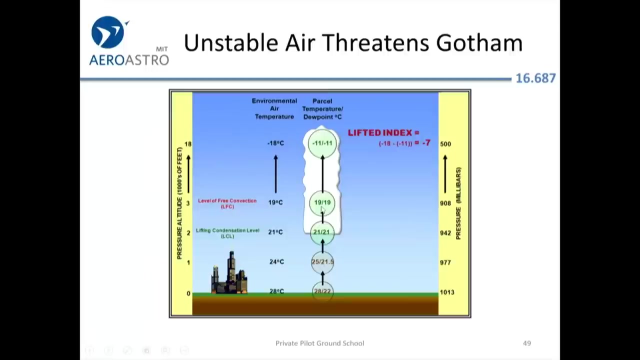 So it is, at least initially, higher than standard lapse rate. So this warm air, it starts at 28, and then it drops only to 25. So it's still warmer than the surrounding air. So it goes into becoming This big, nasty cloud. 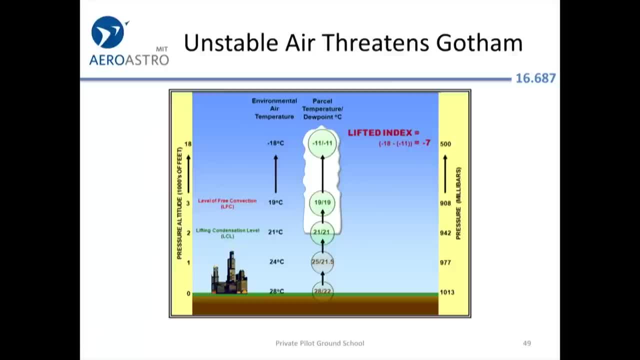 There's this you can kind of see. if you don't want to look at the summaries of weather forecasts, you can look at these charts of lifted index Here. it shows the difference between minus 18 and minus 11 of minus 7.. 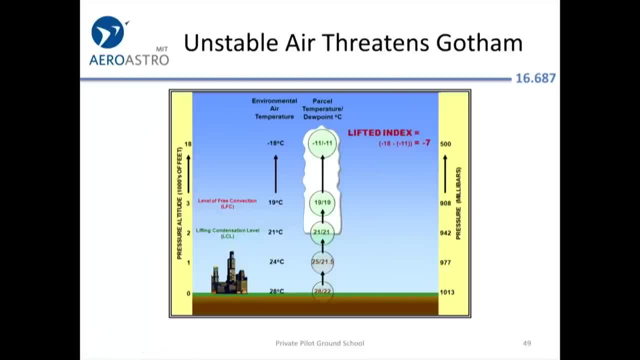 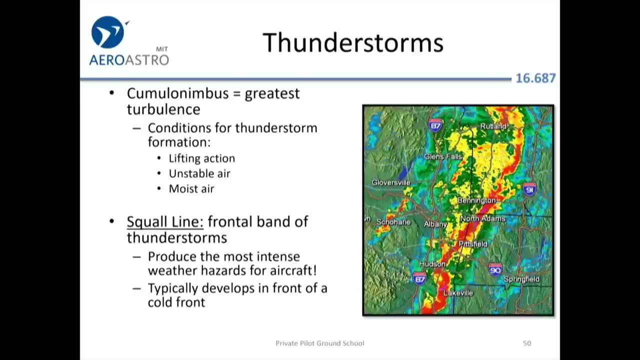 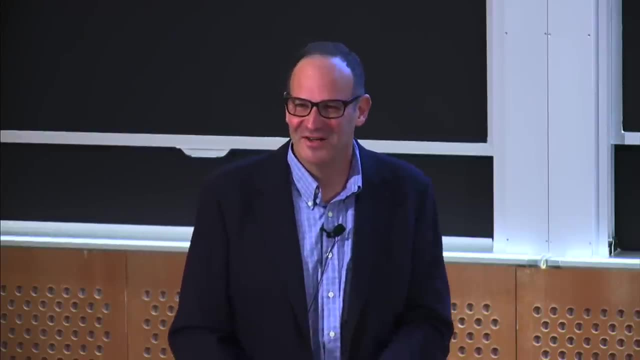 That gives you kind of a measure of the thunderstorm potential. There are charts of that, But as pilots this is kind of more what we deal with on a practical day-to-day basis. We just look at the NEXRAD data from the radar stations. 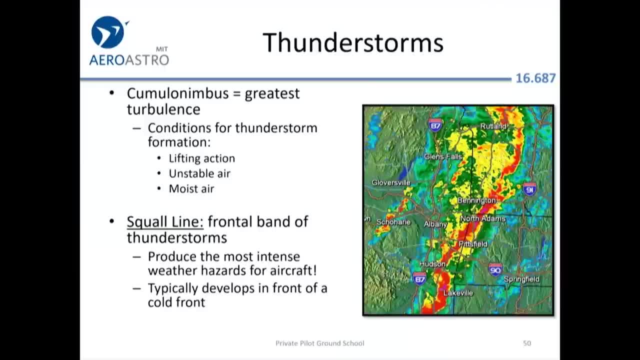 that are strewn around the country, And if it's red, we try to find a path around it because there's just not much else you can do in a little aircraft. It's possible that you could get over this entire front if you were in a jet that could climb up to 40,000 feet. 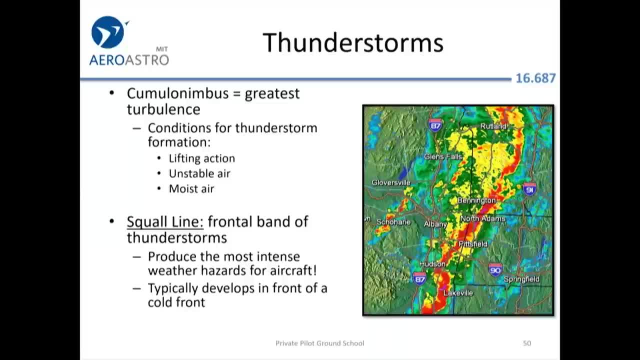 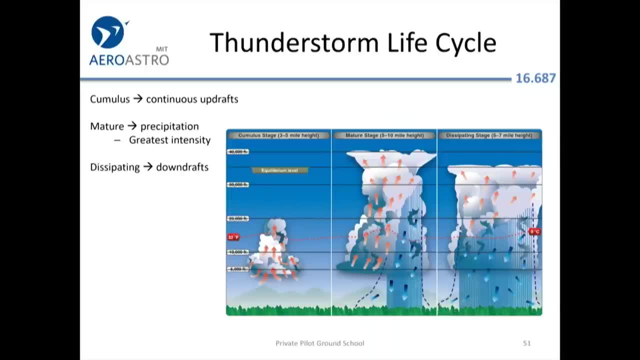 or higher. But you know, In a Piper or a Cessna or a Cirrus you're just not going to be able to do that. OK, The thunderstorm life cycle. This is, I think, a favorite test question. 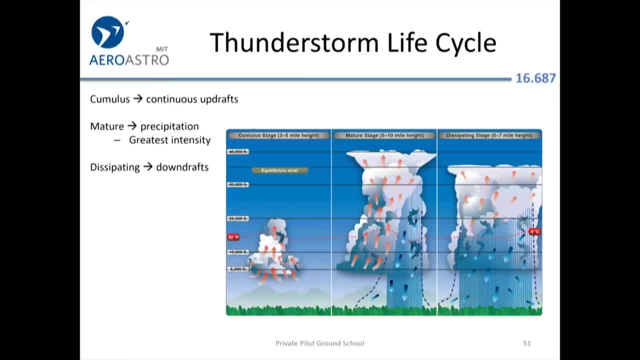 How do you know that the thunderstorm has reached its mature stage? Well, it's raining. Simple as that. If it's raining, it's mature. If it's dissipating, you're going to get these downdrafts. If it's building, you get updrafts. 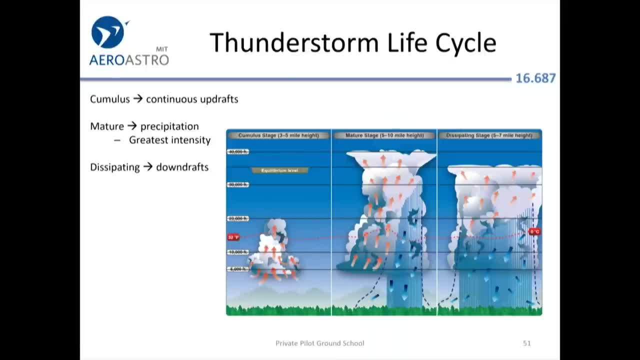 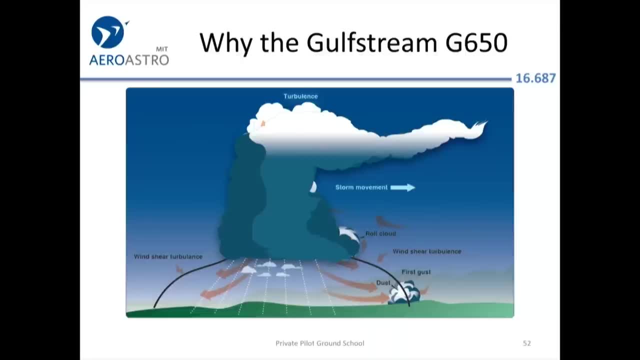 So everything comes up and then it all comes down. OK, Look at that nasty thunderstorm. You're going to get turbulence right on top of it. If you can clear that thunderstorm by 5,000 feet, it'll probably be nice and smooth. 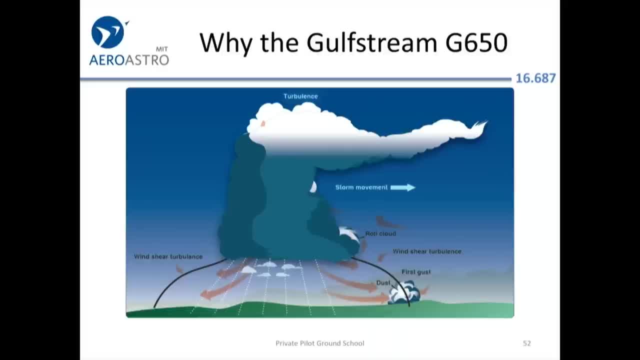 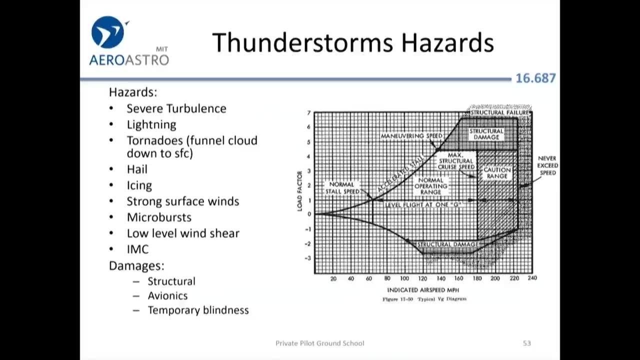 So this is your good argument for a plane that can go to 51, flight level 510.. Airliners don't go that high. The latest biz jets go much higher. They're much higher than airliners. All right, The hazard. we're going to hear more about this tomorrow. 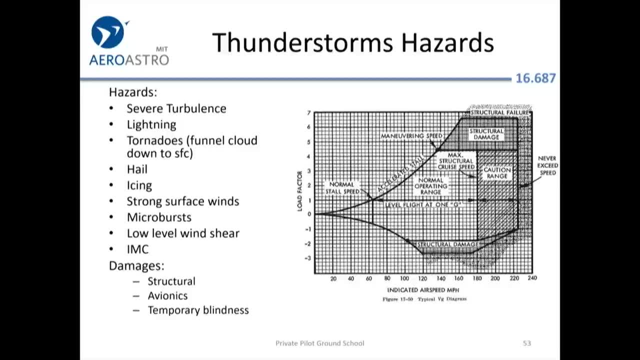 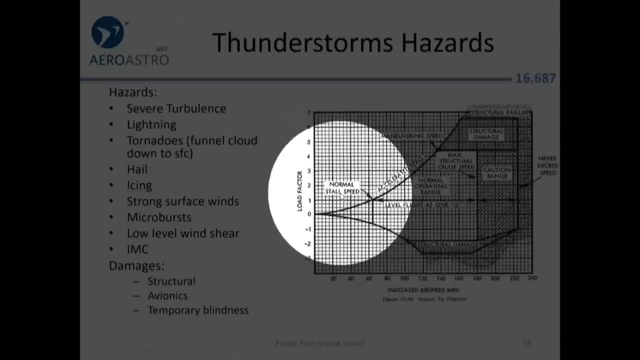 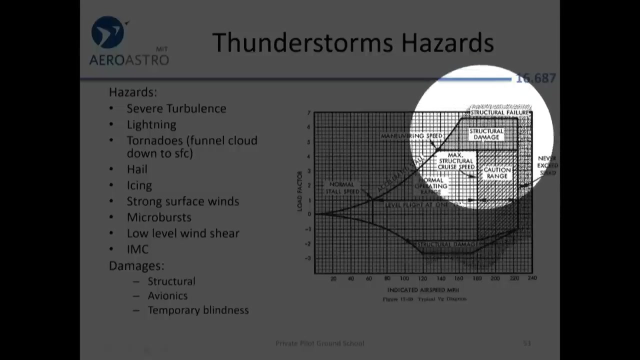 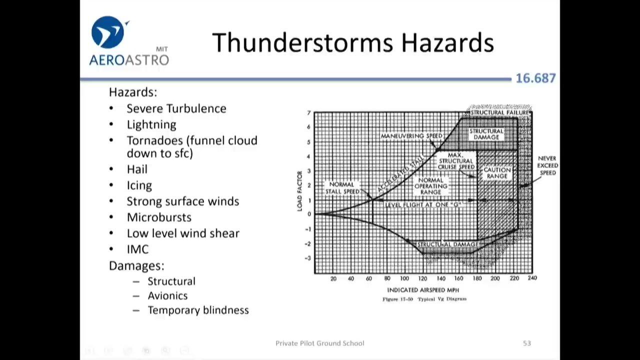 from Dojo, from the Brazilian Air Force. But there is this chart here that shows you how much load factor that's in Gs. If you're going pretty fast, you can pretty quickly- OK- get into the structural damage range. So that's why they tell you this. 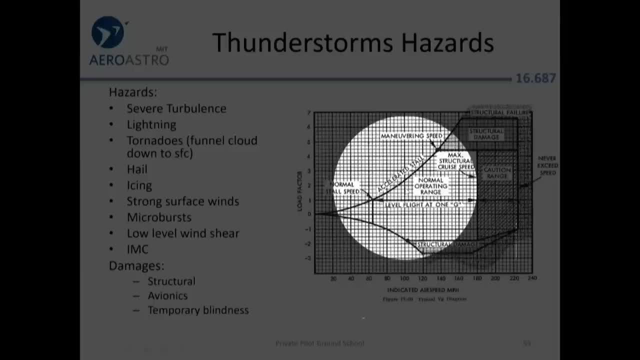 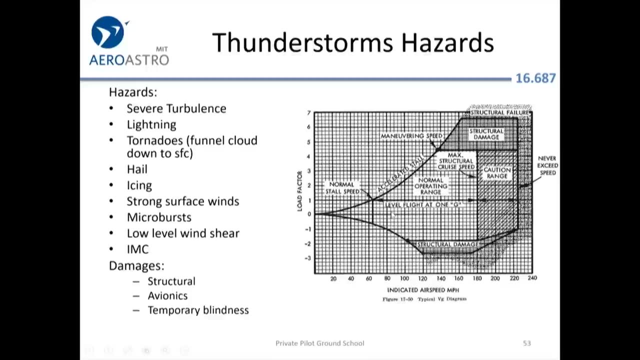 These lines here are basically. this is how many Gs you can get on the aircraft with either extreme movements on the controls or extreme movements that are imposed on you by a thunderstorm or something. So the takeaway from this diagram is: slow down if you get into heavy turbulence. 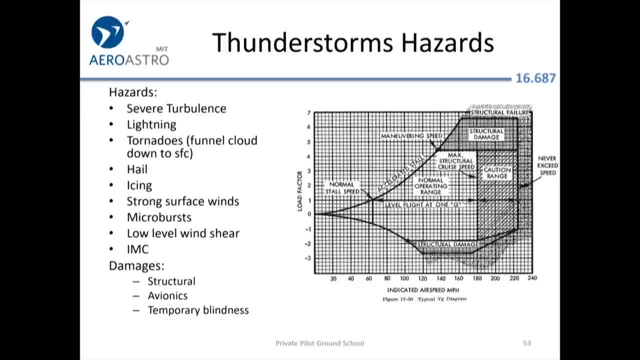 because then the airplane will stall before it bends And the stalling can be corrected by pushing the nose down. OK, so these are all the hazards from thunderstorms. Again, it's a lot better In this day and age. there's so much information out there. 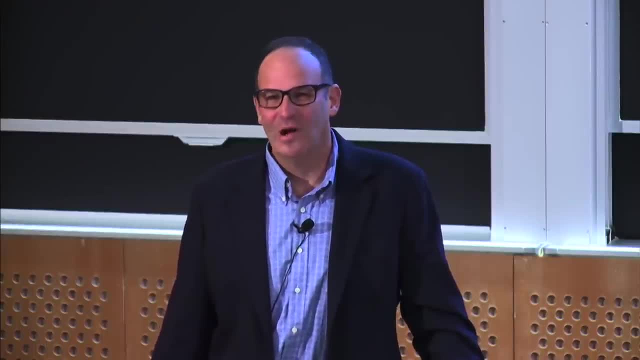 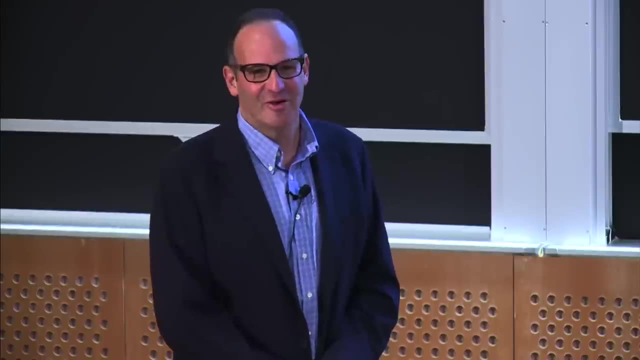 and data link available in the cockpit- that going through thunderstorms is just much less common than it used to be And therefore it's a lot better, And therefore you don't really have to remember too much other than don't fly through a thunderstorm. 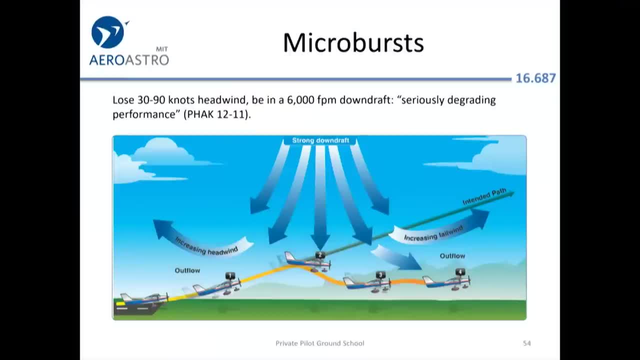 Microbursts. however, if you're trying to land and beat the thunderstorm, you can actually get into a little bit of trouble, because the wind right before a thunderstorm or right after can be pretty squirrely and cause you some difficulties. 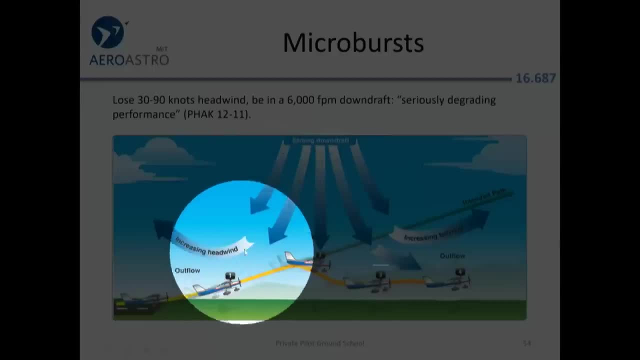 here. So let's see what do we have. So here this airplane is getting a performance boost from a strong headwind. Now not much is happening, except that it's getting pushed down, maybe faster than the airplane can climb. 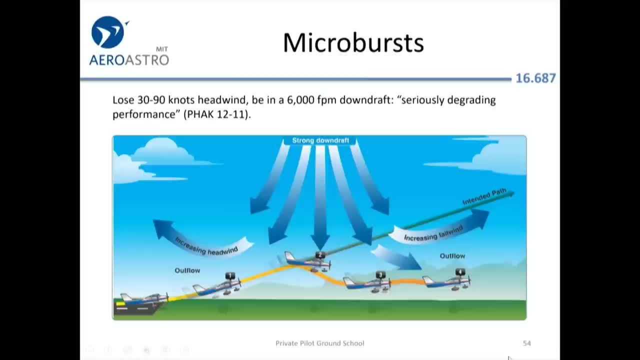 And at this point you're getting a performance reduction from this big tailwind. So you might think: well, that's great, I'm getting pushed along with a tailwind, But if it's suddenly taking away your airspeed, then that's not. 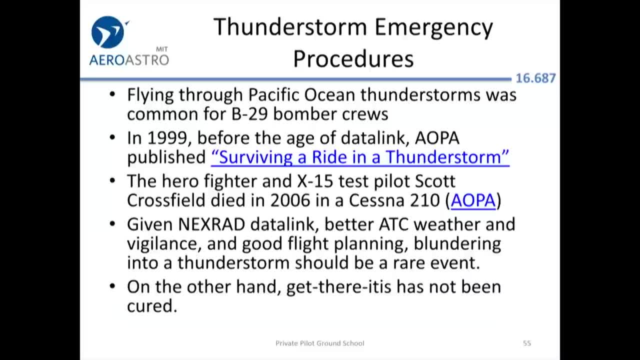 a performance boost, All right. so the thunderstorm emergency procedures are again probably a little bit less relevant now that we're living in this world of constant data link and NEXRAD data 2006,. there was a famous accident with a former test pilot, Scott Crossfield, who maybe 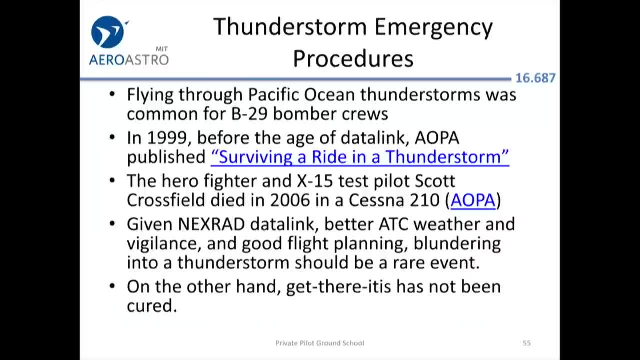 didn't get the best advice from air traffic control And I don't think he had data link in his cockpit- The Boeing B-29 bomber crews. they would fly, I think, seven or eight hours from an island in the Pacific over to Japan. 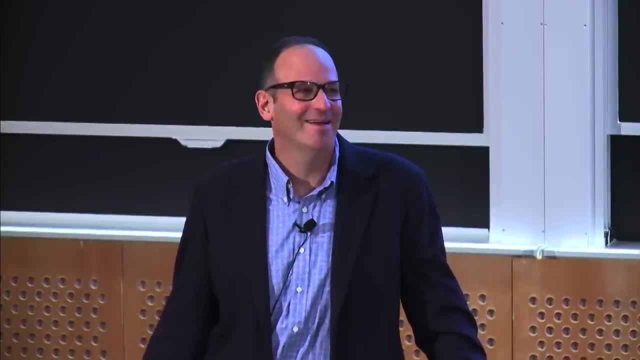 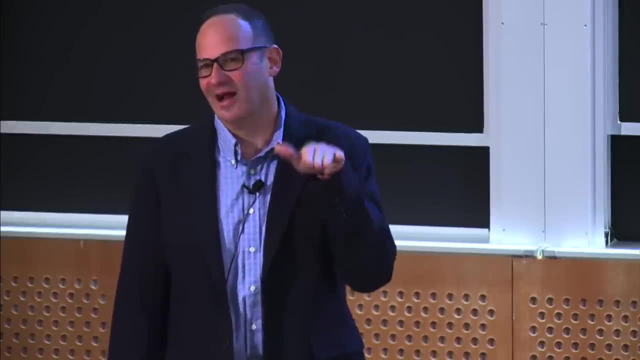 And during those eight hours they had no satellite data, no data from a ground station, So they just had no idea what they were going through And they didn't go as high as the designers thought That airplane was designed to go- super high. But they were so loaded up with fuel and bombs they couldn't practically climb all that high. So they were going at 10,000, 15,000 feet over the ocean And at those altitudes you can't really see. You may get into an embedded thunderstorm. Today's airliners: they go so high that you really are never in a position where you blunder into stuff, or almost never, because you're in the clear And you can just see the towering cumulus and not. 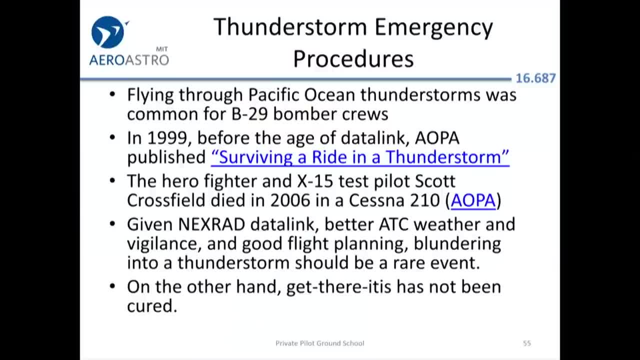 fly there. You just factor yourself around them. So I guess yeah. the final statement there is: get there. itis hasn't been cured. So as a pilot, the safest thing you can do is really fight that tendency to want to complete the mission. 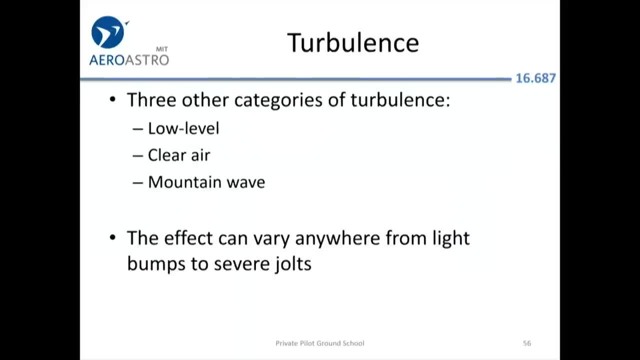 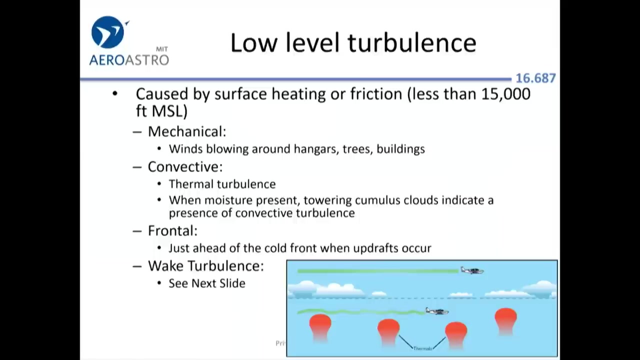 as planned and overcommit to your plan of action. All right, There are three other categories of turbulence to worry about. Probably the worst is from a plane, And that's due to terrain like mountains. This low-level turbulence from thermals is not crazy. 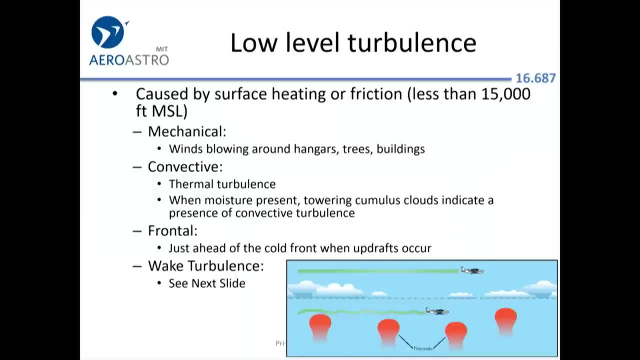 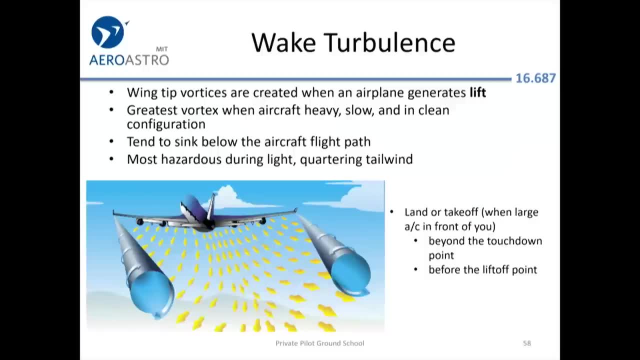 But, as I said, if you get above the clouds, that plane on top is going to be in nice smooth air. Wake turbulence, I guess, is also another thing to consider. Let's look at that If you're taking off behind an airplane. 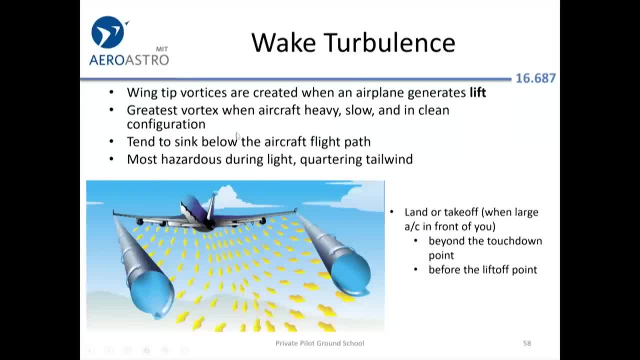 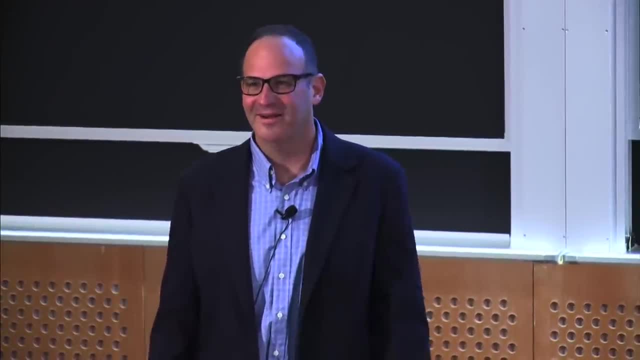 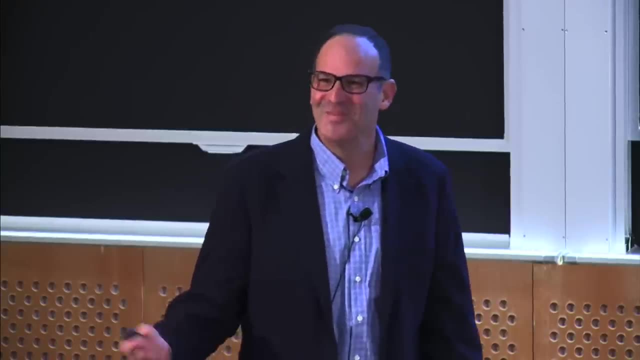 so look at that: Heavy, slow and in clean configuration. So airplanes will tend to retract their flaps and therefore be in a clean configuration shortly after takeoff, Whereas if they're landing the flaps are down, They're not generating quite as much wake turbulence. 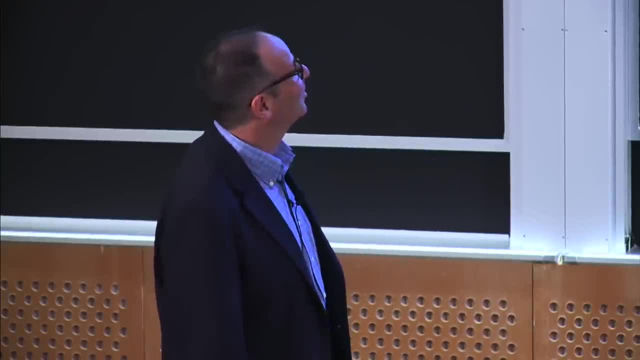 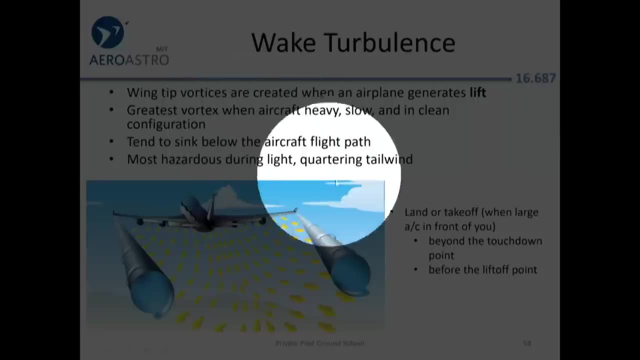 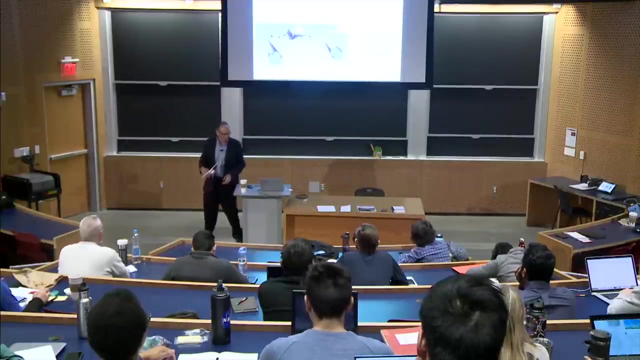 Although, still, if you land behind a Boeing in your little Cessna, you will notice that The solution here- and I think this is a test question- is you land or take off beyond the touchdown point of a large aircraft. So if the large aircraft, let's say the large aircraft, landed, 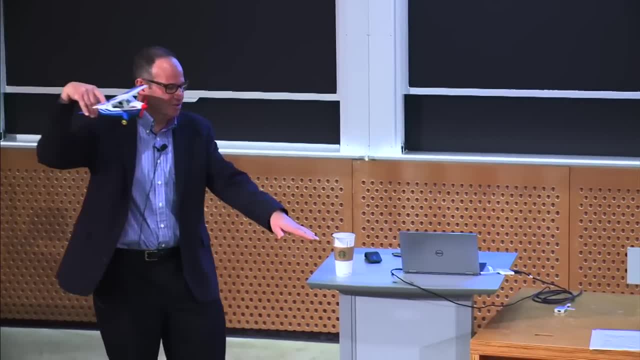 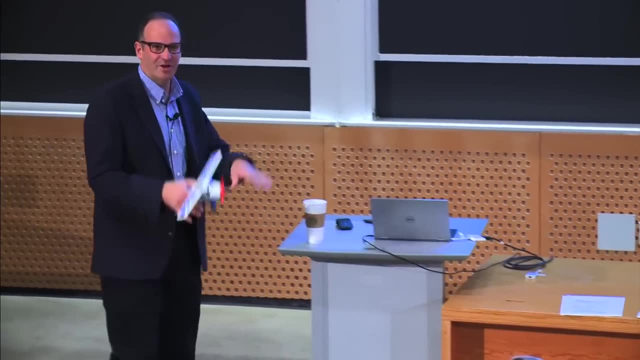 right here in front of the laptop on the runway. you just fly a little bit higher And you land maybe in the middle of the runway, And that way you can't possibly get into wake turbulence because it will have sunk below that big aircraft's flight path. 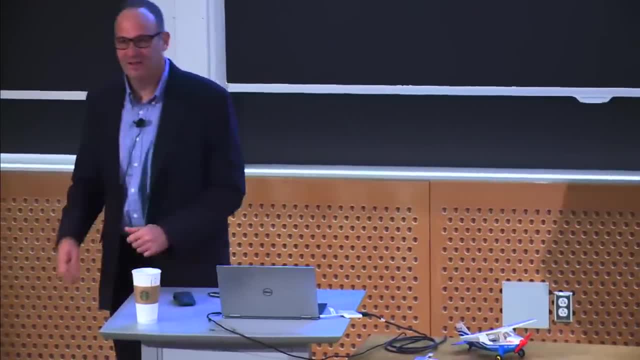 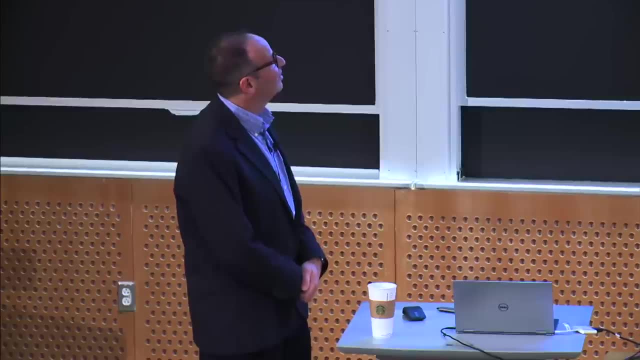 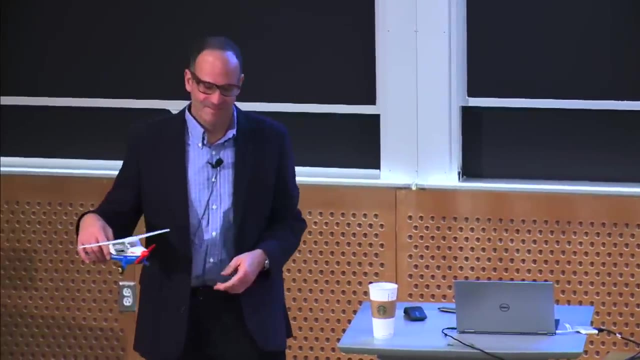 Controllers at a towered airport. they'll also separate you by the necessary number of minutes. They have a bunch of regulations about how much separation they have to have between aircraft And then similarly for liftoff point. So if the big airplane again this. 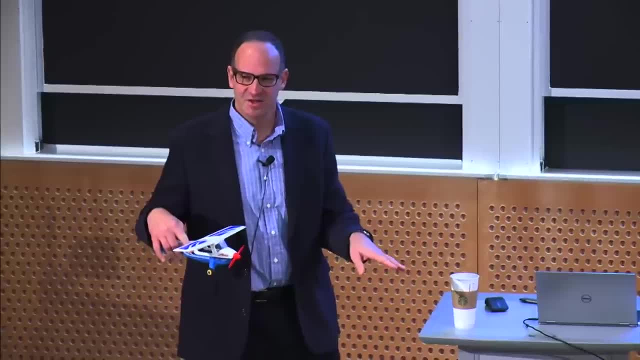 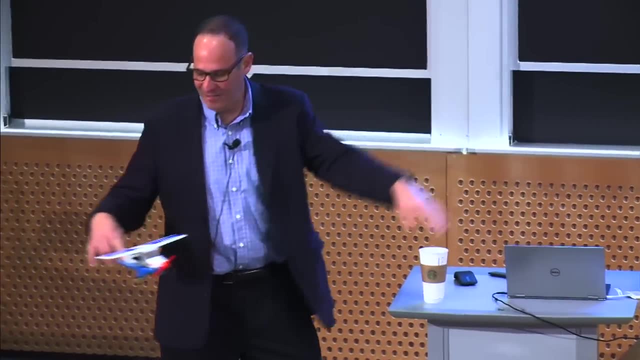 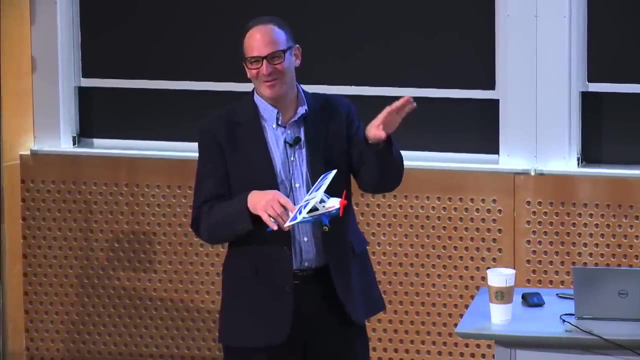 is not really that much of a practical problem because so little runway is used by light airplanes. But if the big airplane rotated and took off and started climbing here, well then you take off and start climbing earlier. Of course the climb rate of the big airplane 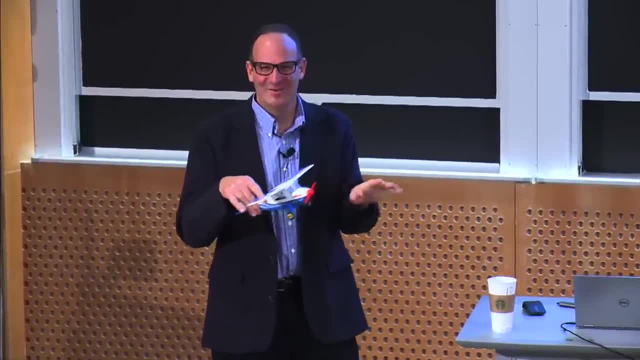 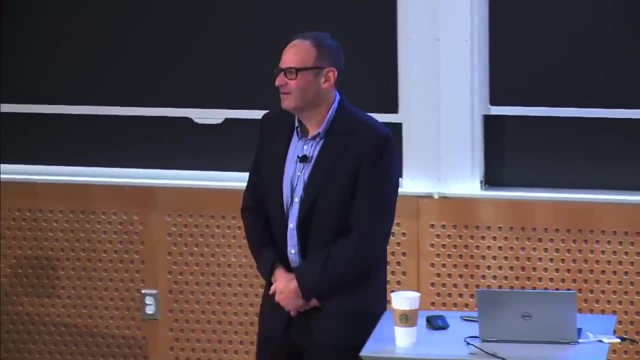 is probably a lot better than yours, So you've got to think about which way the wind is going and maybe try to turn away from it. I've only really been stuck in wake turbulence. once that I can think about, It was at Hanscom Field. 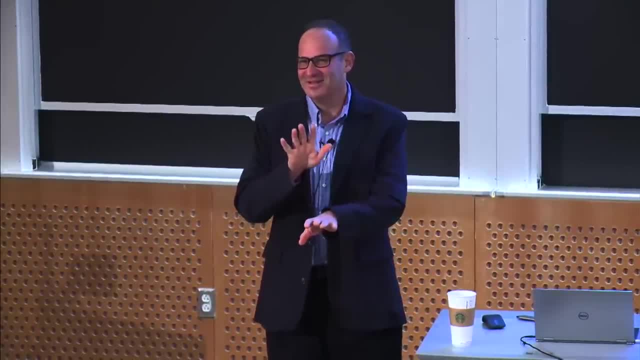 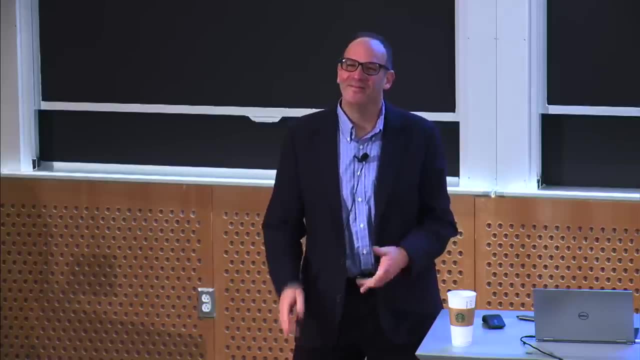 And there was a heavy helicopter that was cleared to land on the runway and then transitioned sideways And I was in the Cirrus And I think the controllers didn't really think about well how much wake turbulence can a helicopter generate. So I was trying to land. 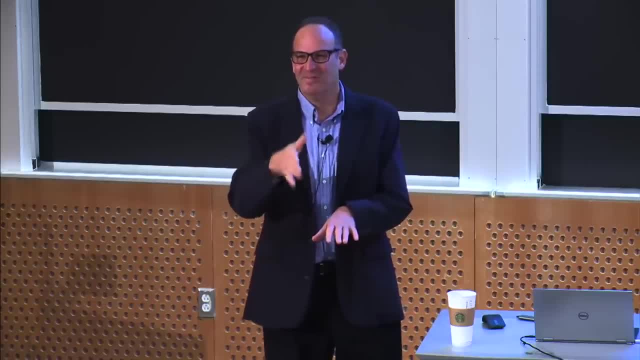 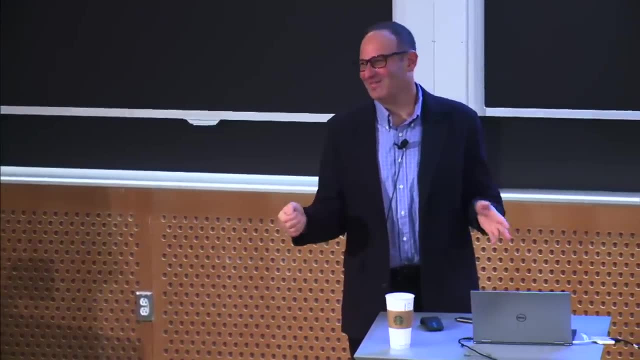 And maybe about 200 feet above the ground, there was a sharp wing dip. that I The good news is you don't have to be heroic to correct it, Because if your airplane is banked, the natural tendency is to want to take the bank out. 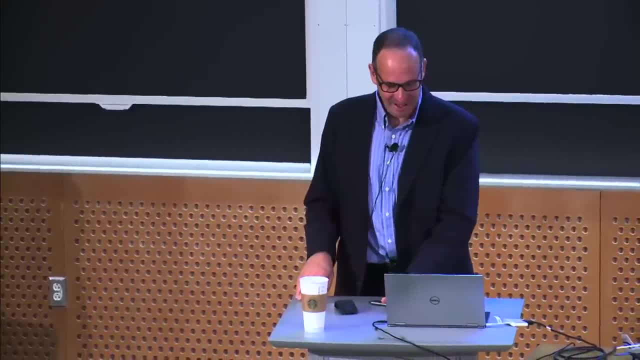 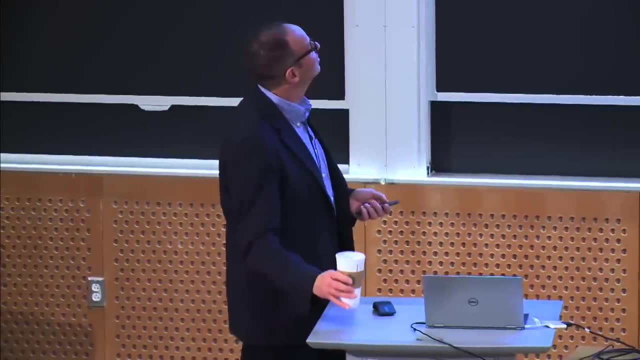 So whenever your natural tendency is to do the safe thing, that's usually not much of a problem. Oh yeah, So anyway, here's the kind of FAA question. Who wants to give an answer? Shout it out: A, B or C. 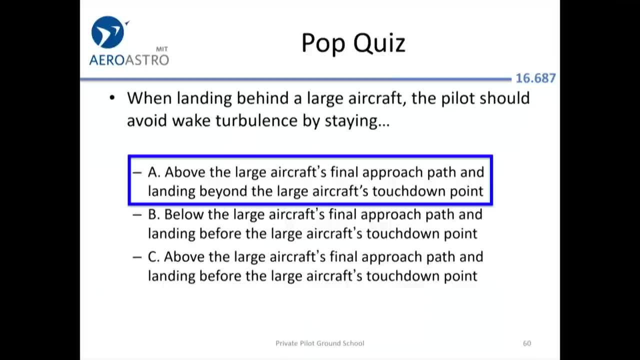 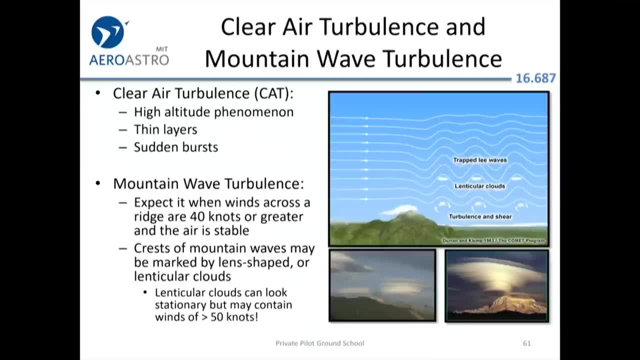 Yay, All right. So This is a practical issue, especially for anybody who wants to fly out west. You have the Sierra Mountains, You have the Rocky Mountains, And you have to be very careful when crossing these mountain ranges. If the air, if the wind aloft forecast. 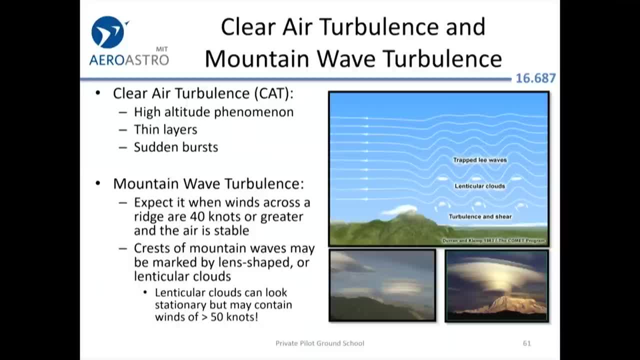 is more than about 30 knots for the time that you're planning on crossing, you can expect this kind of turbulence on the lee side or the eastern side of those mountain ranges. So But when I've crossed those mountains in light airplanes, I have usually done it first thing in the morning. 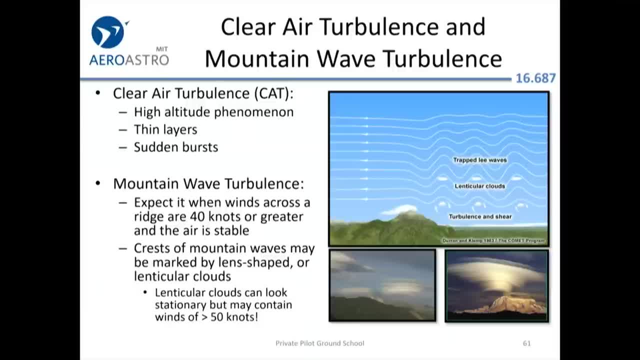 basically. So I arranged to shut down just short of the mountains the night before and then cross early in the morning when the winds are typically calm, So you can look for these lenticular clouds. But again, if you saw the winds aloft forecast. 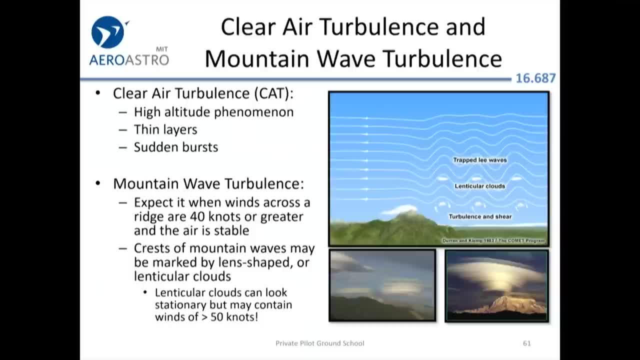 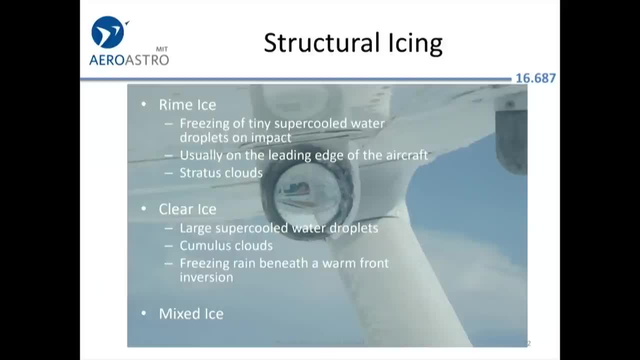 that it was going to be blowing 50 knots at 12,000 feet. you can be pretty sure that it's going to be. you know a lot, Yeah Yeah. Turbulent. All right, Structural icing. You can get rime, clear or mixed. 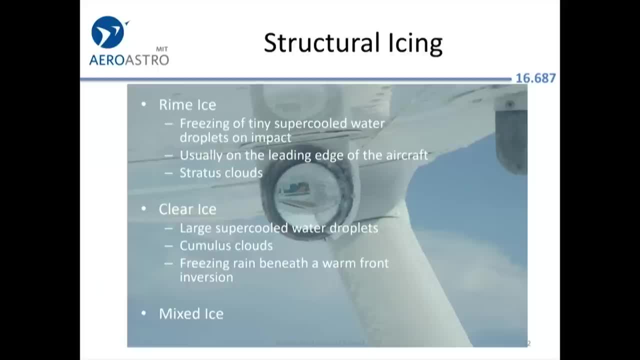 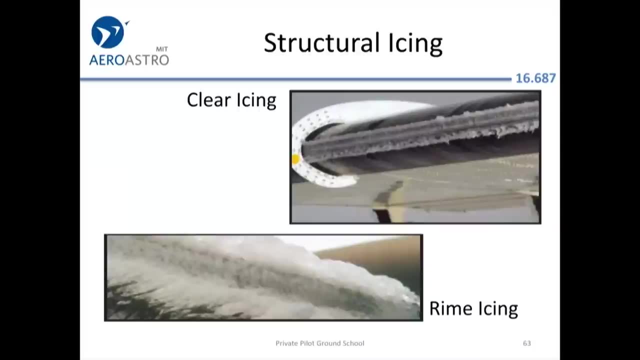 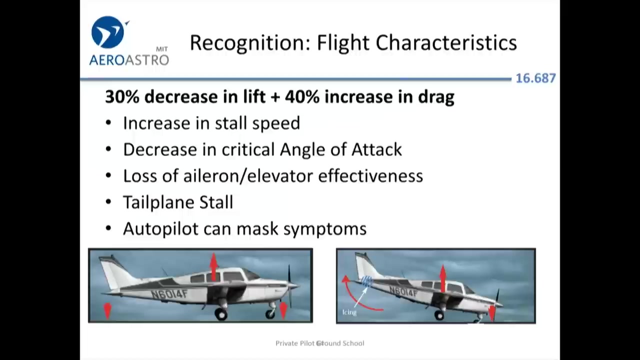 I'll just let you kind of look through the conditions that lead to this. Clear and rime- Probably rime icing is more common, But what happens? everything gets worse about your aircraft, Especially if you're on autopilot. it's kind of a challenge to recognize. 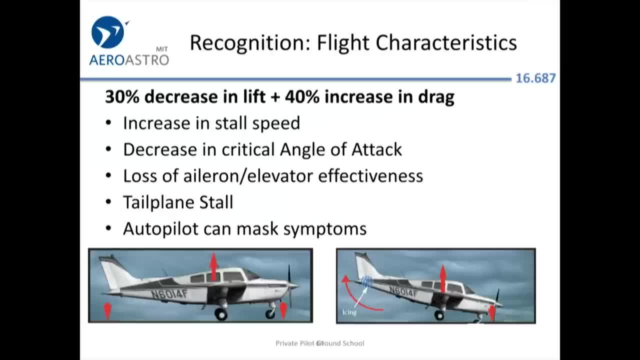 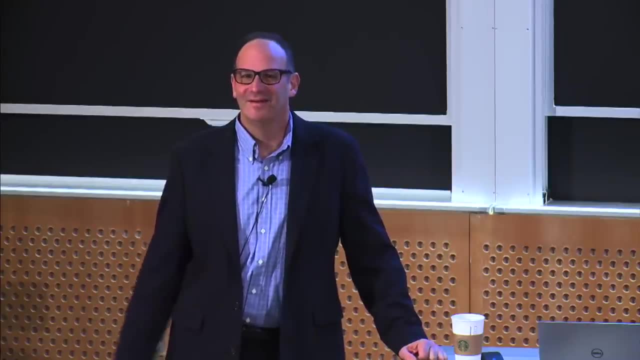 when icing is occurring. You can be in there fat, dumb and happy while the airplane gets iced up. So the worst part of it, I guess, is that you can't climb Basically when your airplane has all this performance reduction. you know? you can summarize it. 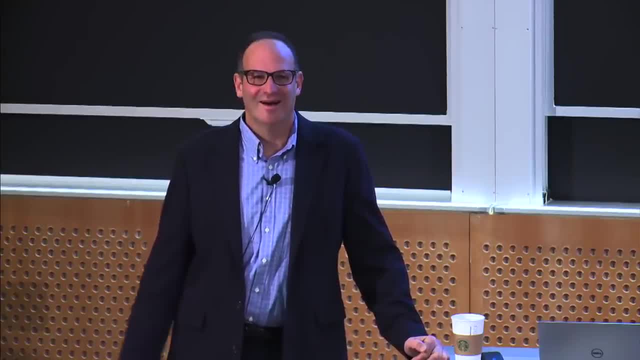 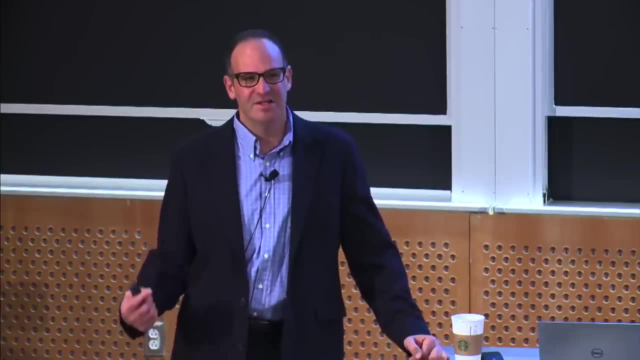 You can summarize this all: If it's only moderate icing, basically you have an aircraft that can't climb. All you can do is descend. So a good practical tip is: if you're well first of all, the good news is if you're a VFR pilot. 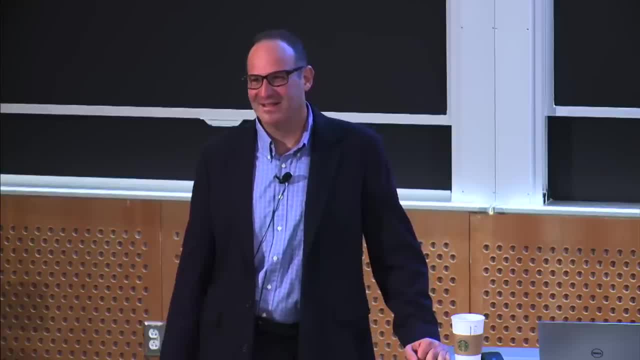 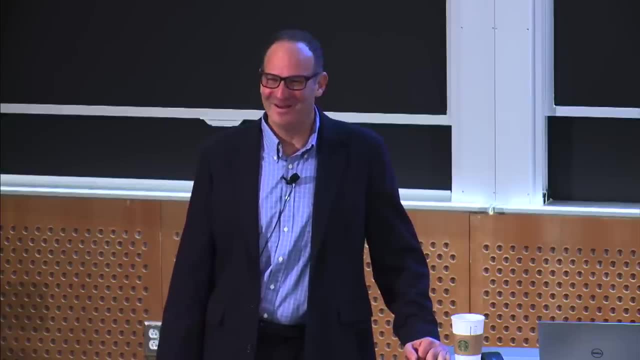 like you guys are going to become. initially, you shouldn't have to worry about icing, because it's a phenomenon that occurs when you're in a cloud, So you shouldn't be in a cloud if you're a VFR pilot to begin with. So how did you get ice? The exception might be freezing rain, if you somehow drive through freezing rain, But if you are instrument rated and you are going somewhere, I'm planning on going to New York next week in the Cirrus. So if it's cloudy, even if there's no icing forecast. 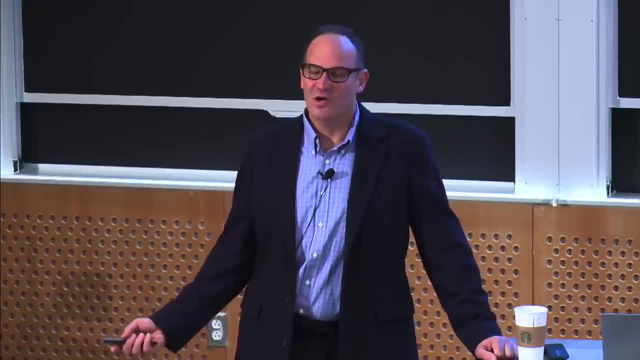 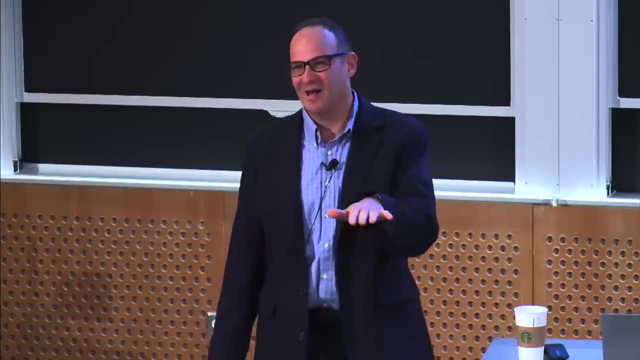 I know that there's a risk of getting ice on the wings. So in the wintertime I just say: well, look, I'm not going to go unless it's above freezing on the surface, Because if I get iced up, then inadvertently 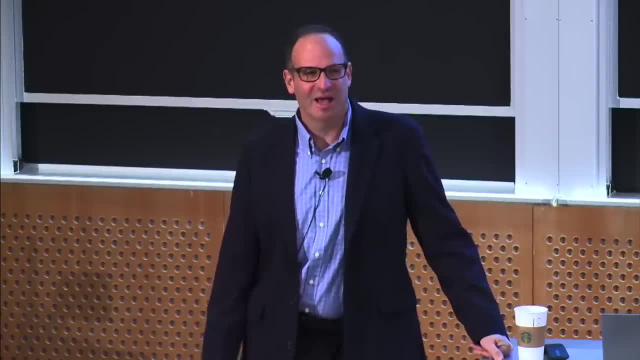 I need an escape route, And if it's going to be above freezing at, say, 3,000 feet, well, that's fine. I know that I probably won't be able to climb if I get moderate icing, but I will be able to descend. Even a brick can descend. So descend down to 3,000 feet and all the ice will melt off. That would be great, But if it's below freezing on the surface, then it's basically a no-go. I've definitely had icing a few times. 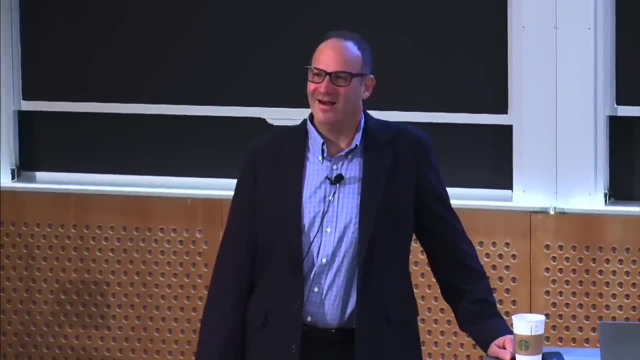 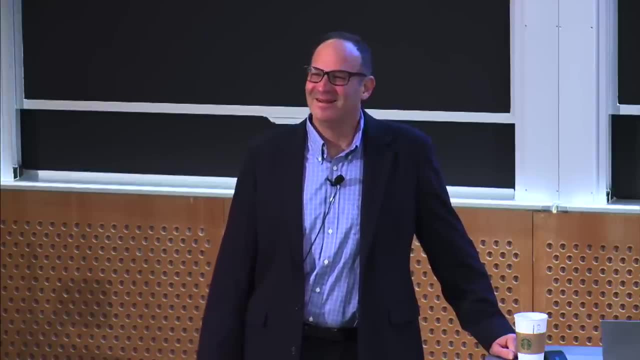 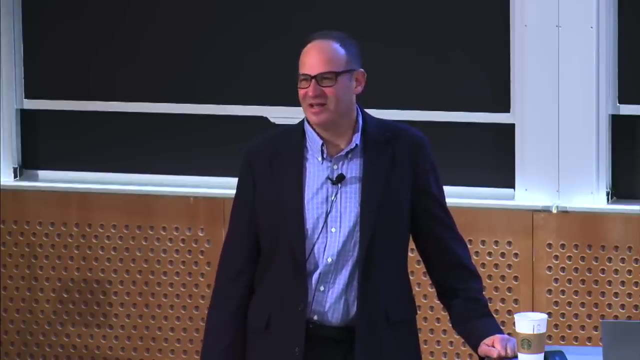 and it's pretty scary. I was out on a day with a instrument student and it seemed like a perfect day to go practice instrument flying. There was no turbulence, There was just clouds everywhere, about 800 feet of ceiling, So you could be in the clouds. do real approaches? 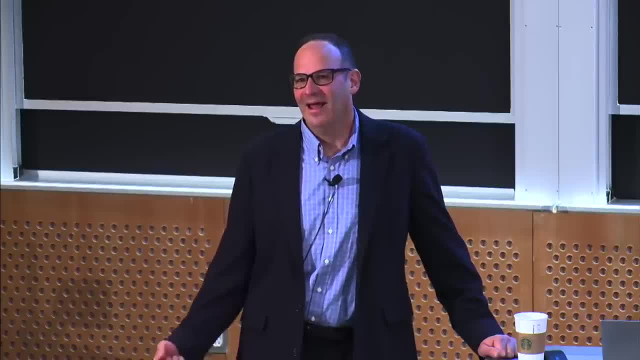 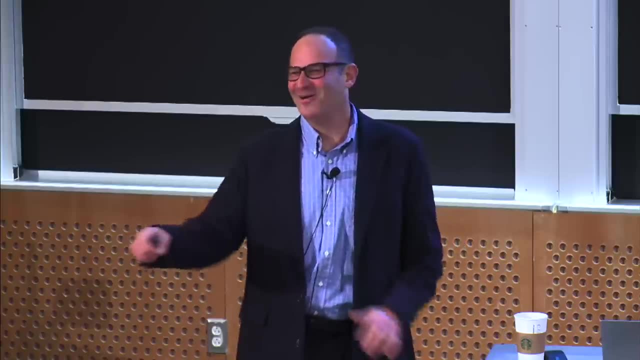 get experience with actual IMC. And halfway through the flight I started criticizing this guy for using way too much power. Like the power settings were all off, Like what are you doing wrong? And then I kind of looked out on the wings. 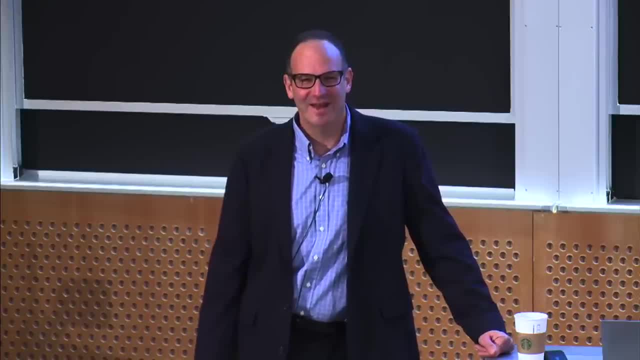 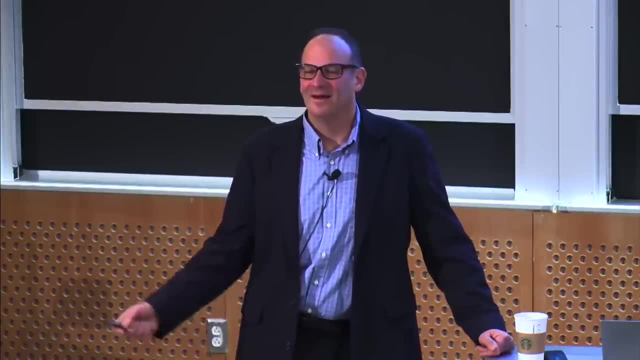 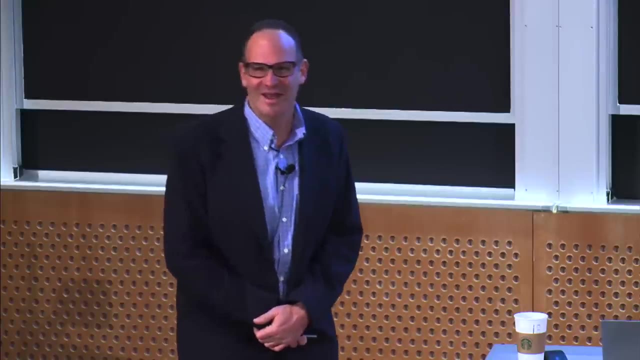 and I saw they were all frosted, So we descended. We managed to complete an ILS approach into Lawrence and pulled the airplane into a warm hangar and got it warmed up. So actually, as we were flying, the FAA issued an airmet for icing, but the controllers never. 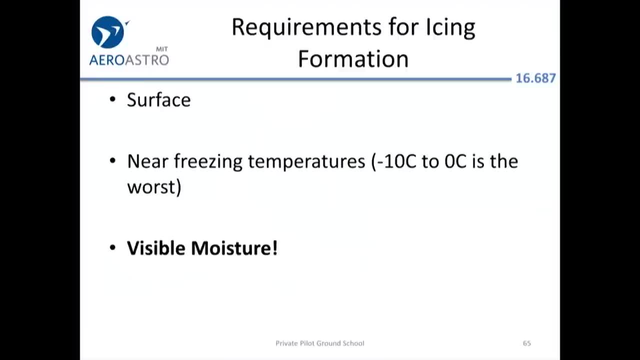 told us about it. All right. Requirements for icing formation: Near freezing temperatures- minus 10 to 0, is the worst. You have to have a surface on which the ice can form and you have to be invisible moisture, basically. 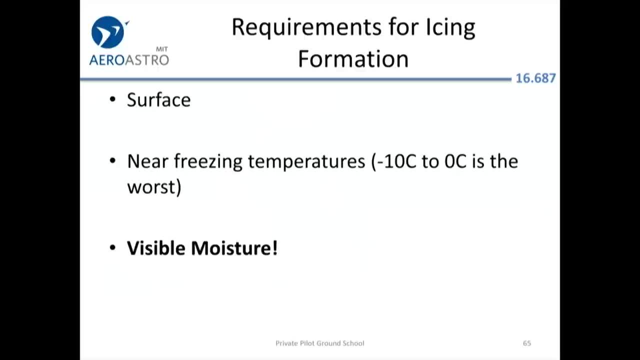 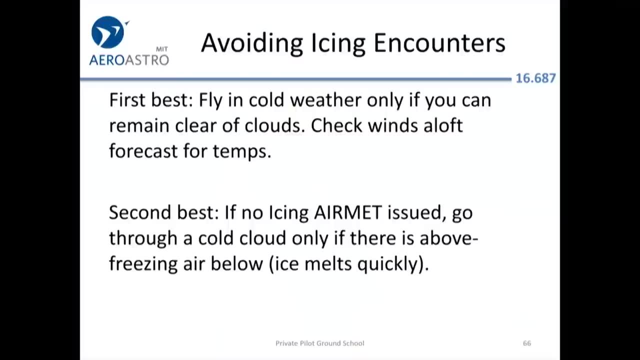 So, again, if you're flying in the clear with your VFR pilot certificate, icing should not be a factor for you. Yeah, So, as I said below, go through a cold cloud only if you have an escape route of warm air below. 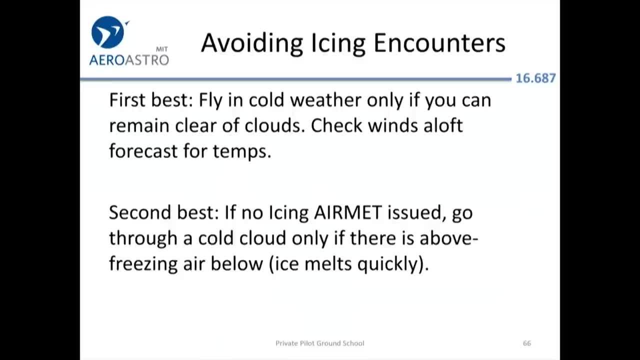 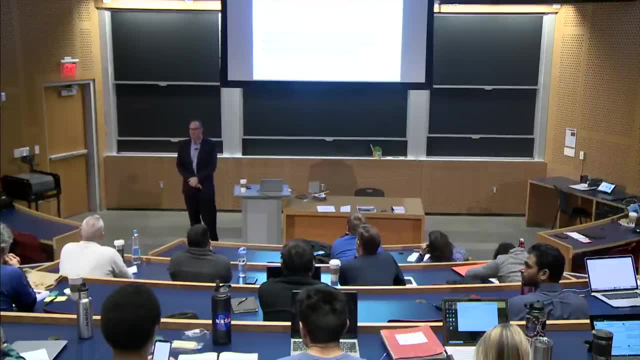 Is that also true for the engine, though? as far as getting the icing, It's evident. Do they have an insurer here in the UK? Yeah, So the question is, what about icing in the engine So you can get carb ice that we talked about? You can get carb ice when it's a You know 50 degrees outside, as long as it's humid. So it's slightly unrelated. The main problem with engines is that you can get ice in the induction, So if the intake for the engine where it's trying to breathe, 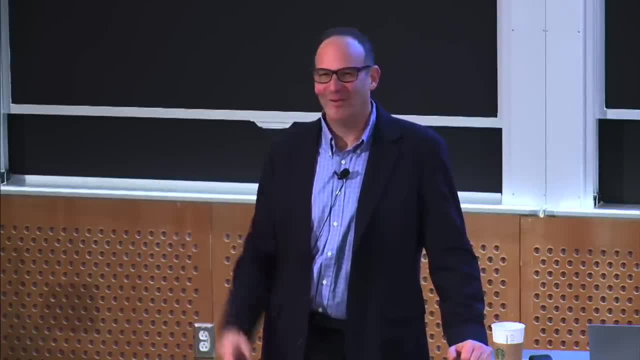 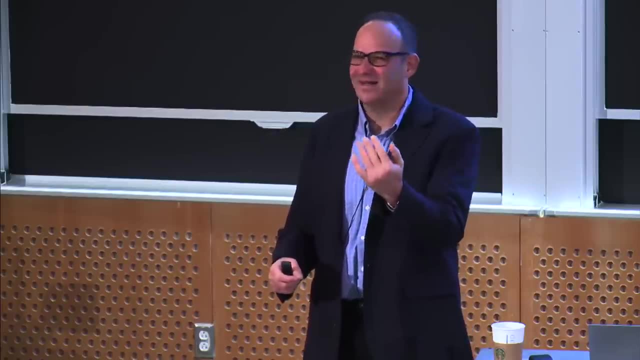 gets iced over. then there's an alternate air. Again, they're kind of relying on the hero pilot Some airplanes. actually it'll just open automatically. The vacuum of trying to suck the air through the intake that's not working will cause some backup doors. They'll have a door to open And a lot of most IFR-certified aircraft have an alternate air lever that you can pull and have air pulled from somewhere inside. that's a little more protected inside the airframe. Does that answer your question? 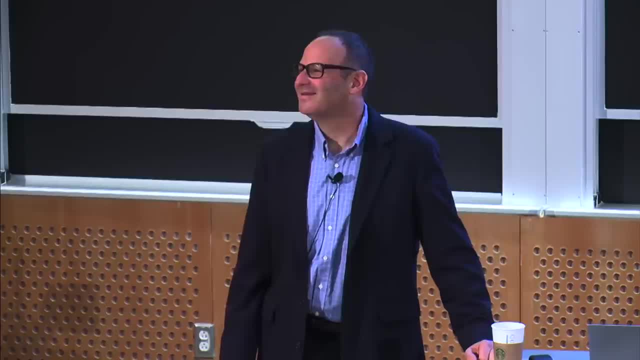 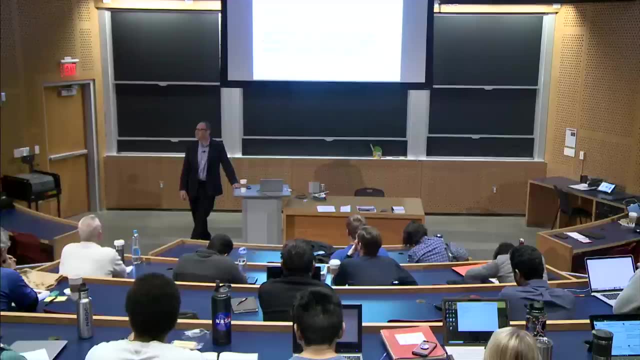 Yeah. So I guess you're saying as long as the heat's working. you're saying clear air, As long as which heat? Well, I guess the engine's running. so I guess as long as you're Yeah, you're not going to get carb icing and airframe. 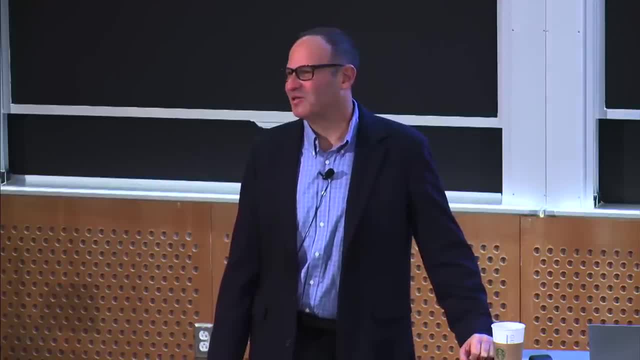 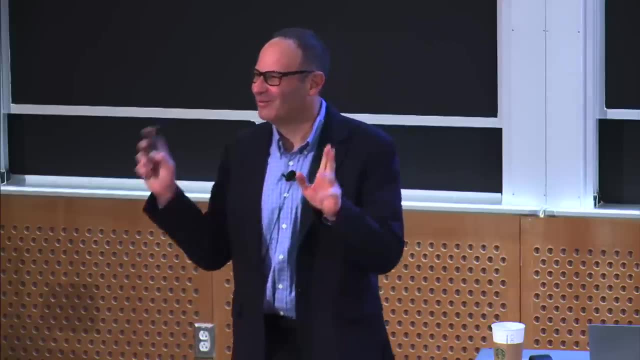 icing at the same time, probably, I think at that point it's probably too cold, I'm not sure. Well, the other issue is: you're probably not going to fly a carbureted airplane into the clouds, because the real IFR airplanes that people 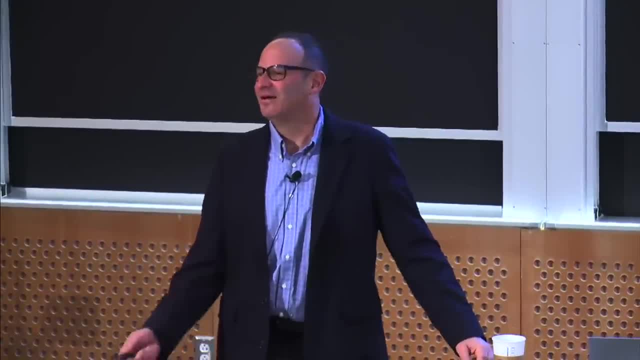 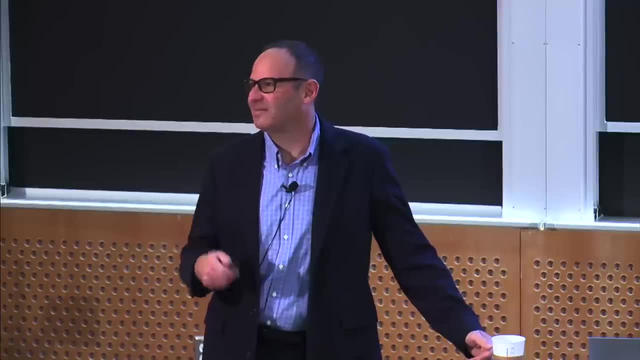 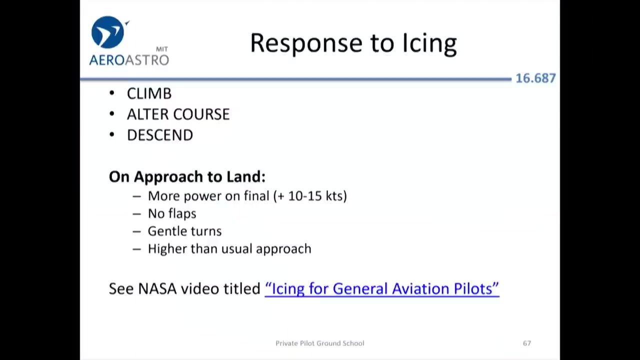 use to travel, like Cirrus' and Bonanza's and stuff in challenging conditions. those are almost all fuel injected, But you do have to worry about induction icing, like I said. Yeah, OK, You can. Icing layers are usually pretty thin. 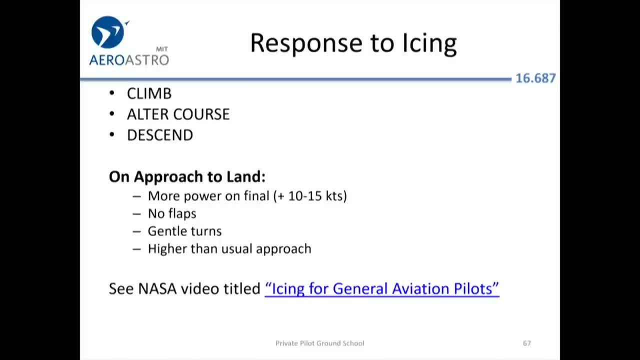 So if you're in a jet, you just add power and climb up another few thousand feet and you're out of it Again. one of the effects of icing is to dramatically reduce your climb performance. So this best approach of climbing out of it- 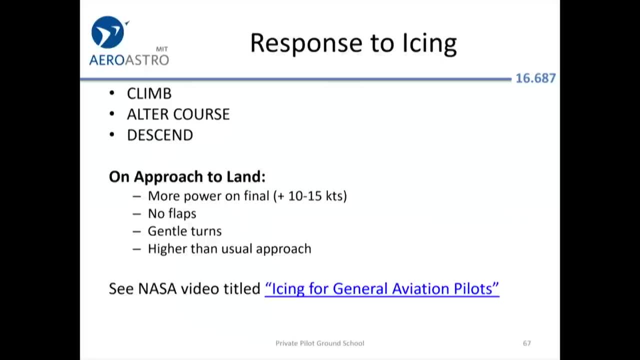 is not always available. You will end up using more power on the final approach And you'll add speed as well, because the stall speed may have gone up And you can't really be sure, since it hasn't been quantified and tested. 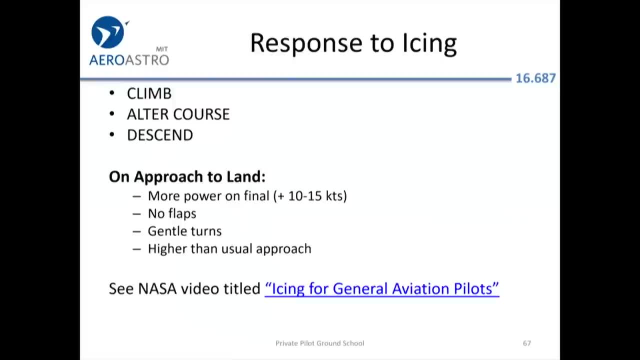 You probably won't use flaps And you'll not make severe turns, So there's a good NASA video that I encourage you to watch, especially as you- Yeah, I work on higher performance aircraft and IFR. NASA has this great video about icing. 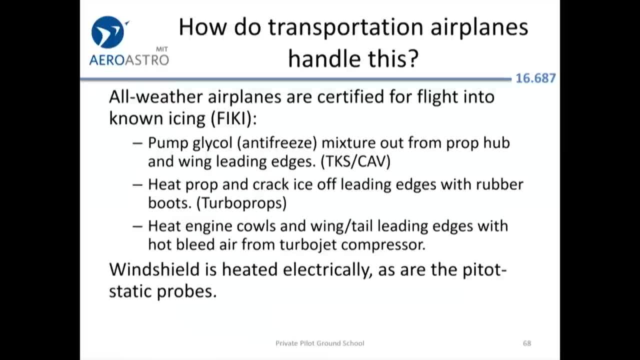 OK, How do the transportation class airplanes handle this? One approach is to push antifreeze out onto the wings. That used to be called TKS, Now it's called CAV. It's just a brand name. So if you go to a flight school and you 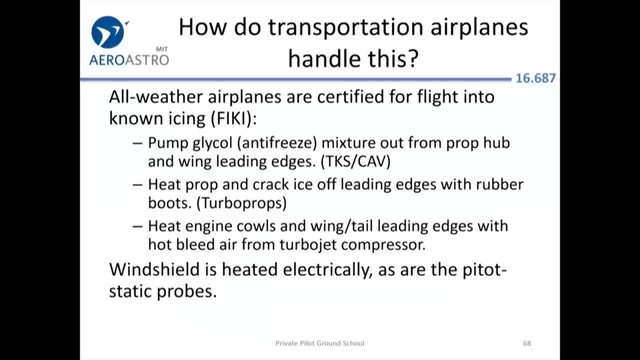 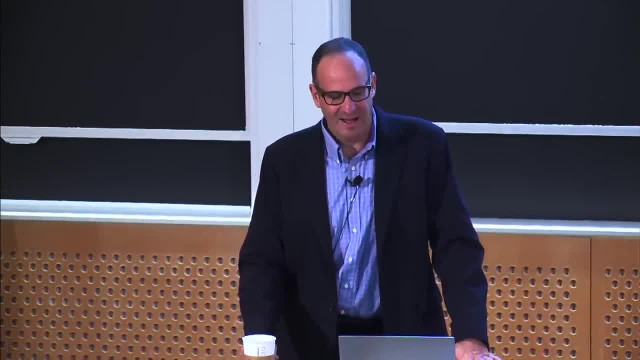 see a modern Cirrus like the SR-22s. the leading edges of the wings will be metal And they'll have little tiny holes in them And that's for this antifreeze to come out, If you have a very light jet or a turboprop. you may have rubber boots on the wings and on the tail surfaces And those inflate to crack the ice off. The jets are really the ultimate. The bigger jets all have bleed air. Remember, the jets are compressing air so much that it becomes really hot even before it's burned. 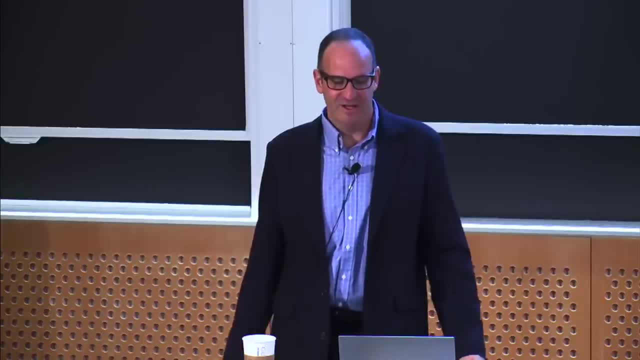 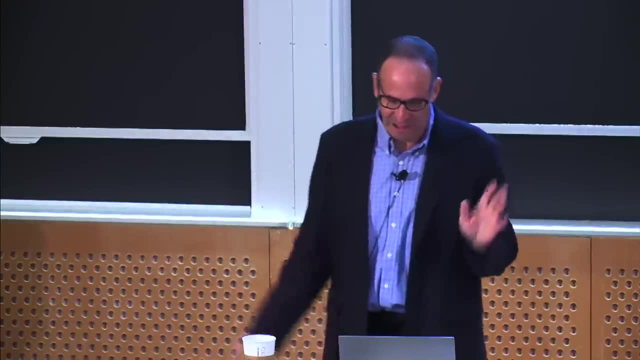 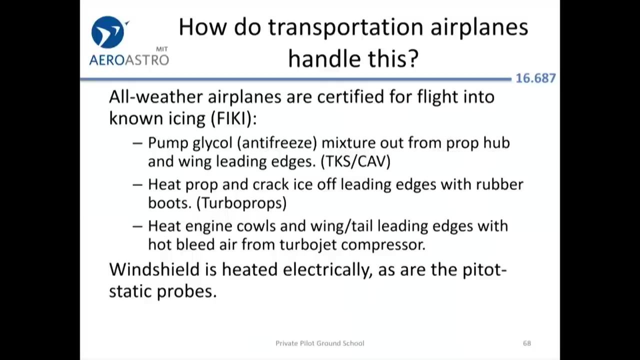 So you pull the bleed air off- It's a compressor- And you run it out into the leading edges of the wings And that just melts the ice off The transport aircraft. they also heat the windshields, So you'll be able to see when you do. 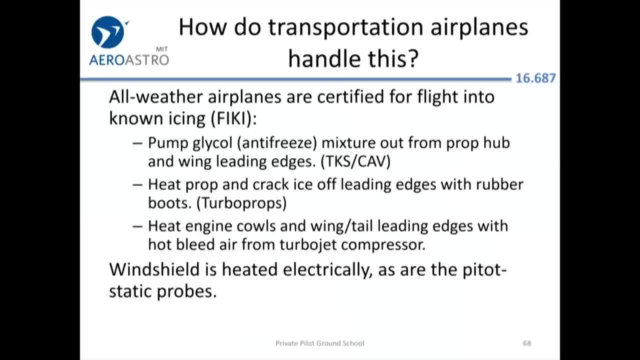 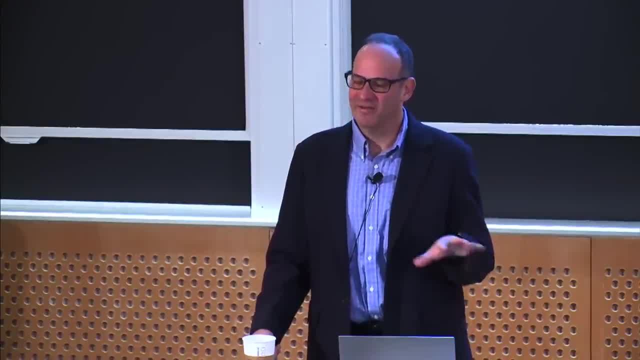 If it's not above freezing at the airport, you'll have a clear windshield so you can see the runway. Even in very basic airplanes like a Cirrus- if they're IFR certified- the pitot tube is going to be heated. 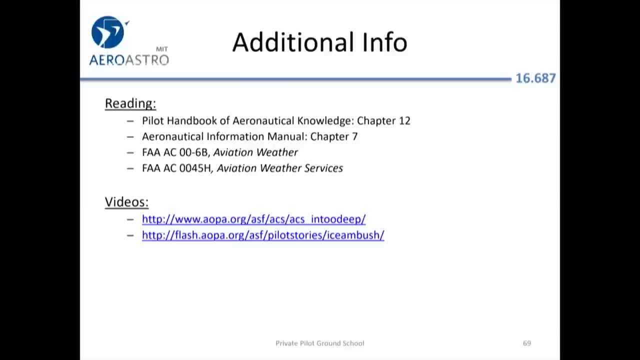 That will be pitot heat. OK, You can learn a whole bunch more about this. I think everything you know to pass the test is pretty much in the pilot's handbook of aeronautical knowledge. There's a little bit in the AIM. 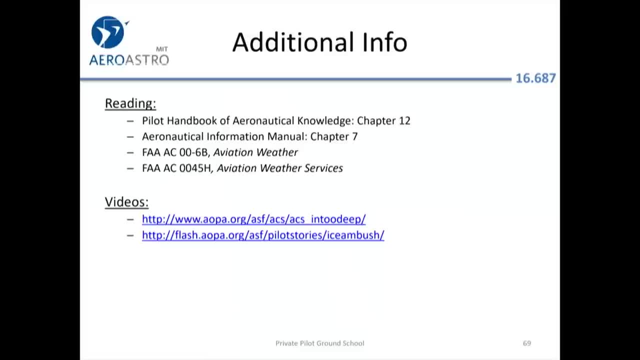 If you want to dig deeper and understand more of it, then I would encourage you to look at these FAA weather publications. One is about weather theory And one is about information that you can get from various sources. There's also these videos that I would encourage you to look at. 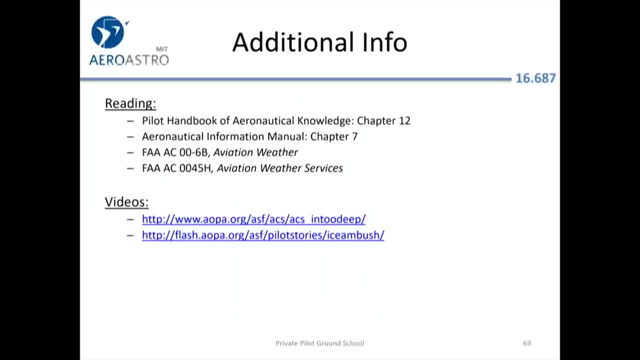 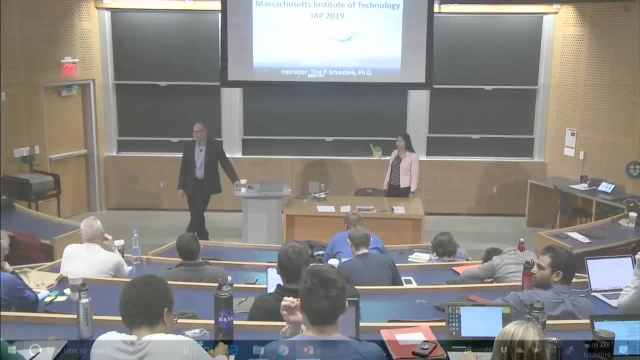 One of them is called Ambushed by Ice and Into Deep. I think these particular links don't write those down because I fixed them last night But the Dropbox didn't update yet. Do they have real-time weather data? So the question is in your basic trainer airplane. 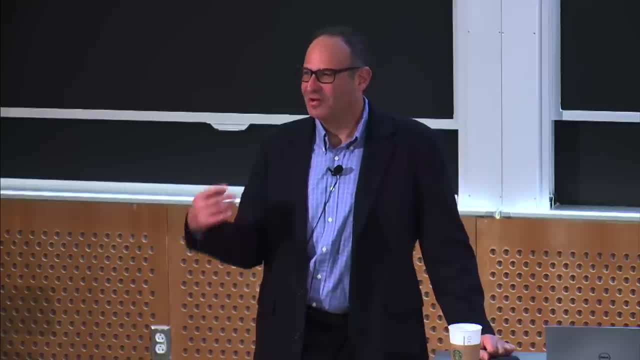 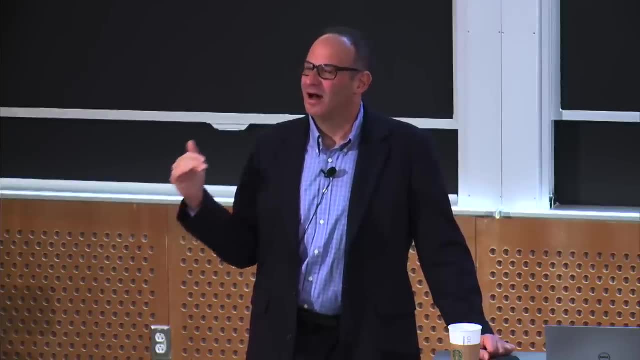 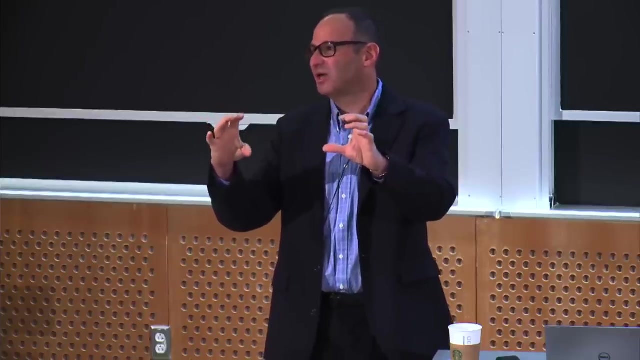 do they have real-time weather data? So I'll just talk about East Coast. Aero Club is sort of a typical higher-end flight school. About maybe 10 years ago almost all the aircraft had a Garmin IFR-certified GPS put in a Garmin 430.. So at that point you had a really good GPS, But they did not have XM weather pulling data from satellites, which we'll talk about in a little bit, Because it's like a $500 a year subscription And it's a $10,000 box. 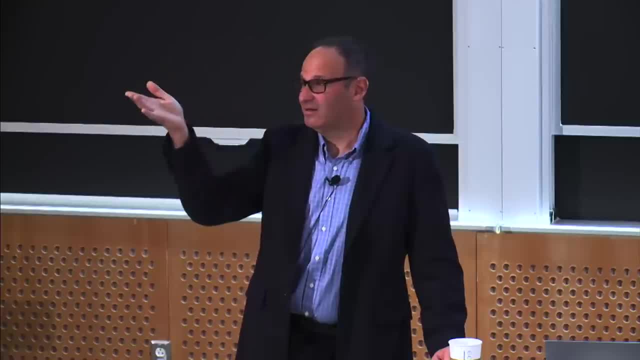 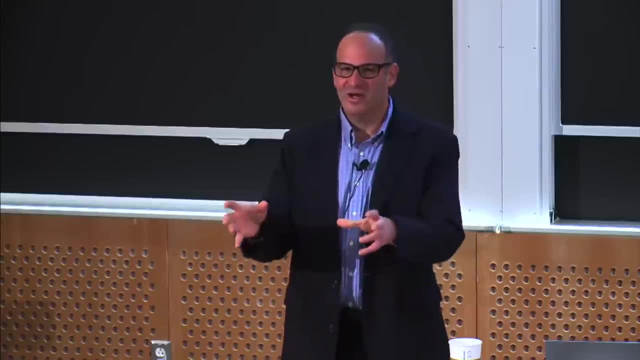 So people didn't want to do it. With ADS-B, the FAA is now providing some of the same data that XM was providing for free. as long as you have an ADS-B in transponder And the East Coast Aero, well, everybody. 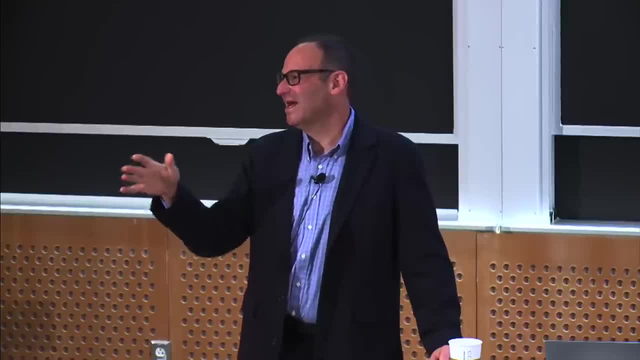 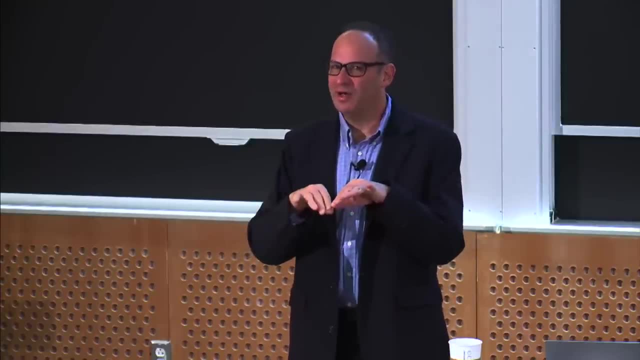 has to upgrade to ADS-B by 2020.. Not everybody has to have ADS-B in, But I think East Coast Aero Club is probably fairly typical of the better flight schools, Or they're gradually putting in ADS-B in and out transponders. 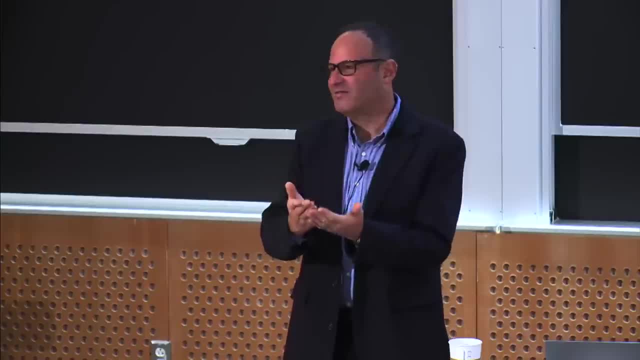 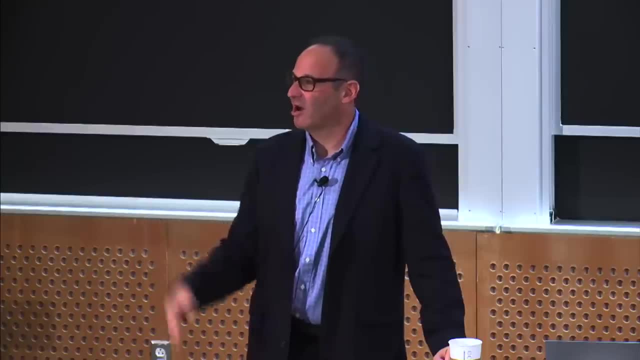 in all their aircraft. It won't display in the cockpit. You'll have to have your phone or your iPad or something. But you'll be able to see a NEXRAD radar picture. You'll be able to get METARs and TAFs. 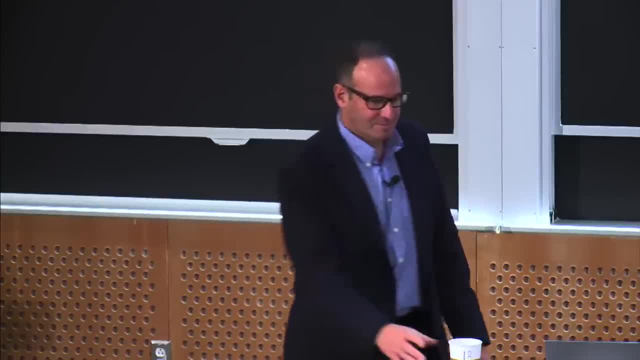 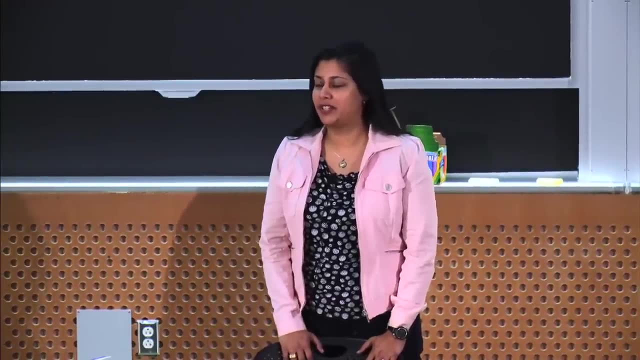 You'll get all of that, So I think. But if you don't want to rely on someone else- this is MIT- you can actually get that data yourself. So when we talk about weather data today, we're going to also talk about how you can. 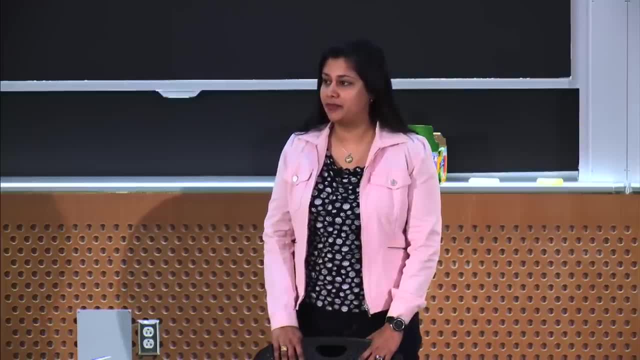 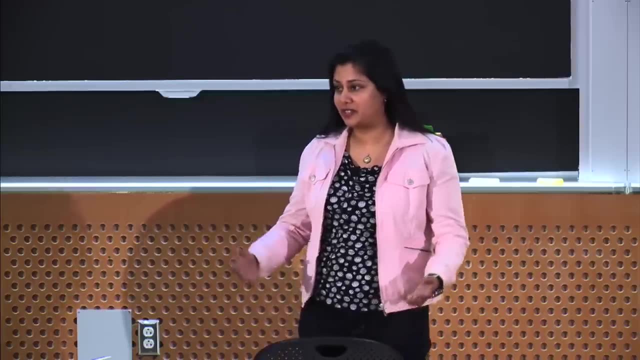 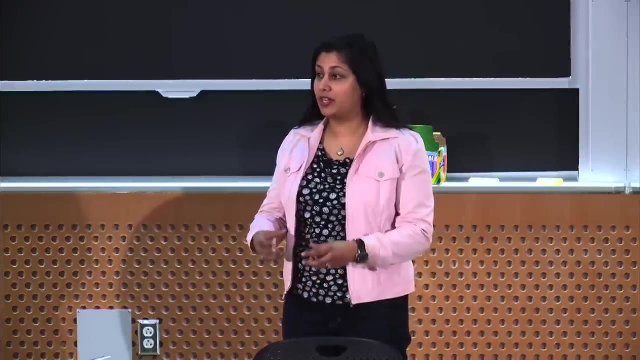 do it yourself: build your own Stratix ADS-B receiver- And I've actually done this. It was really fun to do. It's very easy actually. It's basically based on a Raspberry Pi with a couple antennas with a little cooling fan. 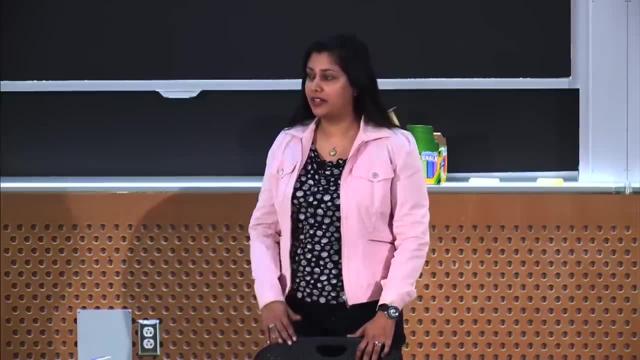 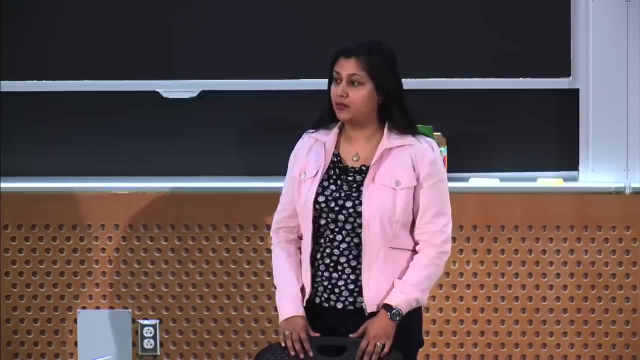 You can build a little box that can receive that weather data And actually the software is open source And it can sync with your other tools. So I have it synced with my ForeFlight app, So when I'm flying I plug that in. 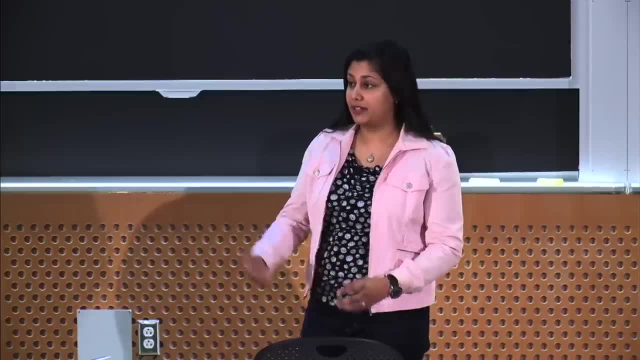 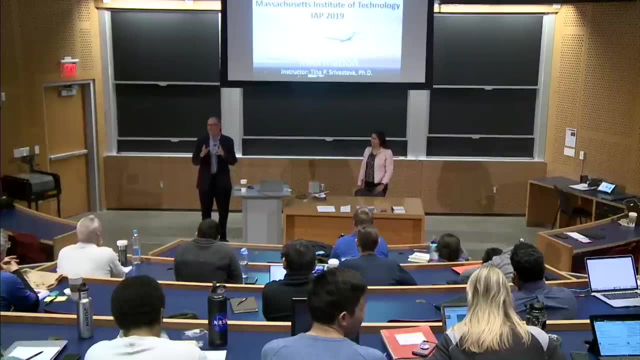 I bring a backup battery for it And it gives me weather data and some other traffic data, And we'll be talking about that in a couple hours. Yeah, I should have noticed, as Tina said, a lot of flight school customers for the last five years. 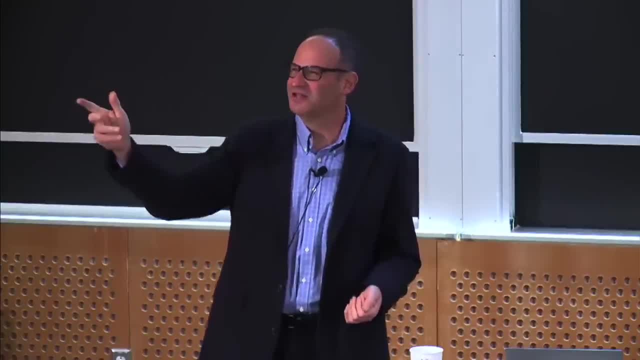 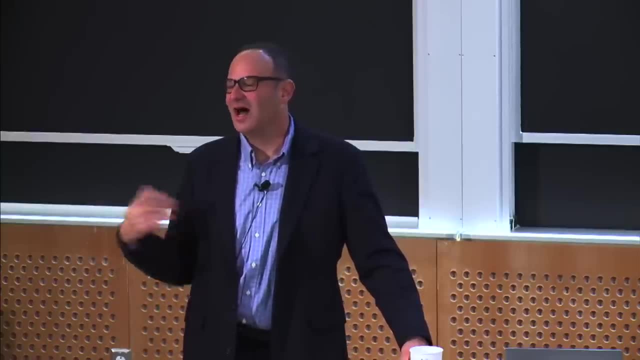 would bring little battery-powered boxes and stick them to the windshield of whatever they're flying And they would get a whole bunch of more modern services. I personally don't love that. When I started out In my flying career, I had my big flight bag. 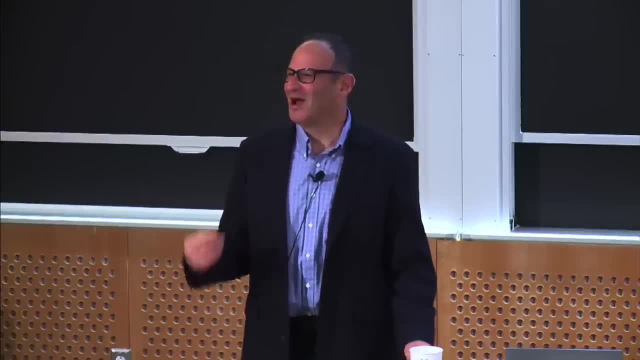 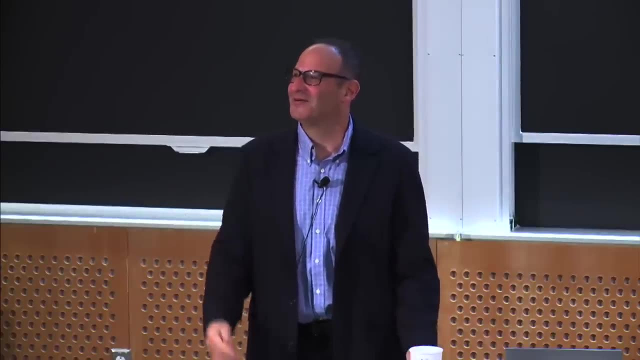 with all the stuff I was going to bring into the airplane And now I have the philosophy that I don't want to bring anything into the Cirrus other than a pencil. I want everything that I need to be in the panel. But yeah, I definitely think in the older airplanes. 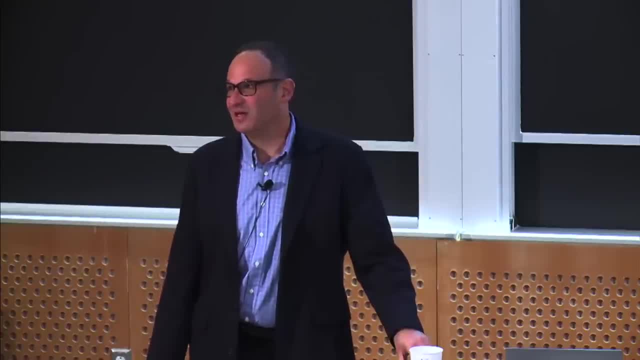 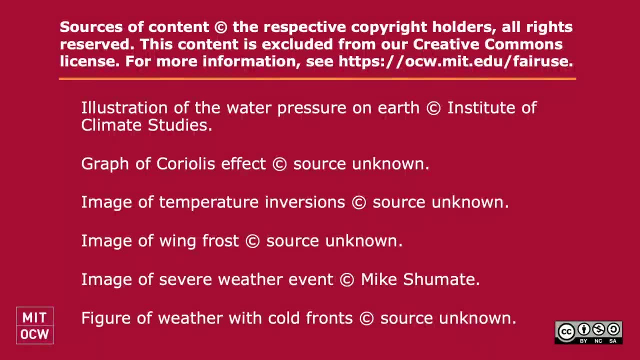 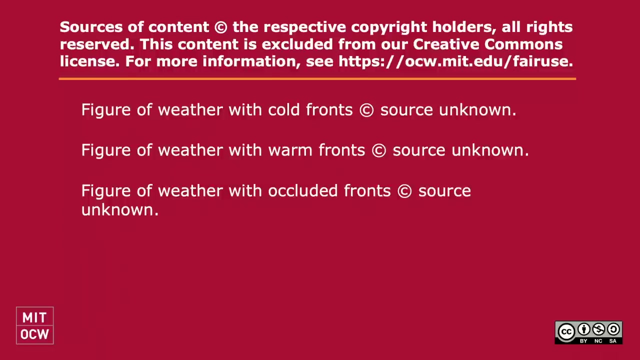 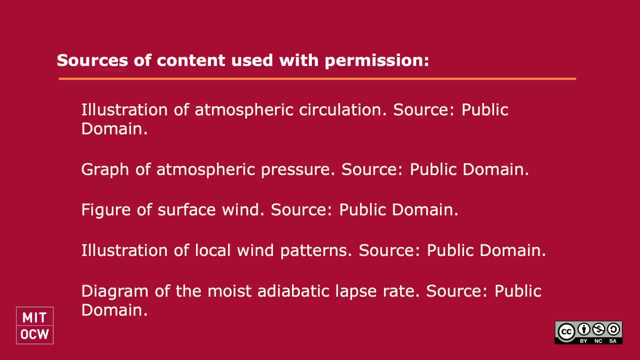 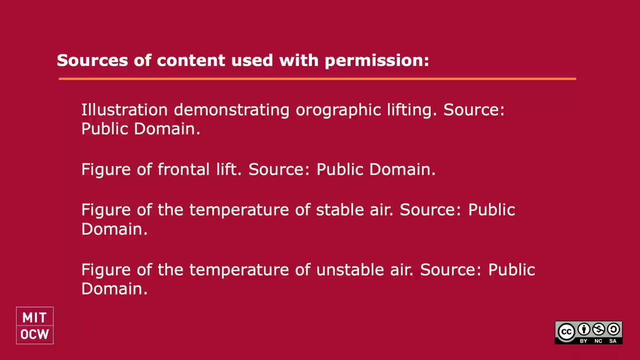 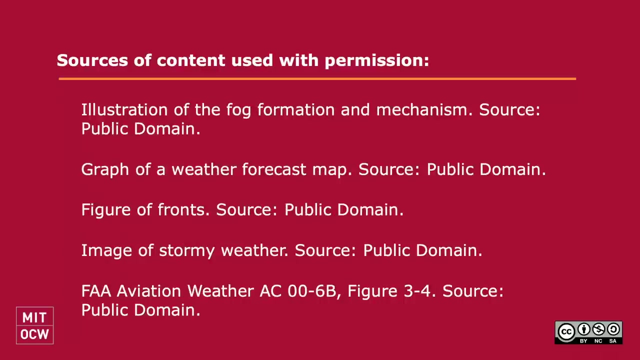 it's become conventional for people to bring some sort of ADS-B receiver and get that data. Yeah, you.